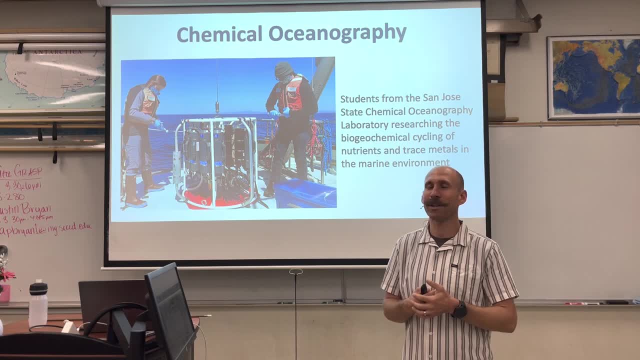 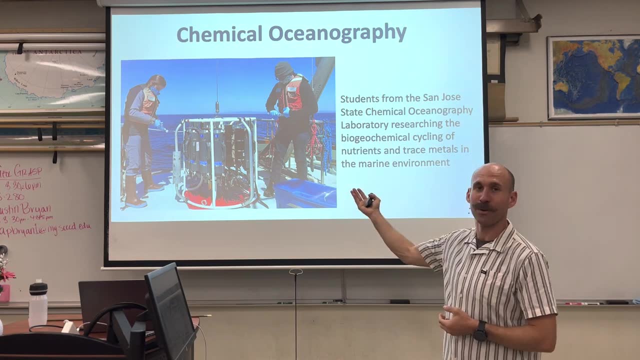 And if you like what there is today, please contact me, Let me know. We will get you connected. There's great resources and great institutions out there where you can do groundbreaking science, just like this. Okay, Whole laundry list of what we're getting into today. 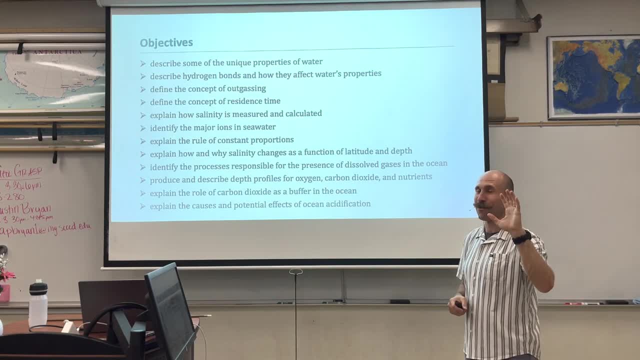 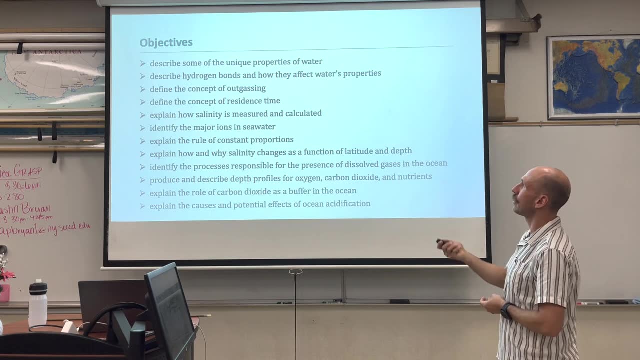 We will look at the unique properties of water. This is one of the biggest, Most important, most exciting parts of our lecture will describe hydrogen bonds, how they affect water's properties, to find the concept of outgassing and tie that into the origin of Earth's water. 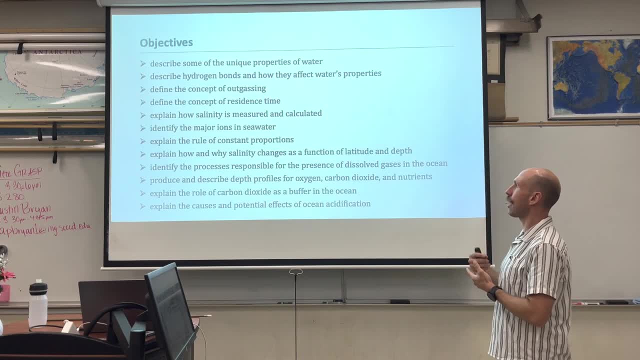 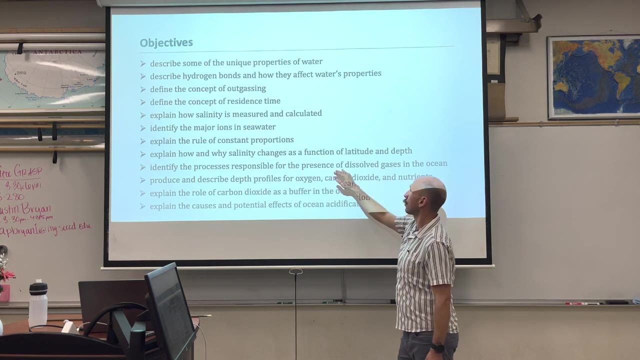 We'll look at residence time. discuss salinity, how it's measured, how it's calculated, identify the six major ions in seawater. talking about the rule of constant proportions, We will dive into why salinity changes with. these are the big two. 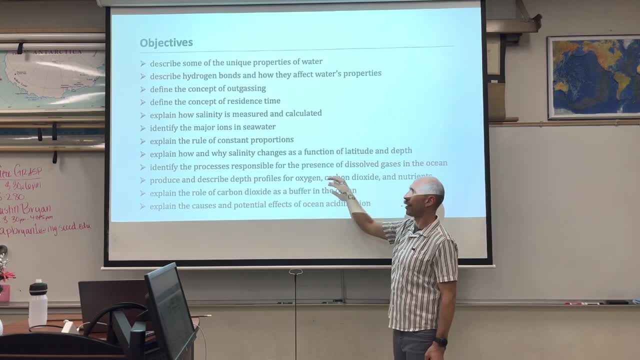 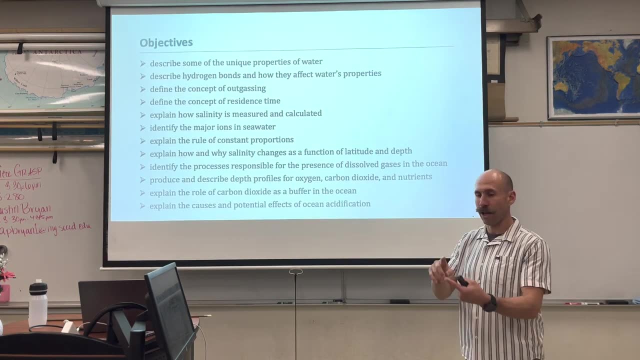 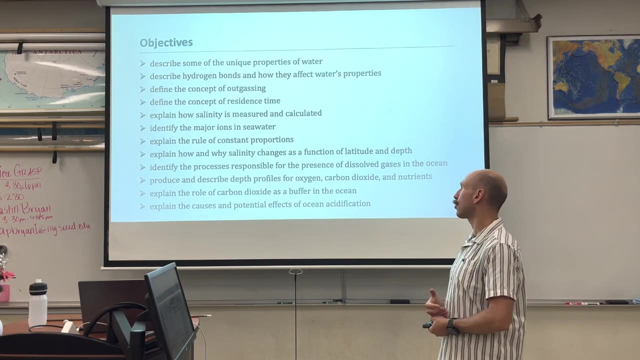 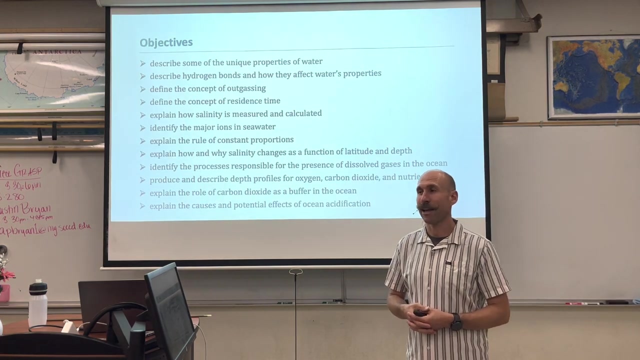 Latitude and depth, will identify the processes responsible for dissolved gases, the importance of those dull dissolved gases, including oxygen, carbon and nitrogen, And then we'll look at carbon dioxide as a buffer in the ocean and then round out our discussion on ocean acidification: what it is and why it is important. 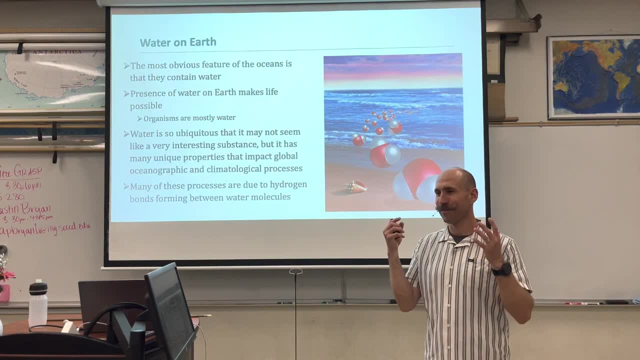 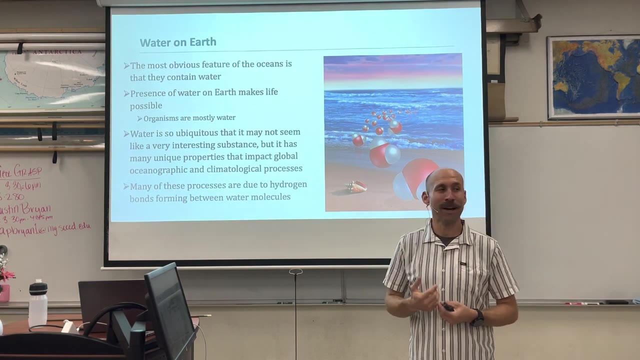 Okay, So water. It's the most obvious feature on earth. This is the blue planet, as observed from outer space. Water covers 70% of our globe And water makes life possible. without water, As far as we know, from anything that we have ever seen, discovered, understood, there's no life without water. 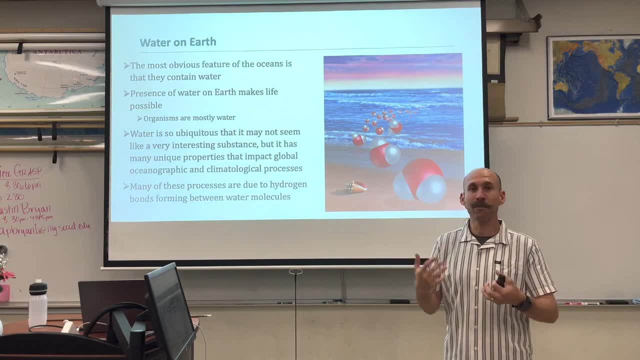 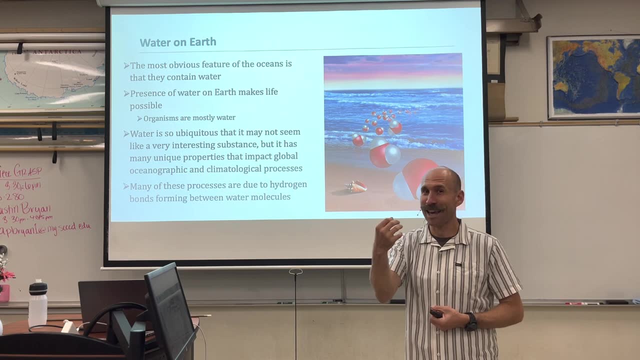 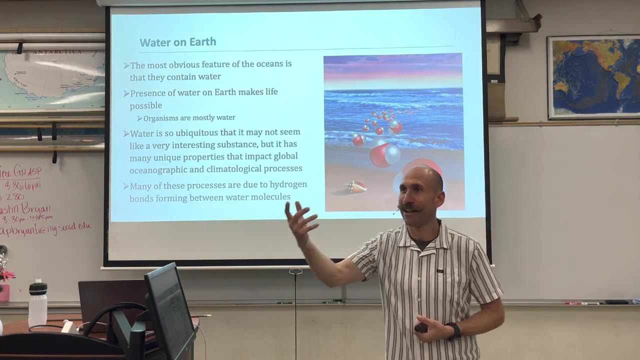 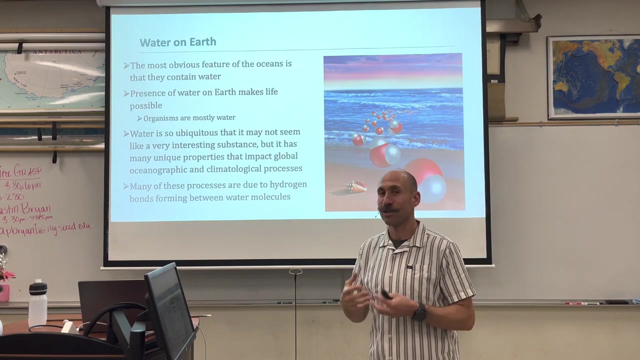 And so thank you water For being here. It's ubiquitous, It's easy to be taken for granted, But no Water has unique, special properties in its chemistry that allow the oceans to be what they are, that influences atmospheric and biological systems. and then water is so cool all the way down to 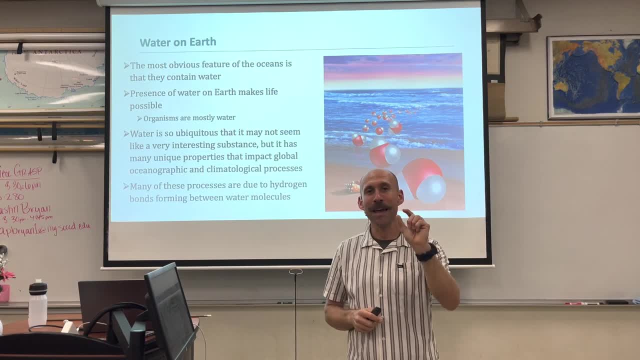 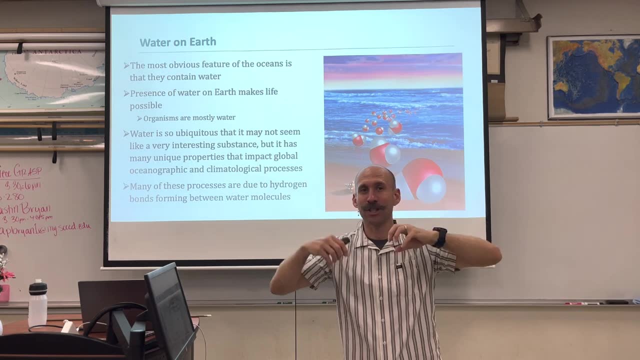 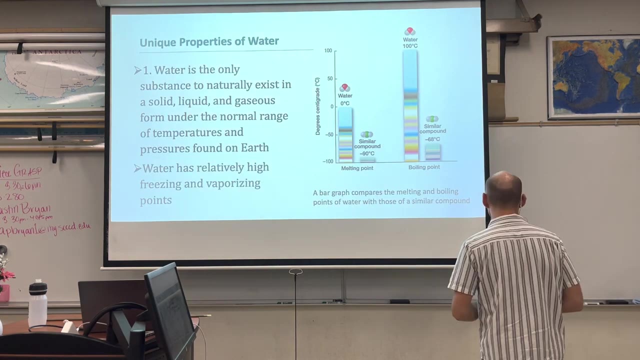 its atomic level, that the way that the hydrogens and the oxygens bond together and the way that water molecules bond together with each other, helps to provide all these great characteristics, of which we'll get into. so here is number one, the number one interesting property of water, that is, 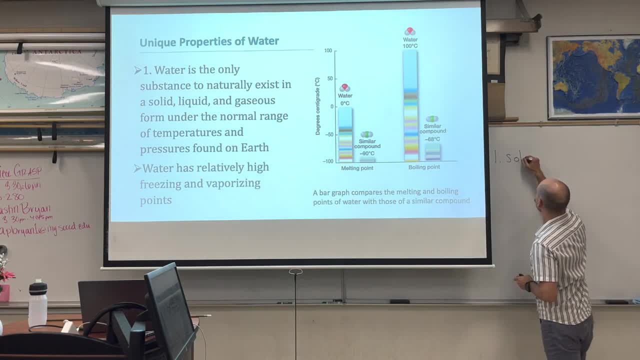 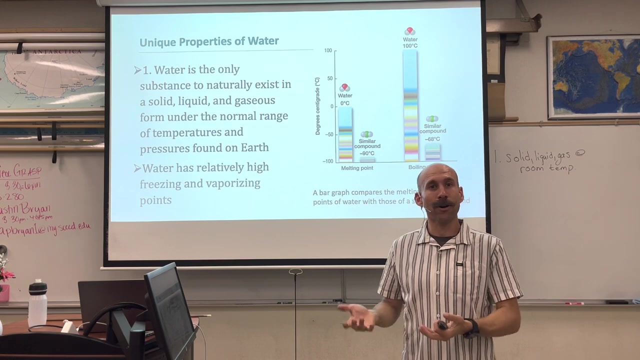 unique to water in and of its own is that it is a solid liquid and gas at room temperature. so there's water vapor in the atmosphere, there's ice in glaciers and there's liquid water on earth, all three of these through the normal range of temperatures that are experienced on earth's. 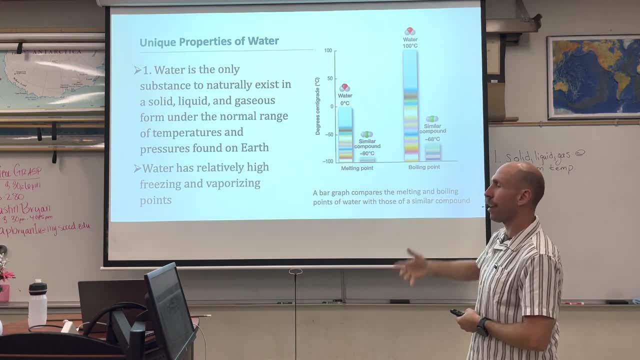 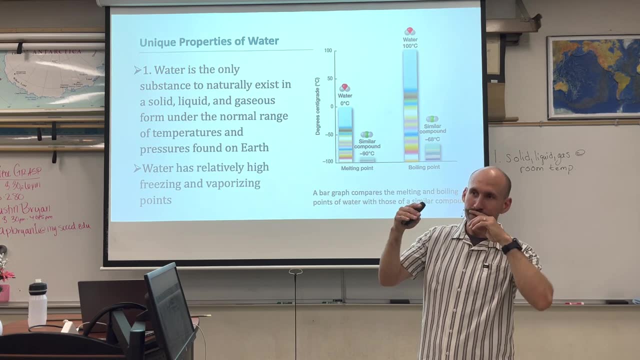 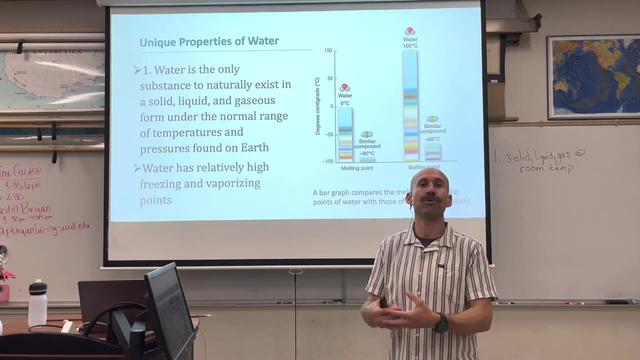 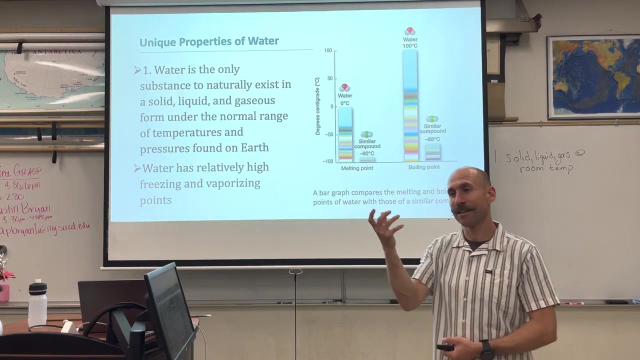 surface. other similar compounds do not do this. rocks are solid at earth's surface and, excuse me, deep down in the atmosphere. there's water vapor in the atmosphere beneath the surface. it takes incredible temperatures for them to melt into molten material, but water, being what it is and shaped the way that it is, has this extremely unique property. 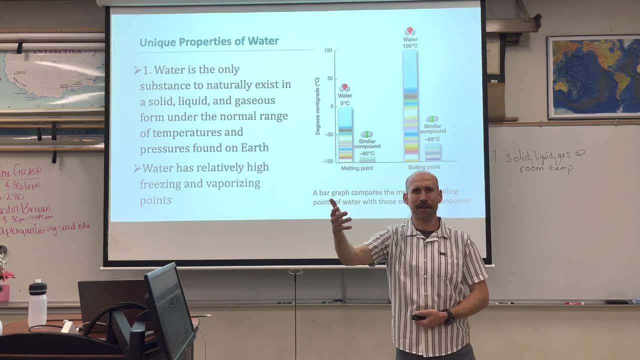 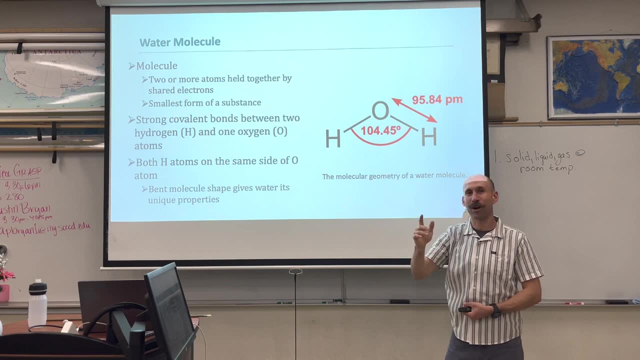 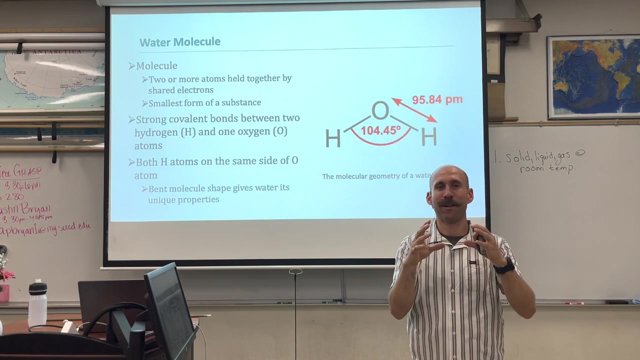 okay. so the question is: why does this happen? why is water so unique? and the answer has to do with the shape of the water molecule. now, this is absolutely amazing: h2o- two hydrogens, one oxygen- are sharing electrons to form a molecule. in this molecule, the orientation of the hydrogen. 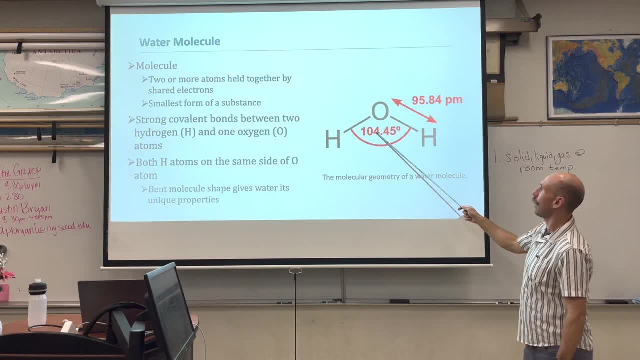 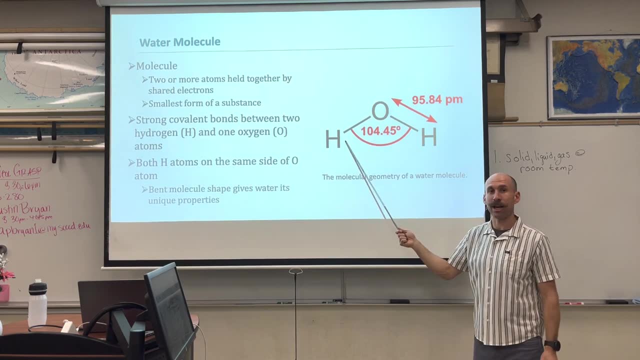 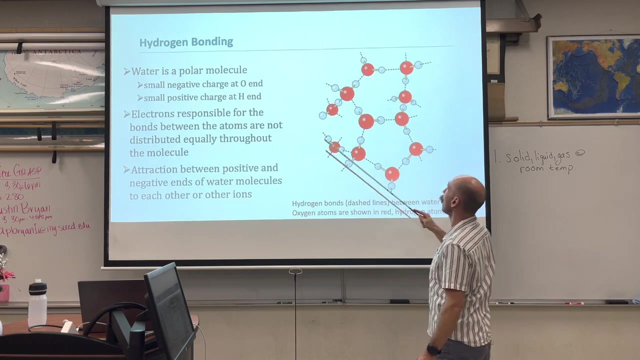 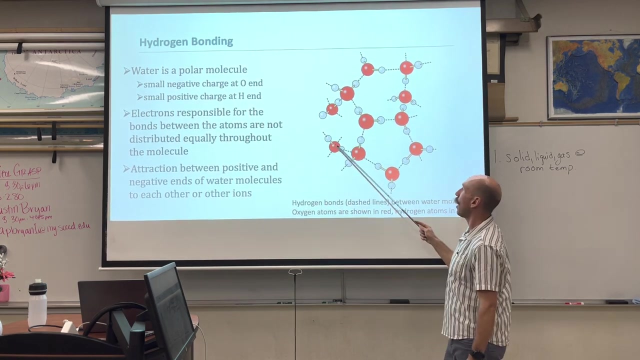 is offset, so they're both on one side and they're separated by about 105 degrees. now, and Captain Lawrence goes on, by his contrasty you can see this bent shape of the water molecule that gives it such unique properties: absorption in the atmosphere, isוג蘇 andr hai2. that gives it such unique properties. but not only that, it is also a polar molecule, which means that there's a small negative charge on the oxygens, there's Eptinger. 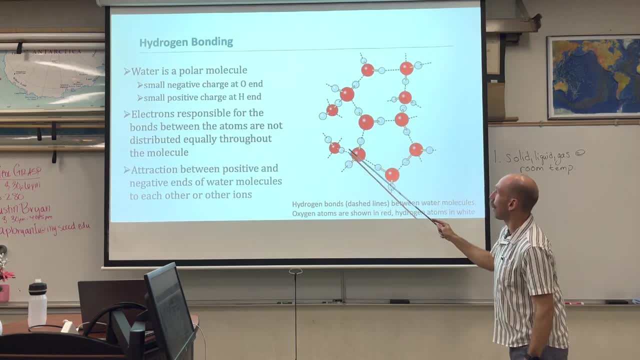 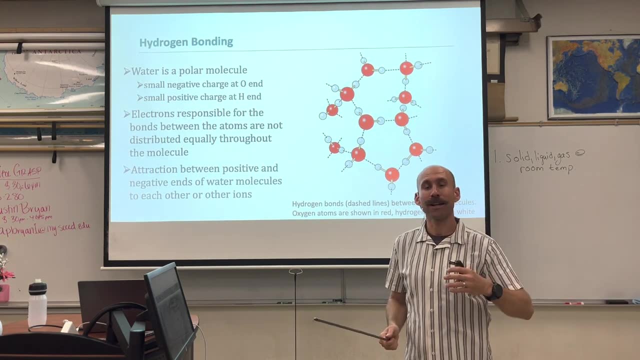 there's Eptinger through this very unique pattern of hydrogen bonding. Now, there's not a lot of substances in the world that have hydrogen bonds, and this is one reason why oil and water do not mix, even if you separate, if you've stirred them up all together. 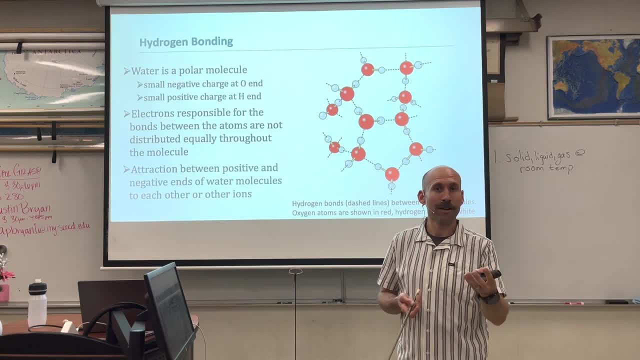 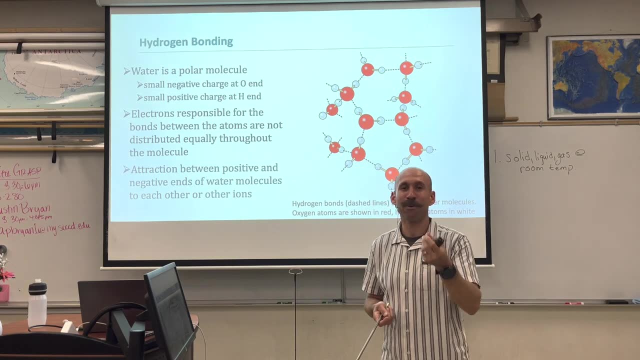 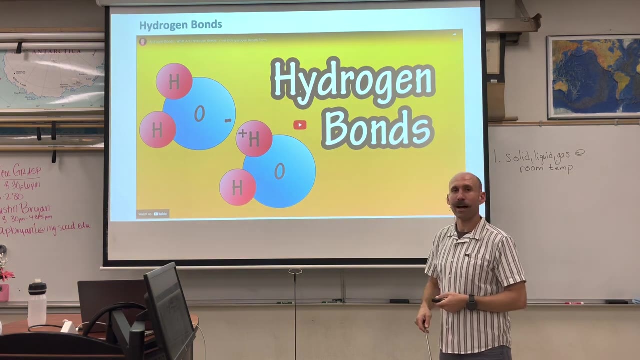 Well, it's because the water and the oil, the elements, don't actually bond together, so those two stay completely separate. Please watch the video on hydrogen bonds associated to learn more about this very unique process. You will also see the example of the olive oil and the water in this video. 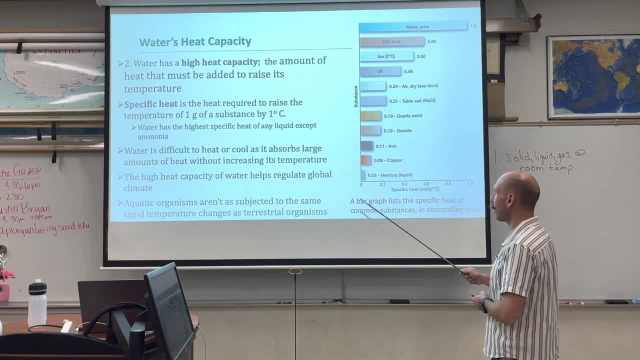 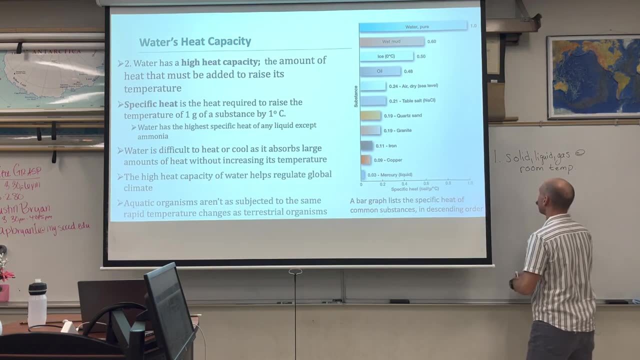 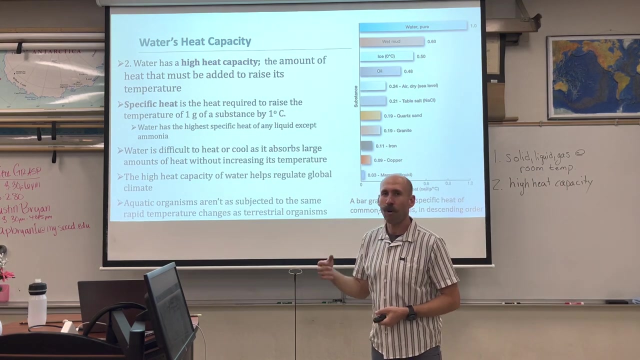 so please go There, check it out. Okay Now, water has a lot of unique properties. This one may be my favorite. This is water's high heat capacity. So what the heck does this mean? Well, basically, this means that water is really difficult to heat up or to cool down. 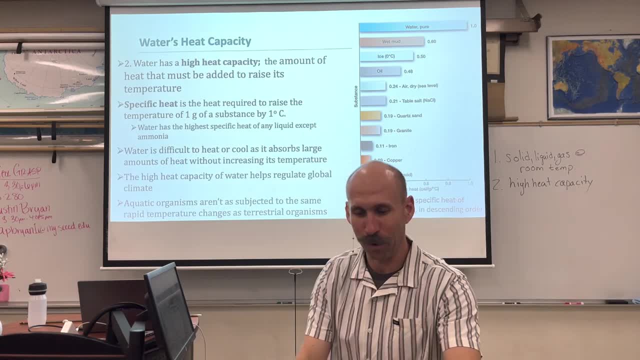 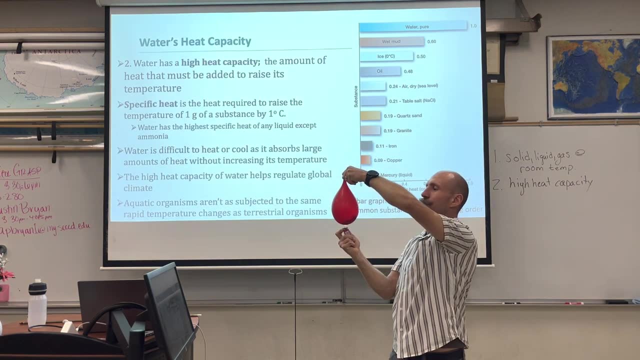 because it has a great heat capacity. It can absorb a lot of water. So here I have a water balloon and this is a lighter. You will see I have a video on this also. but hey, what the heck, I've got this in front of me. 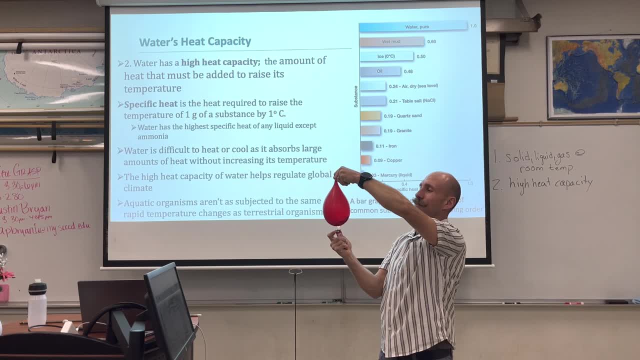 Let's just do this right now. So as the flame touches the balloon, the heat from this flame goes directly into the water, The water absorbs it And therefore the balloon does not melt, it does not burn, It does not pop. No, In fact, the high heat capacity of water means that 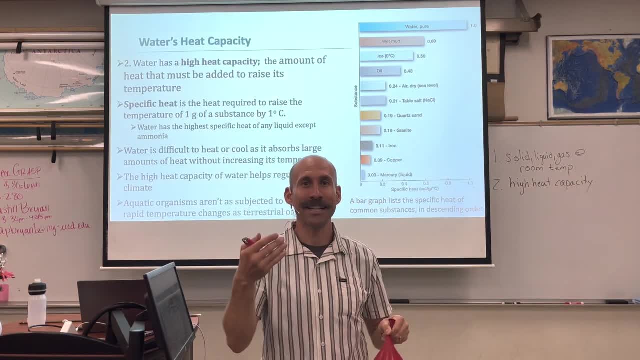 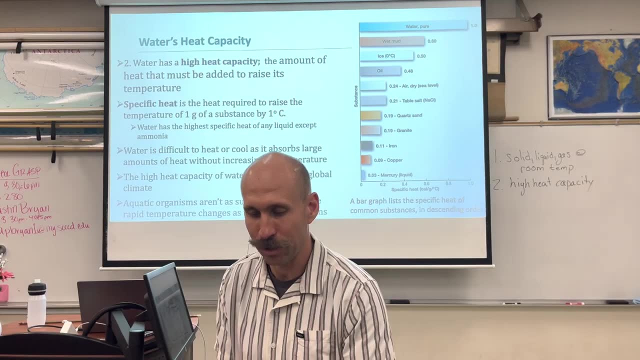 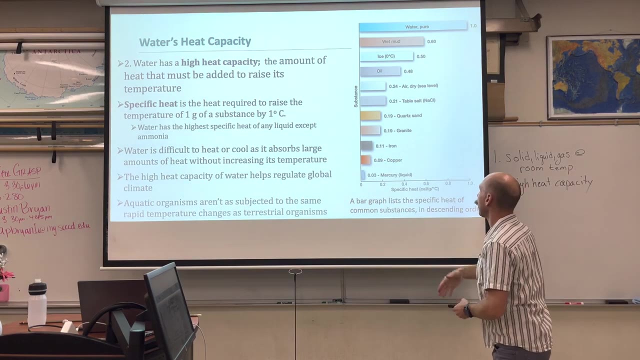 the water absorbs heat without changing its temperature. A lot of heat has to go into it for water to change its temperature, And this is the heat capacity of water. We can see a bar graph of various substances. What I want to highlight here, for us to notice, is that water has an incredibly high heat capacity: quartz, sand and granite. What are those Continents? Land Land has a lower heat capacity, So if you are at the beach on a hot day, the sun will heat up the sand, so hot sometimes that your feet will burn. But the sun doesn't. 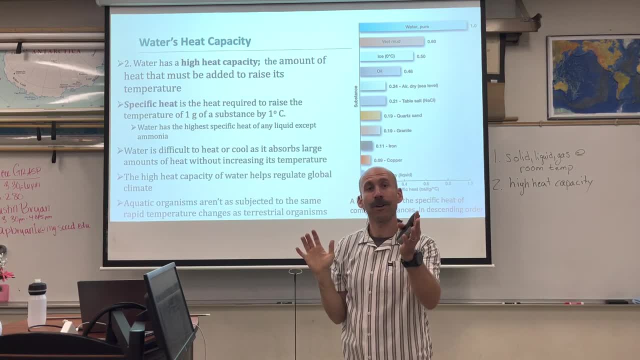 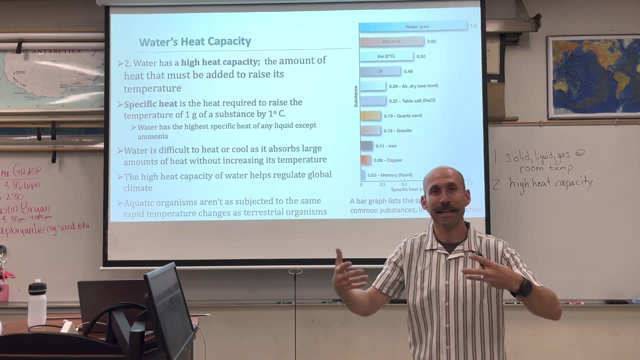 heat the water up. So if you are at the beach on a hot day, the sun will heat up the sand, so hot that's right next to the sand at the ocean. this is because the water has a high heat capacity. It can absorb a lot of heat without changing its temperature. Now there's another quality. 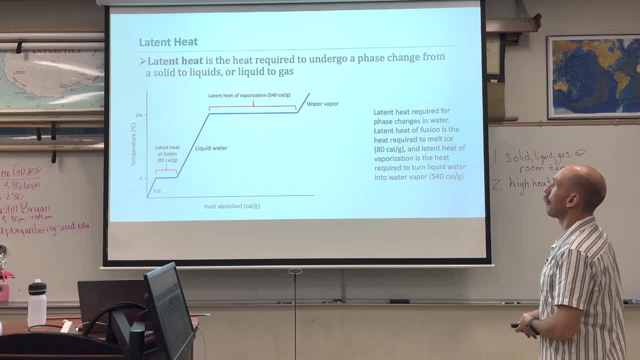 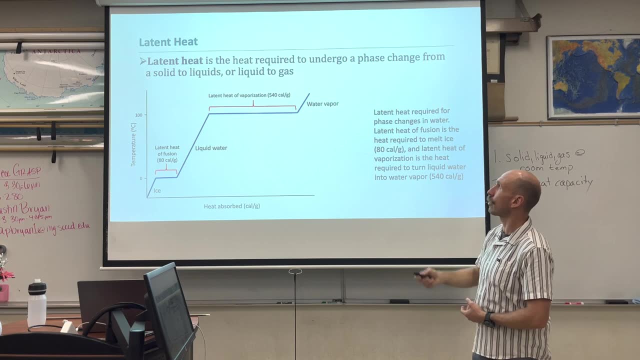 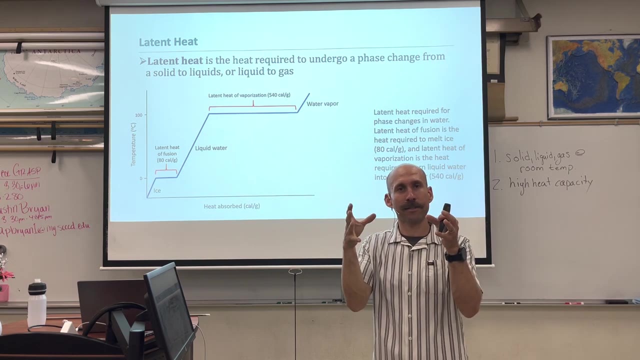 of water, called latent heat right, And this is the amount of heat required to undergo a phase change from liquid to solid or liquid to gas. And the way that I can exemplify this is now: imagine you have a block of ice and it's 112 degrees outside. It's roasting. 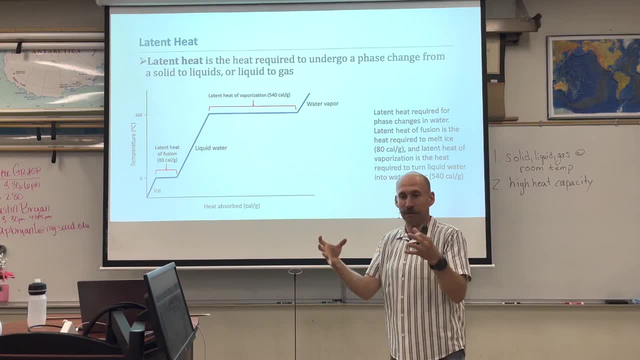 Goodness gracious, it's so hot. But you go outside and you take this block of ice and that ice, it sits there and it absorbs heat. That ice, it doesn't just melt. What's going on there? Well, it's absorbing heat without changing phase. First, it has to 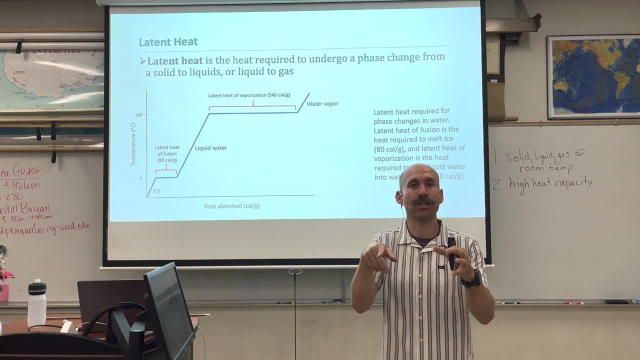 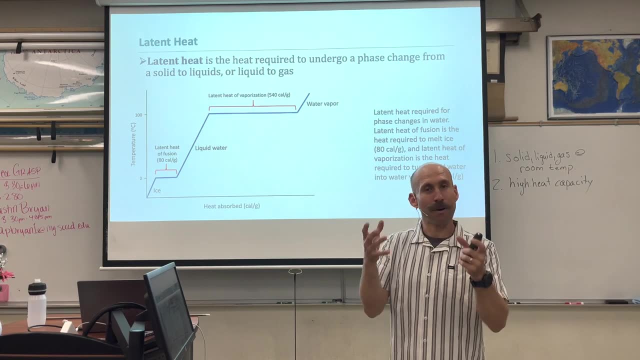 absorb heat. Second, it has to absorb heat. Third, it has to absorb heat. Fourth, it has to absorb heat, An incredible amount of heat, and then the phase change occurs. You also know this: when you boil a pot of water, You put the pot on the stove and you turn it on. Maybe you have gas, Maybe you have. 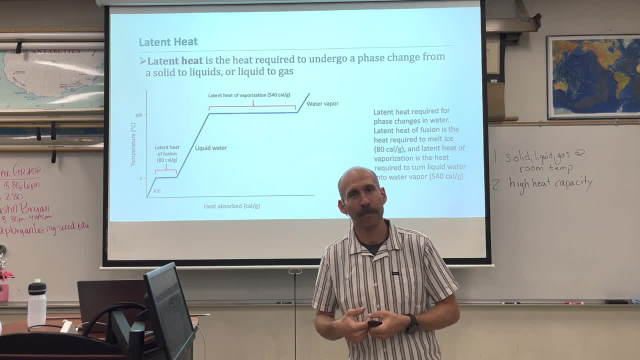 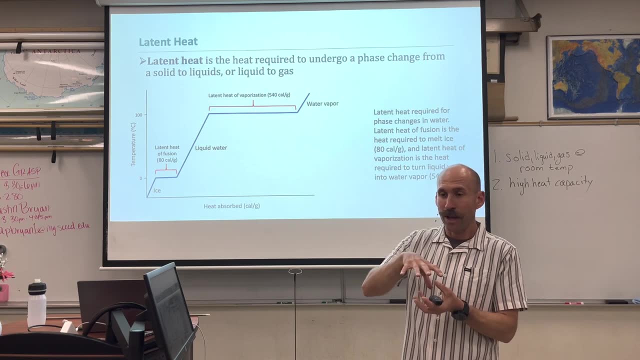 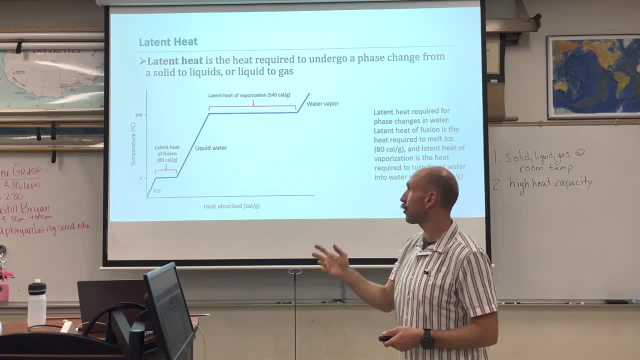 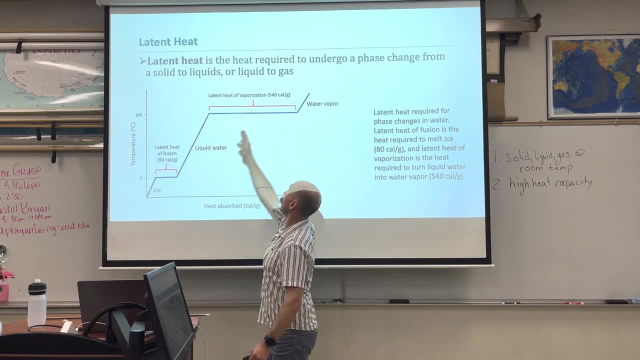 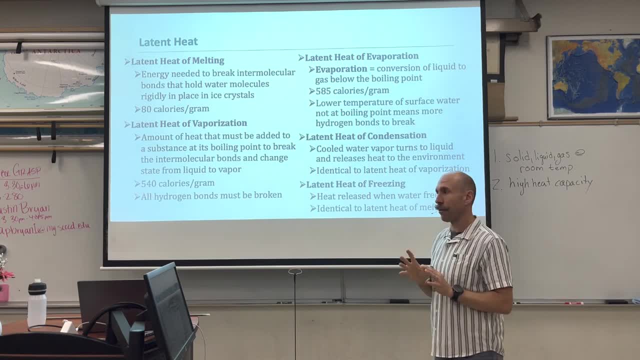 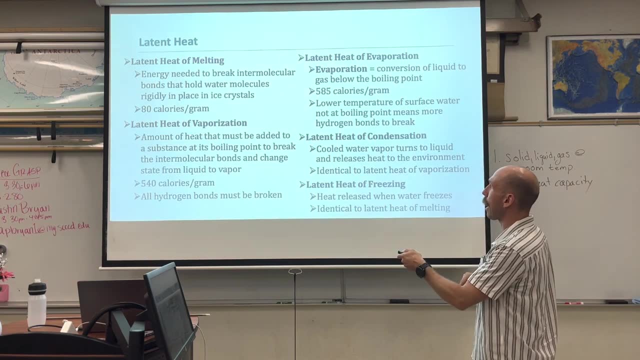 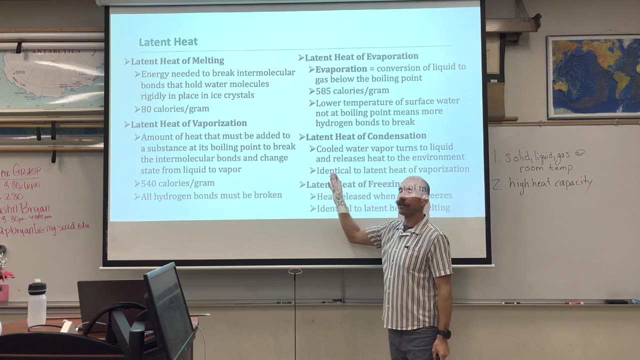 name. So I'm not a fan of all tech slides. I apologize for this. But to get these definitions in one place, here we go. Latent heat of melting and vaporization. latent heat of evaporation, condensation and freezing. Now, these are basically the heat that it takes to move. 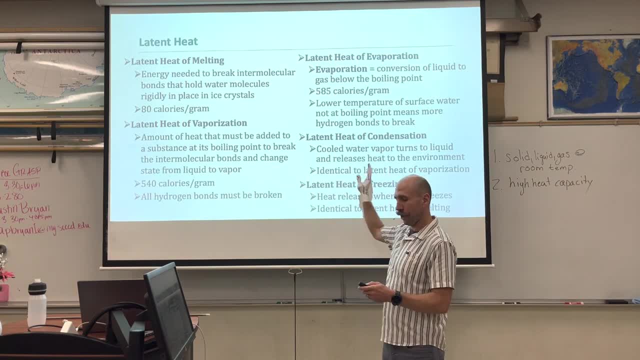 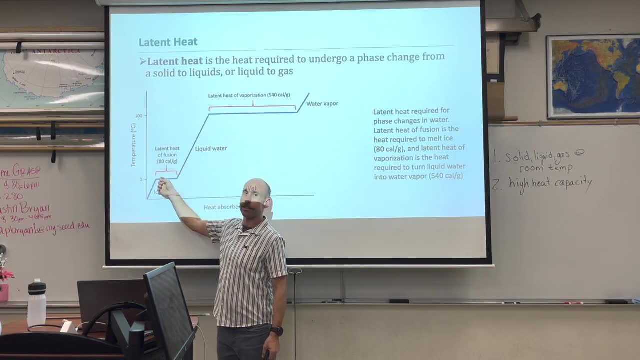 from one phase to another in either direction. So, without going too far into these, the concept I really want you to know is: when ice gets to zero, it doesn't just melt into liquid, It absorbs heat before that phase change occurs And then, before liquid water can turn to water vapor. 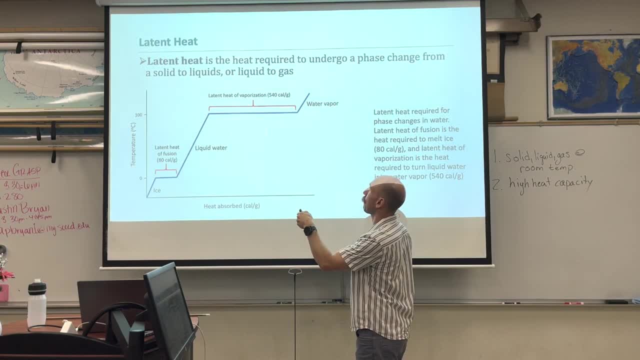 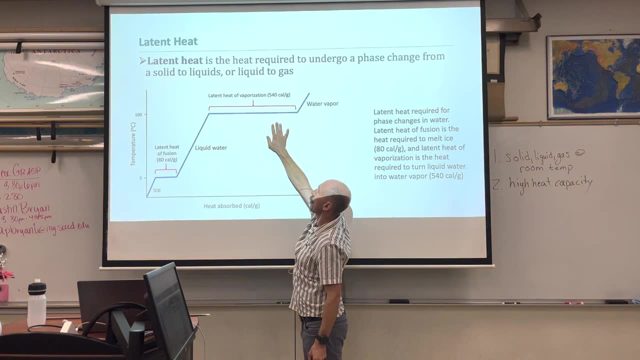 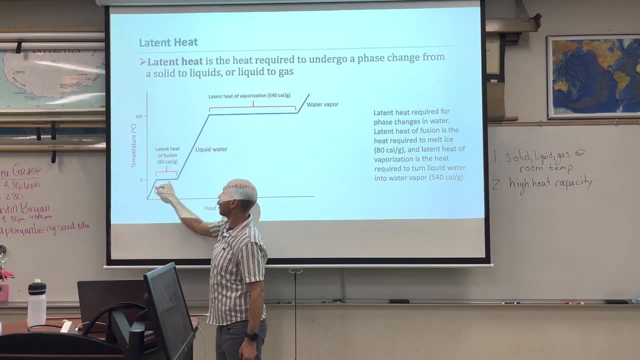 it has to absorb a whole heck of a lot of heat- about 500 calories per gram. Same thing in the opposite direction: For water to condense into liquid, it has to lose a lot of heat. The temperature drops And then the same thing: a lot of heat has to be. 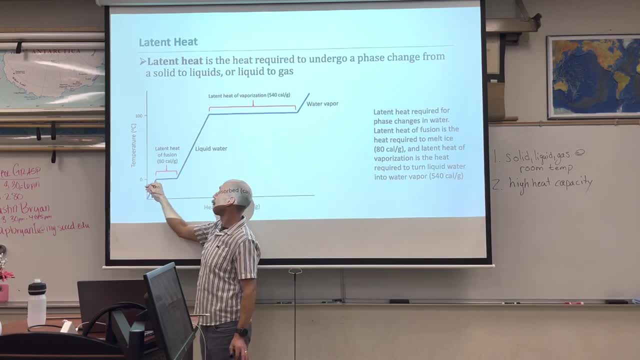 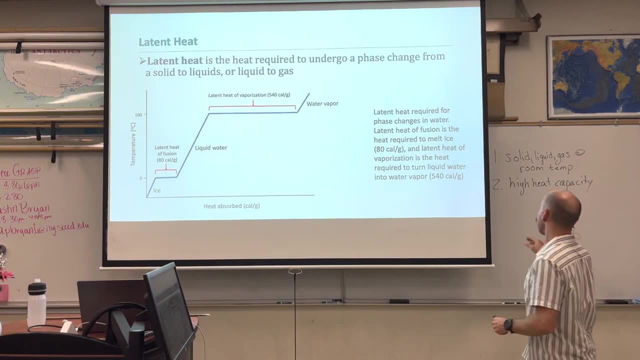 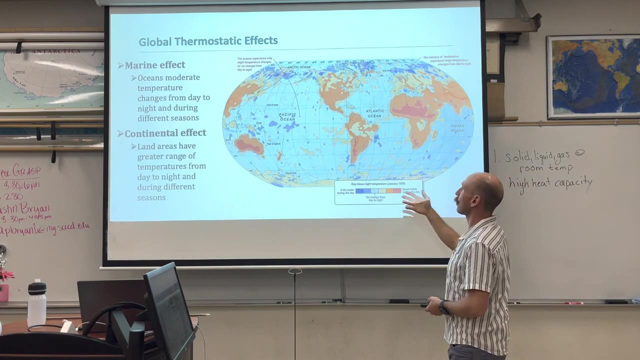 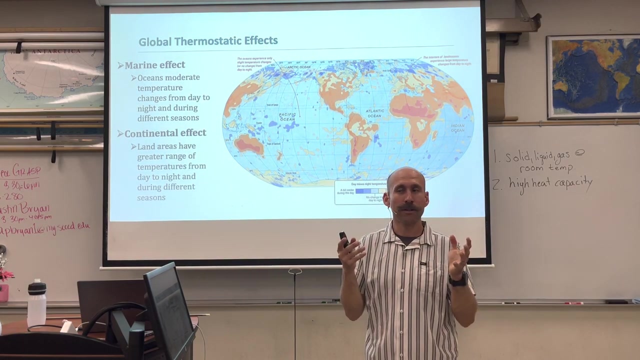 absorbed out of it or released, that is, before liquid water will freeze into ice. So exciting, Important, unique property. number two: water's high heat capacity. What this does is it creates marine effects and continental effects. Land heats up, cools down, Water stays relatively. 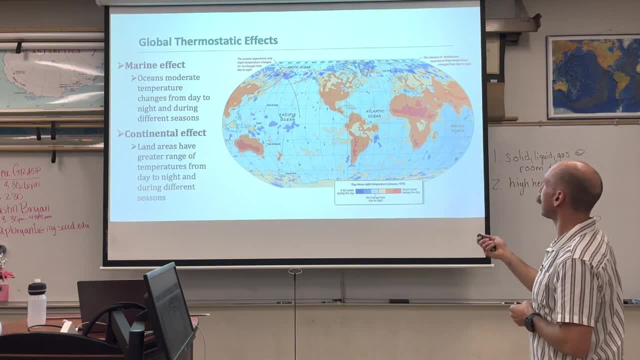 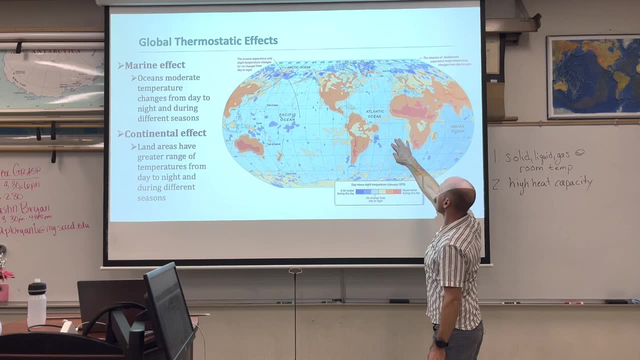 stable. So if we look at the day minus night temperature- this is the temperature range- we can see that oceans exhibit relatively no change from day to night, And then land, as we see here, experiences significant change from day to night because land areas have a much 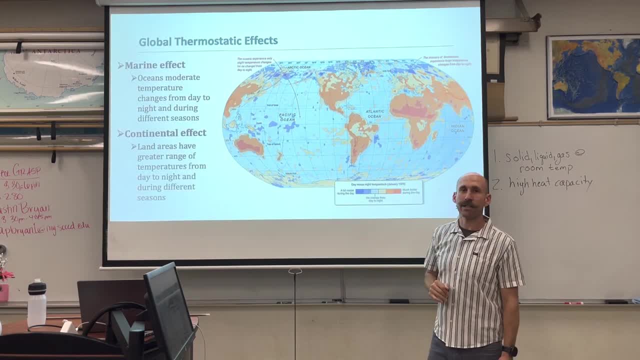 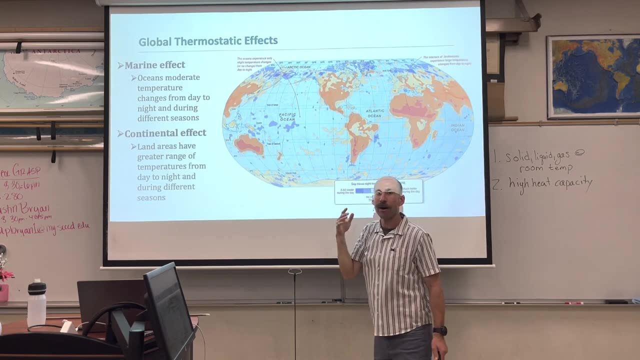 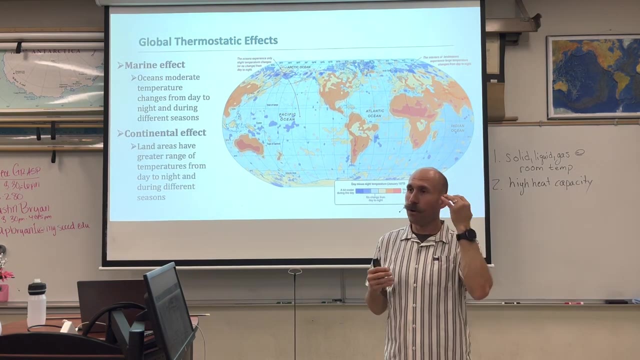 greater range of temperature from day to night during different seasons. where oceans moderate, the temperature changes from day and night throughout all the seasons. So this is why it's 112 degrees at home. You're like whew. oh, my goodness, what am I going to do? I got to get out. 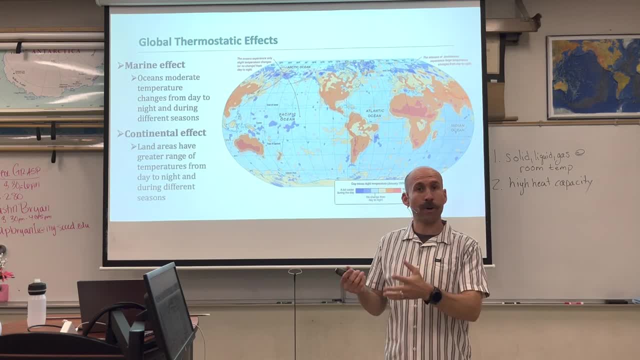 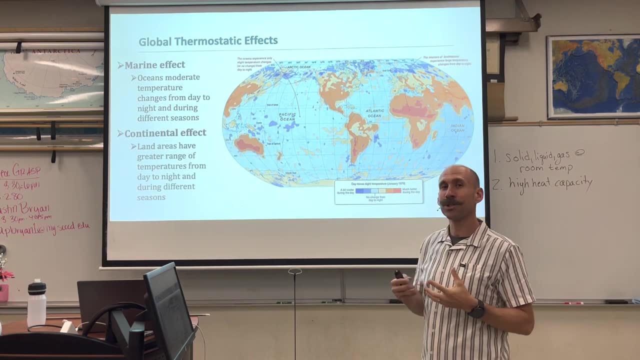 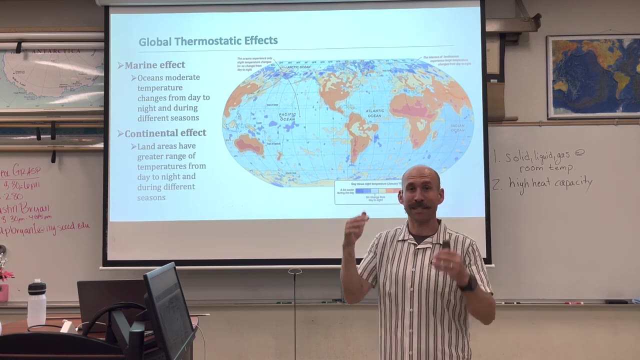 of here. Where do you want to go? Let's go to this study we've done so far. I'm looking forward to the beach. why? because of the marine effect, oceans are moderating temperature and we know that whenever we go to the beach it's a lot cooler. it feels the temperature is much lower. we can find a. 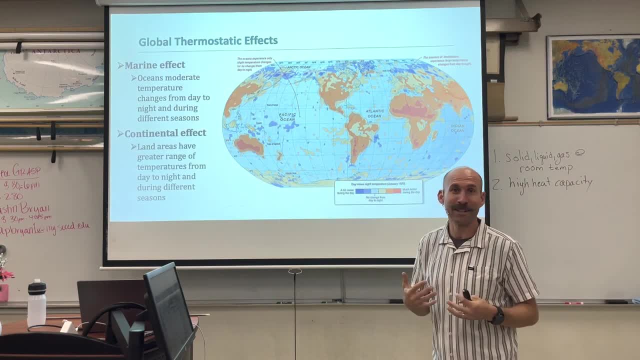 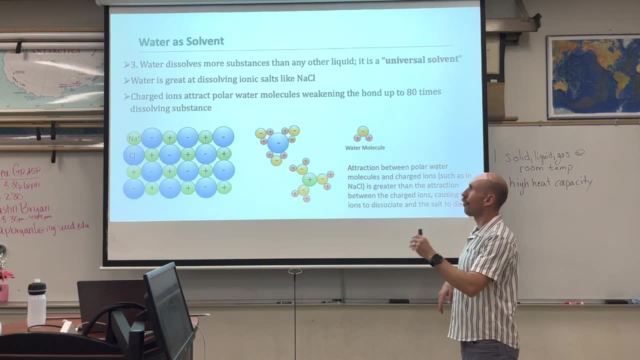 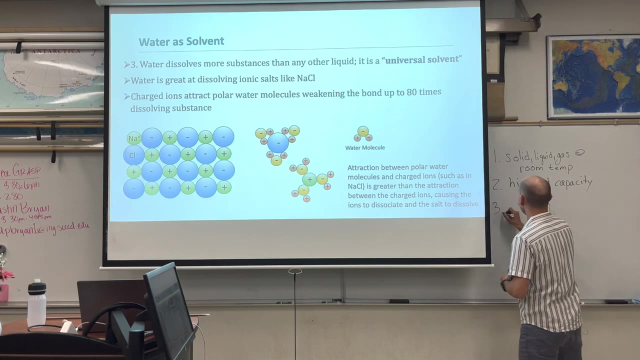 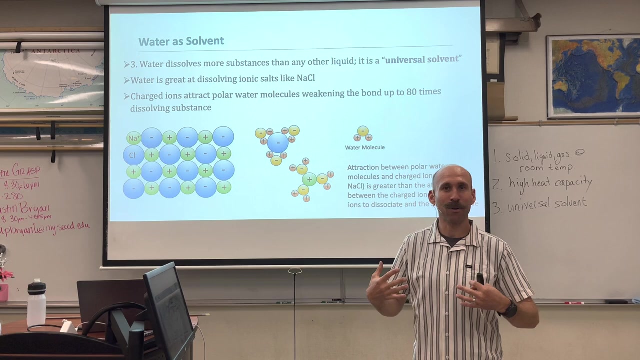 little respite from the enduring the hot temperatures that have been coming our way through central valley summers. water is a solvent, so this is the important property. number three: water is known as the universal solvent because of the unique properties of the polar molecule. here we go again: chemical oceanography. let's talk about this, the polar. 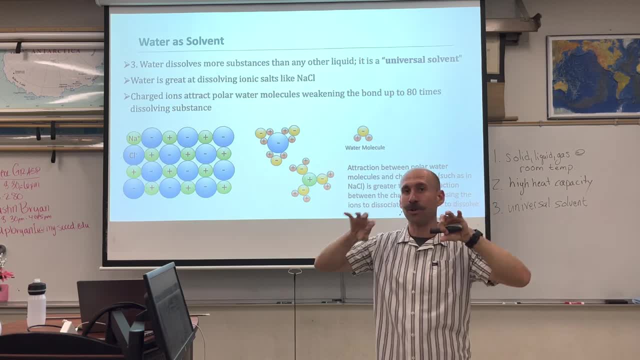 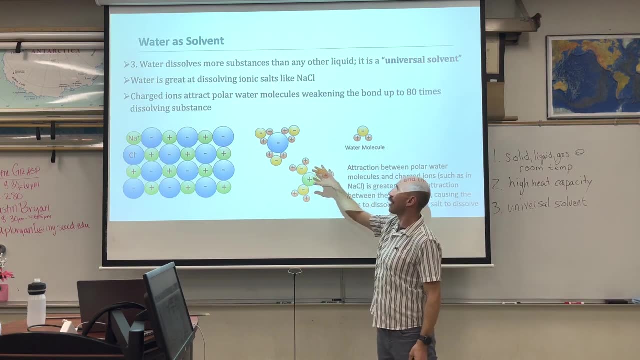 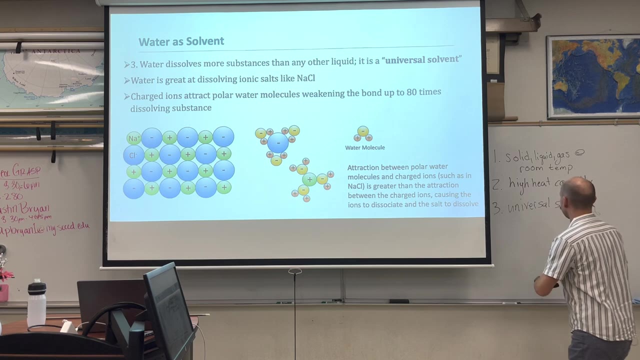 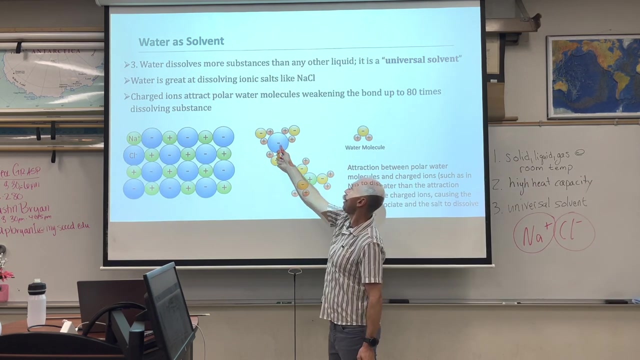 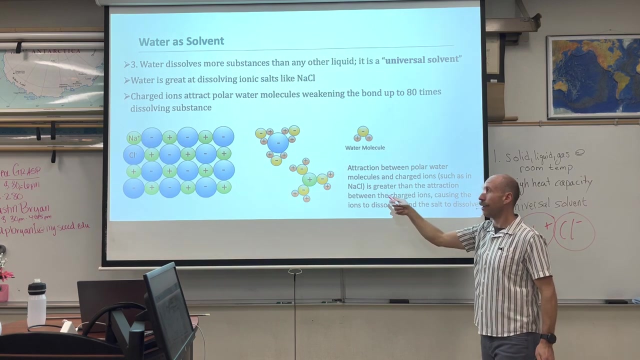 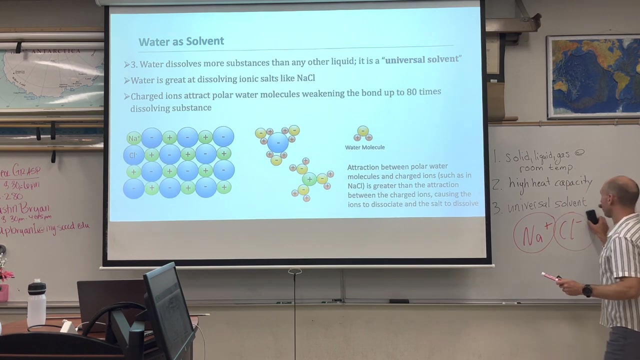 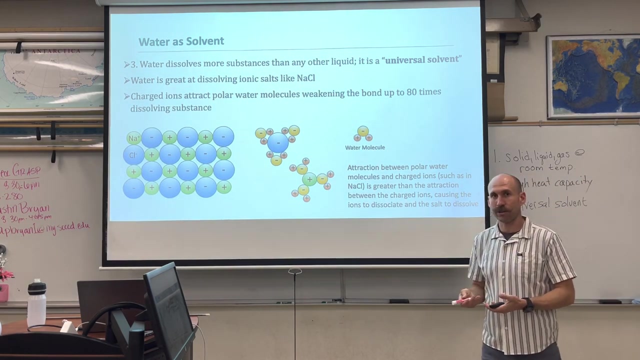 molecule over beer. not just that did the from the maximum ocean, Hij inar. only there earth solution 야 ground and bond, keeping that ion in solution bonded to the water molecule. This is an amazing feature of the oceans. This is kind of the nuts and bolts of how the oceans are salty And we'll 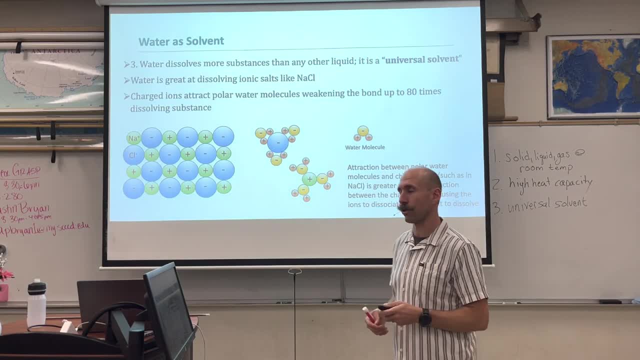 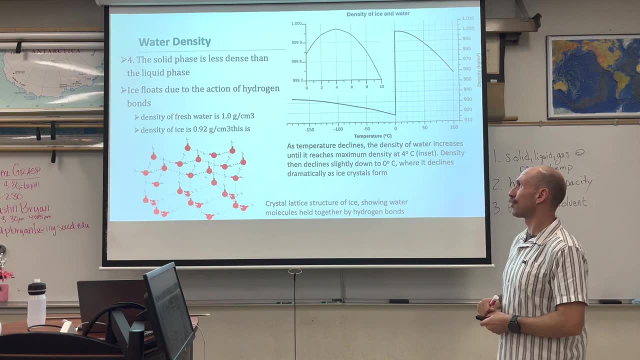 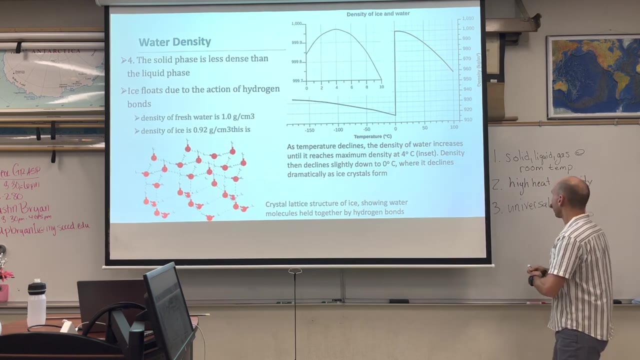 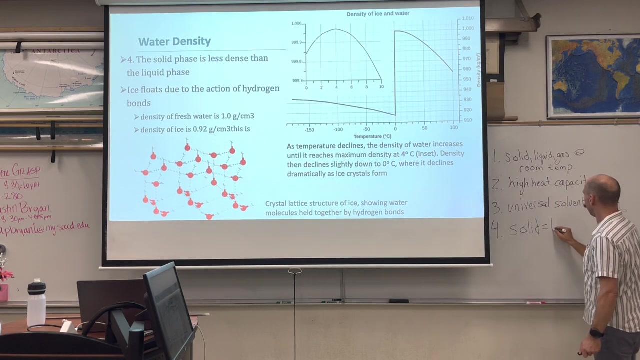 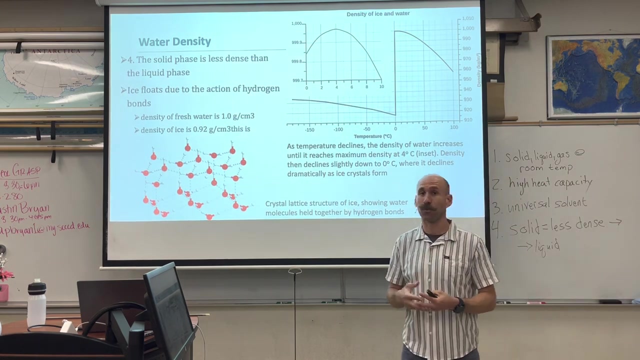 talk about more why the oceans are salty here coming up. So number three: water is the universal solvent. Number four: the solid phase is less dense than the liquid phase. Solid is less dense than the liquid phase And then liquid. Essentially, what we're saying here is that ice floats And it's a really good 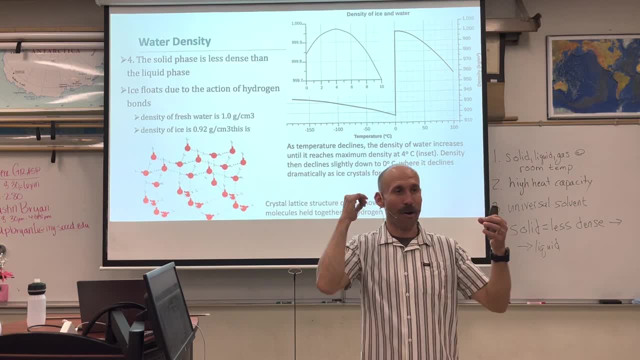 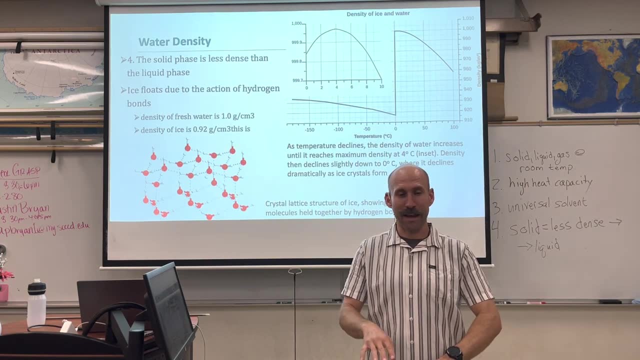 thing that ice floats, because if ice sank, then all the water, all the frozen sea ice would sink to the bottom and it would accumulate, And then it would accumulate, and it would accumulate, and it would accumulate and accumulate, and so on and so forth, until the oceans were frozen, And then 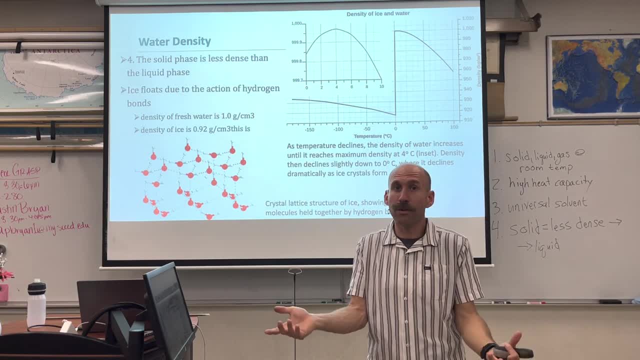 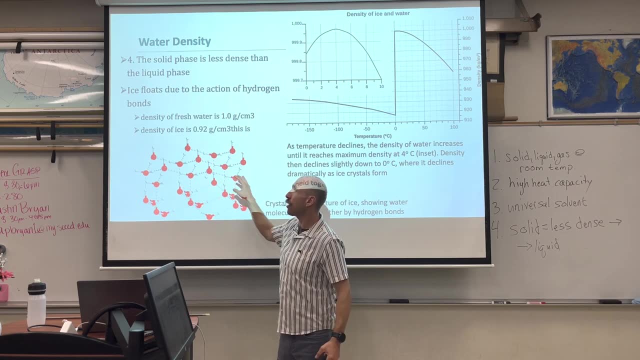 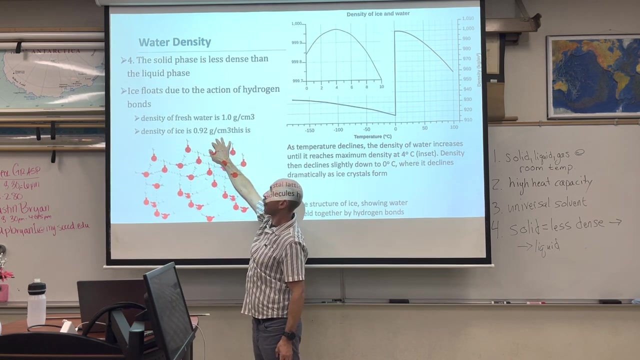 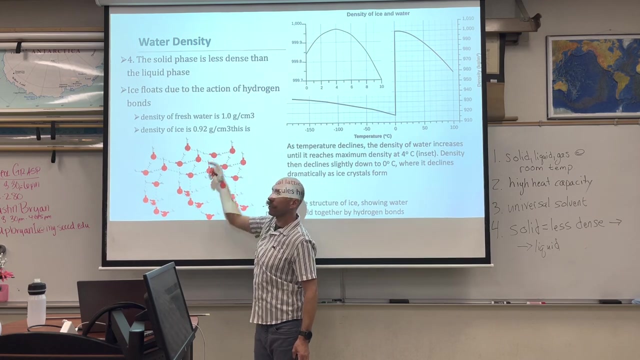 there's no life living in the frozen oceans because they're frozen. And so thank you water for the way that you bond in these frameworks where, when you have free-floating molecules into weekly bonded, into framework bonded, the density of water actually decreases. Water, fresh water is about 1 gram per cubic centimeter, Ice, 0.92 grams per cubic centimeter. So Вы хоть swim на нratos и все темно rituals. So when вода вы Decrease in the nous, water actually decreases. Water: fresh water is about 1 gram per cubic centimeter, Ice 0.92g per cubic centimeter. 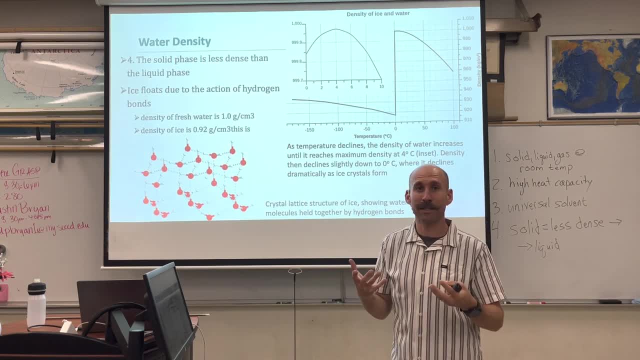 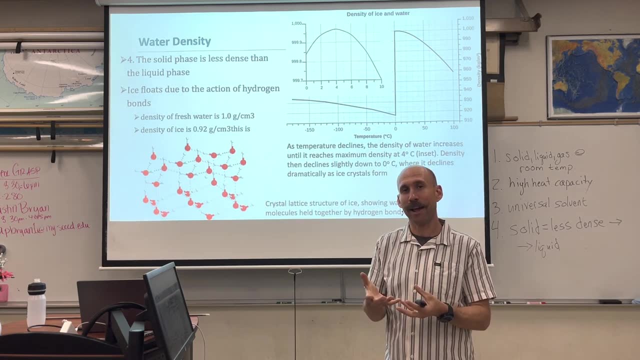 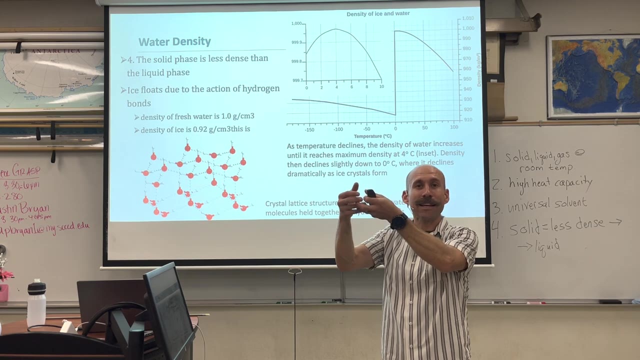 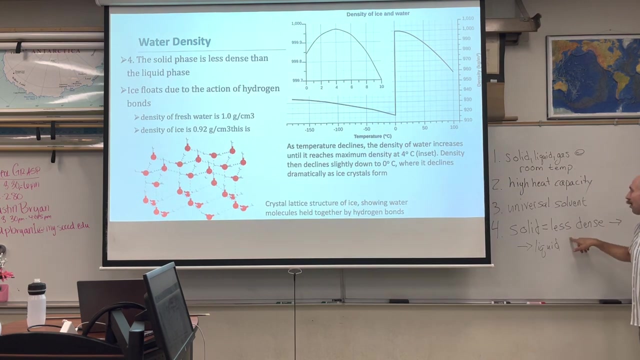 So when? and this is very unique to water, because most substances are more dense in solid form than less dense. water, on the other hand, freezes, and its solid form is less dense than its liquid form. thus ice floats. thank you, water, for your solid being less dense than your liquid, that's. 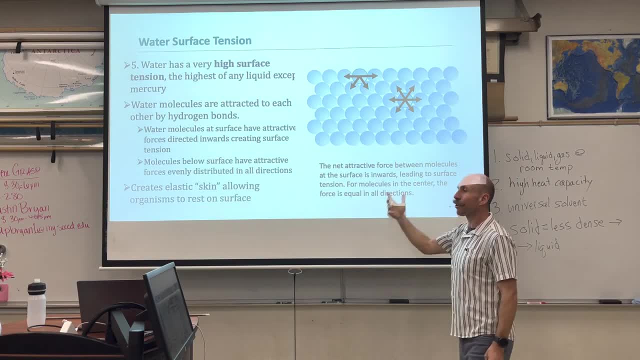 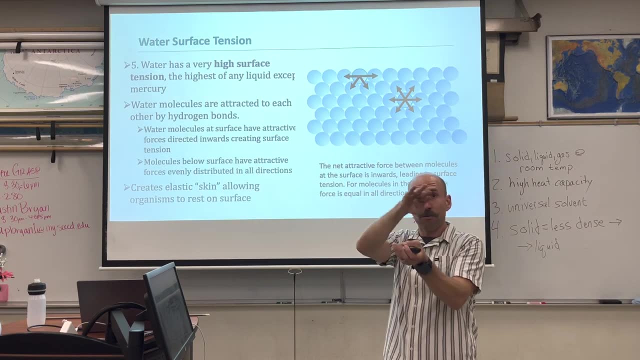 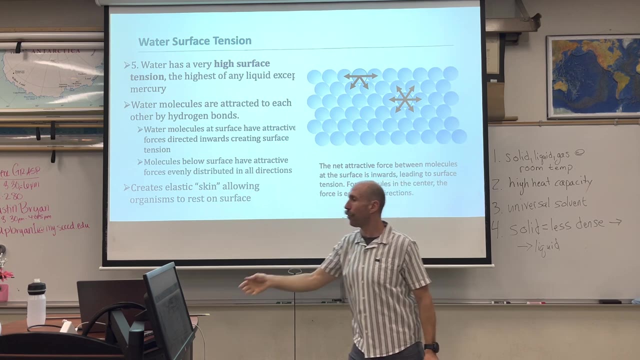 awesome. okay, number five: water has a very high surface tension. there's capillary action on the top. if you've ever filled up a cup of water too full, you'll notice that there's a little dome shape on top, and this is because there are attractive force forces below the surface of 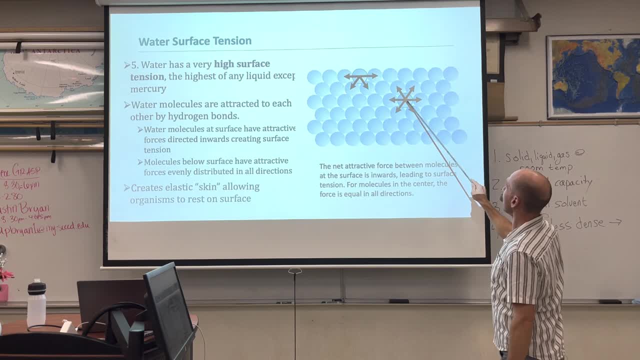 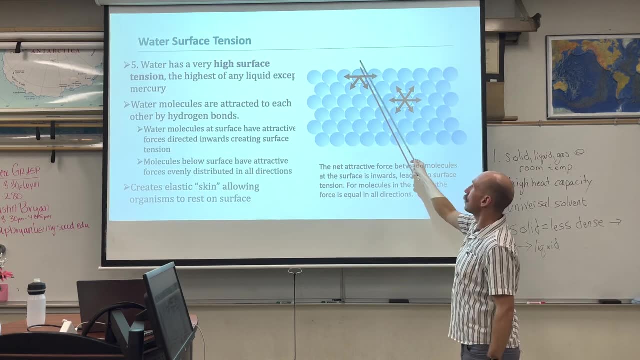 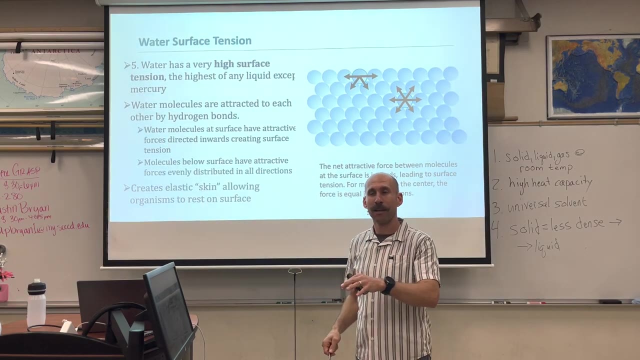 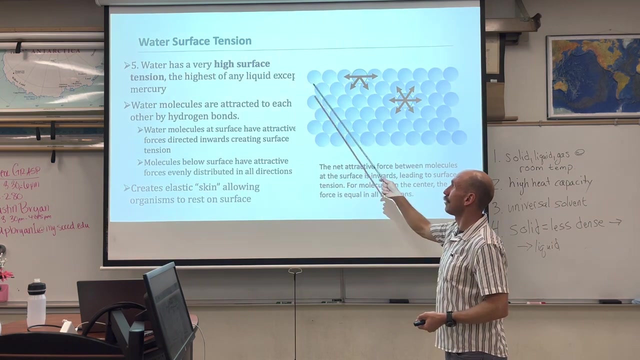 water, they are equally distributed in every direction. at the top of the surface, the attractive forces go into the mass of water. what this does is it gives an elastic skin that allows aquatic organisms to rest on top. some birds can sit right on top of the sea water. what the heck is going on there? well, that's because water has a 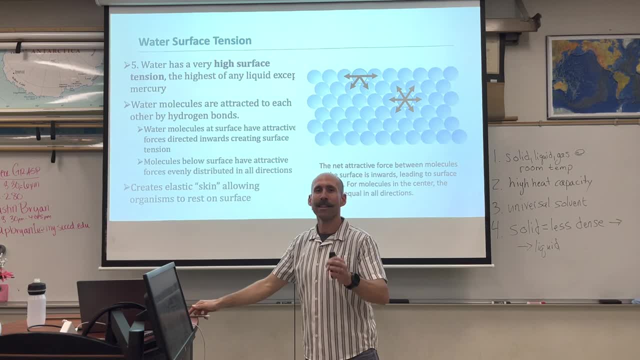 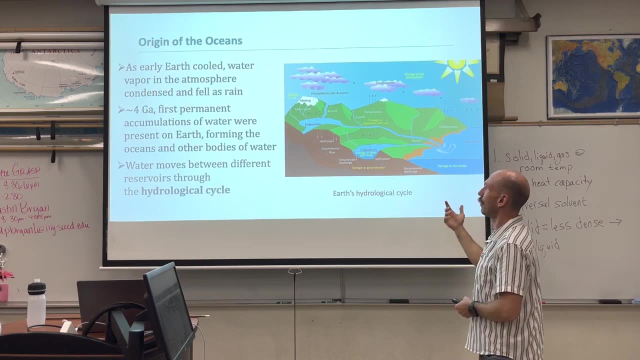 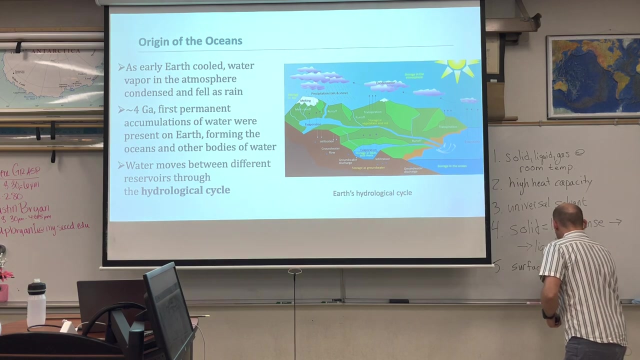 high surface tension. so again, thank you, water, for your very unique characteristics. now let's review that real quick, actually okay. so water is amazing. we'll put number 5. number one: water exists through normal surface temperatures freely in a liquid, a solid and a gas. in the save. the amazing number two: water has 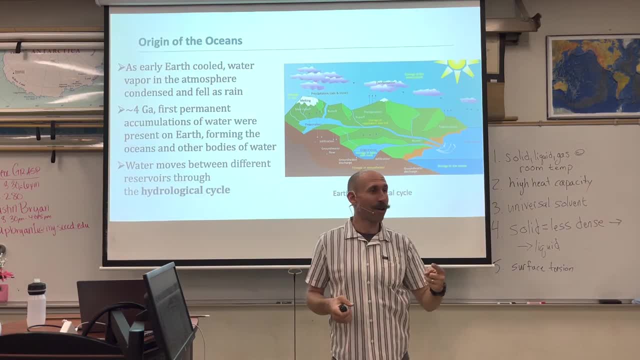 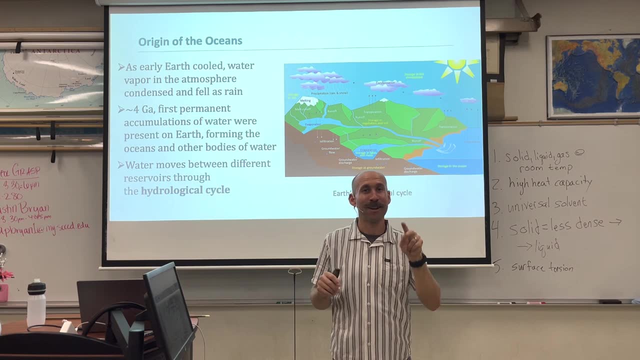 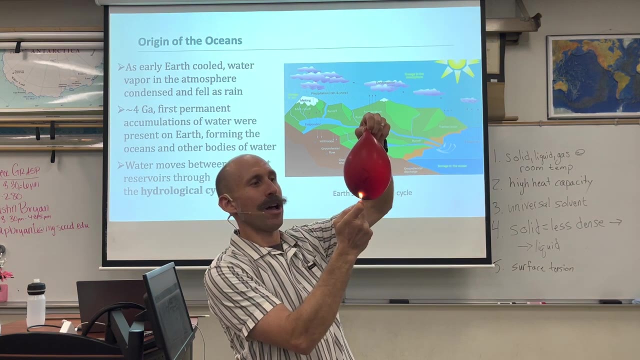 an incredibly high heat capacity capacity for each of these soils. so thank you all. right now, a goodüe- we got a little insta also, you're welcome- and ability to absorb heat. i think i could just leave this on for the rest of the lecture, but 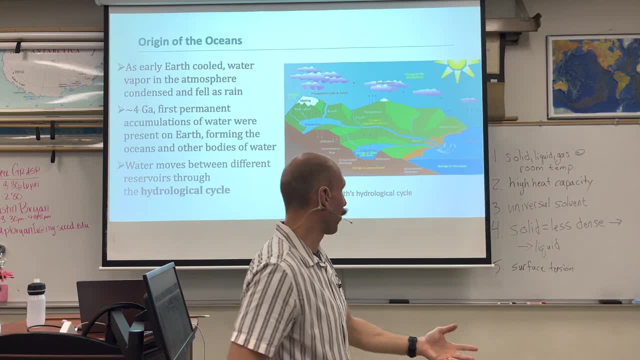 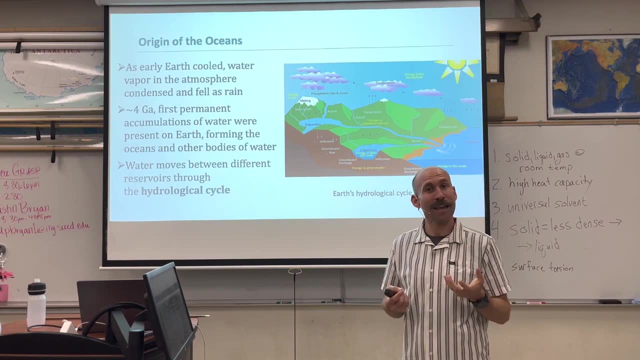 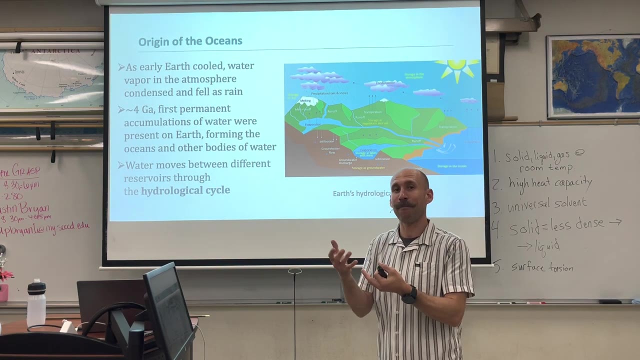 nope, we got to keep going, so let's keep going. number three: water is a universal solvent. it can dissolve a myriad of different substances, like putting sugar in your coffee or a powdered drink. right, the whole reason that we have powdered drinks is because of this unique property of 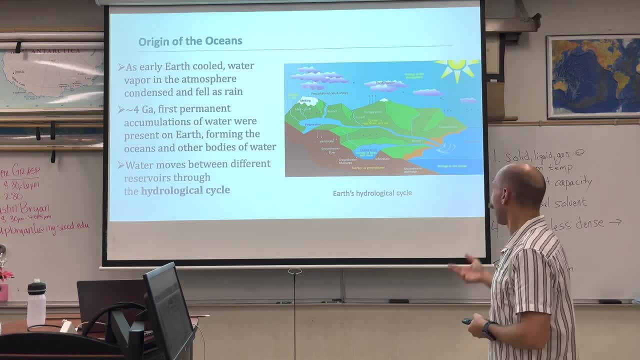 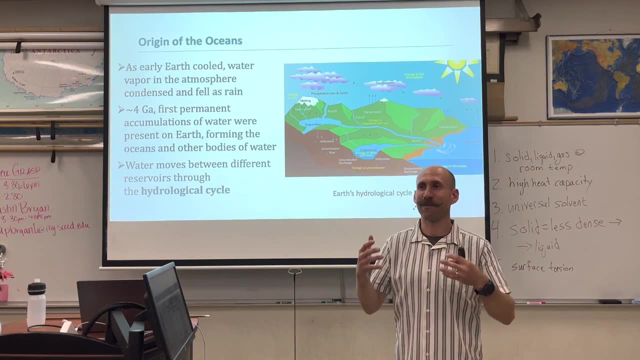 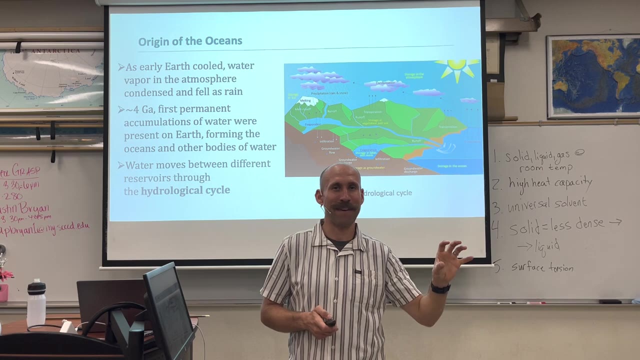 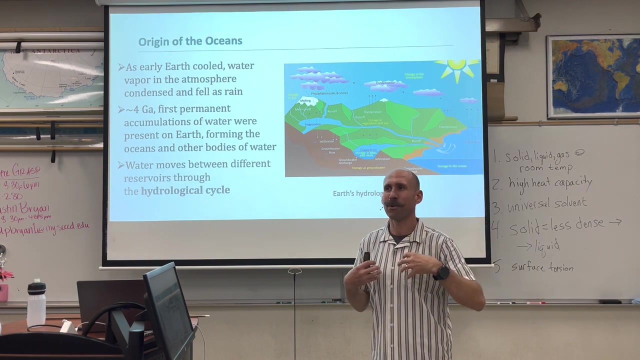 water, that it is a universal solvent. uh, we've got the solid fate. the solid phase less dense than the ice phase- ice floats. let me restate that the solid phase is less dense than the liquid phase, meaning ice floats. that's so cool, that ice floats, thank goodness. i am just so personally happy that. 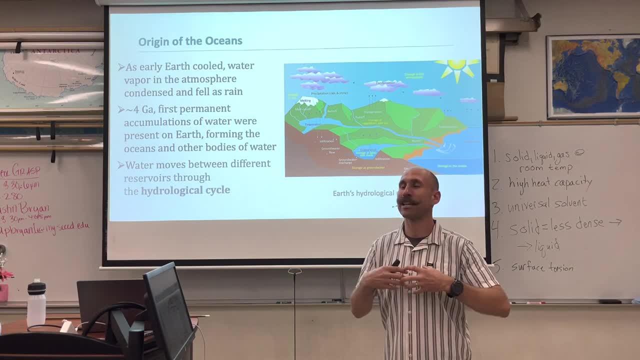 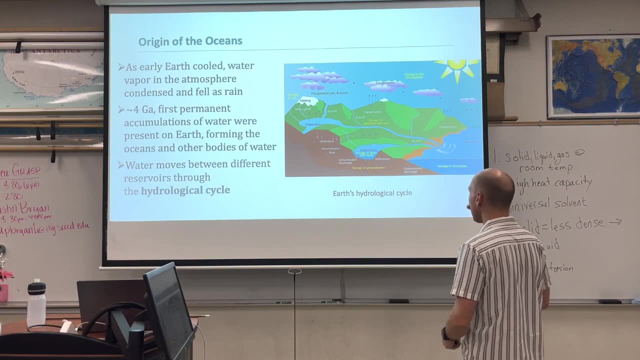 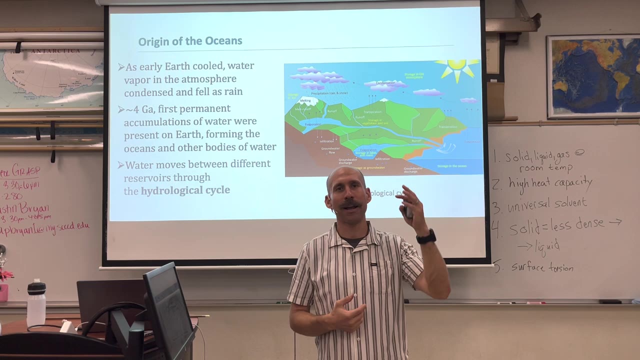 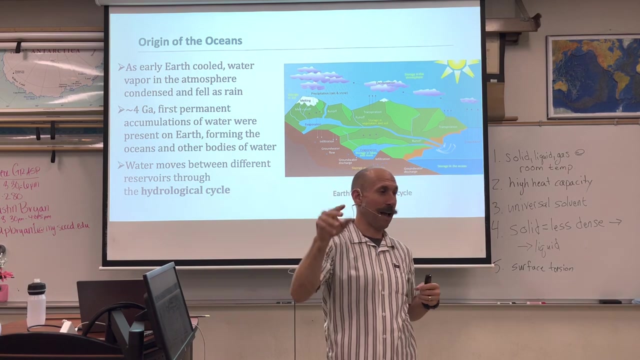 ice floats and also the surface tension of water is extremely heavy, allowing for an elastic skin to develop on the top. okay, so where did all this water come from, anyways? well, let's go way back the origins of earth, around four and a half billion years ago. the late heavy bombardment through this period was bombarding- for lack of a better word- the earth. 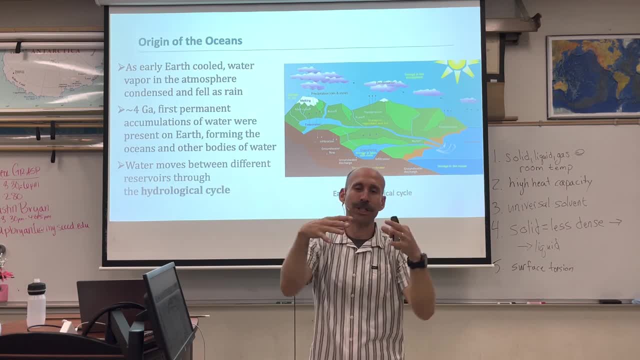 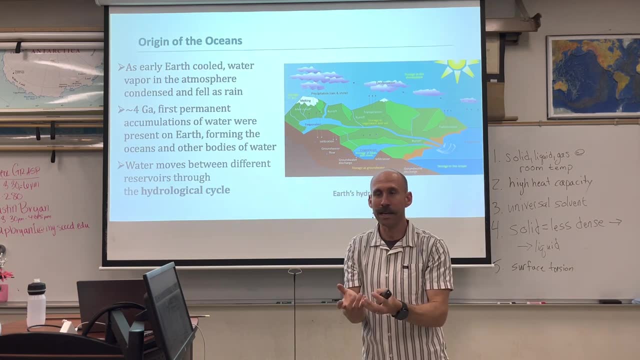 with comets that had ice. the earth was differentiating into its compositionally distinct layers of core mantle crust, and the earth was differentiating into its compositionally distinct layers of core mantle crust, and the earth was differentiating into its compositionally distinct layers of core mantle crust. plate tectonics were beginning. 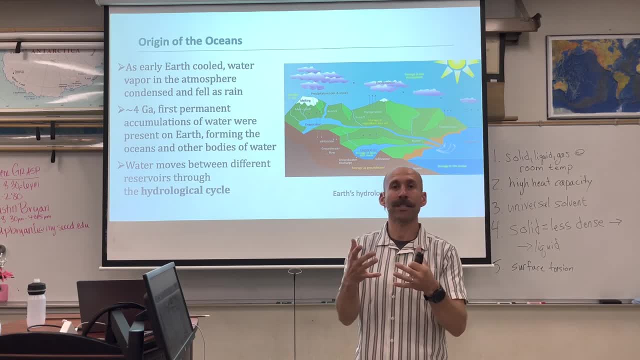 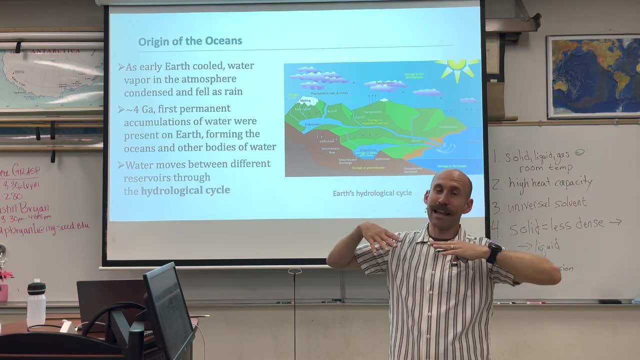 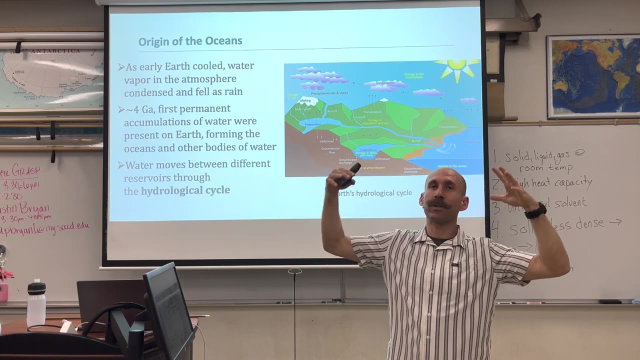 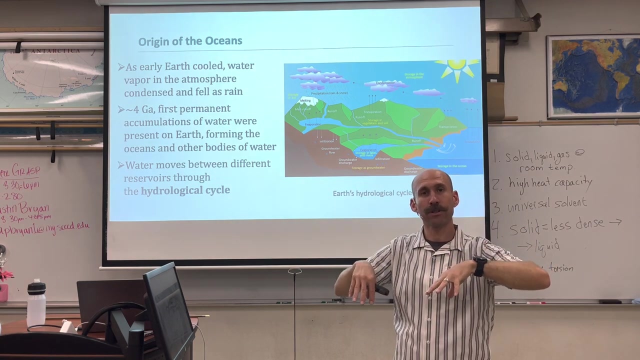 plate tectonics were beginning and the movement of heat and material through earth's interior led to volcanoes. those volcanoes erupted and outgassed water into the atmosphere. in over about half a billion years, that water was able to collect, condense, precipitate and form pools on the surface of the earth that we know about. 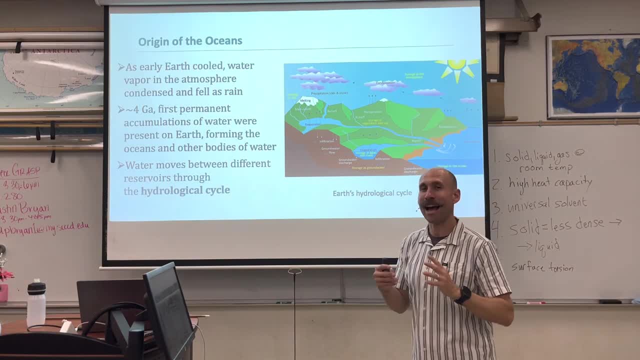 half a billion years that water was able to collect, condense, precipitate and form pools on the surface of the earth that we know about. half a billion years that water was able to collect, condense, precipitate and form pools on the surface of the earth that we know about we now call earth's oceans. it's a fantastical story and i love thinking about the origin of earth and the origin of the oceans. so as water began to fall, there was water everywhere: water in the atmosphere, water in the oceans, water in the ground, water frozen on top of mountains, water in lakes, water running over the river, water in vegetation and soils. 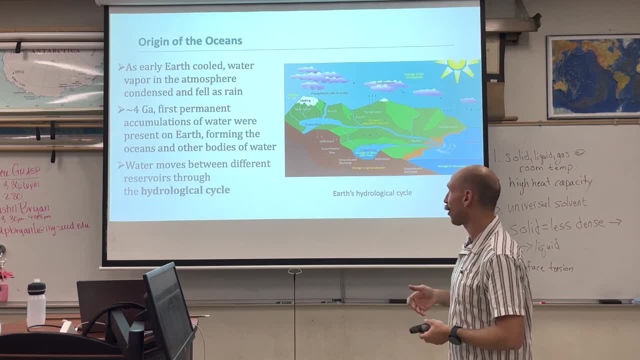 we now call earth's oceans. it's a fantastical story and i love thinking about the origin of earth and the origin of the oceans. so as water began to fall, there was water everywhere: water in the atmosphere, water in the oceans, water in the ground, water frozen on top of mountains, water in lakes, water running over the river, water in vegetation and soils. 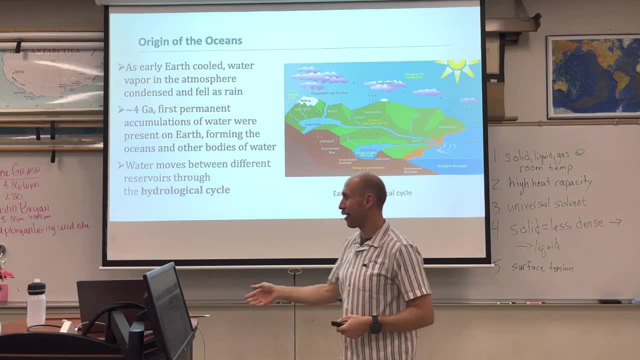 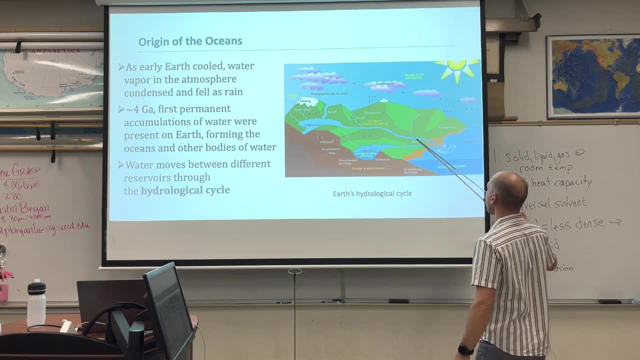 we now call earth's oceans. it's a fantastical story and i love thinking about the origin of earth and the origin of the oceans: water in the atmosphere, water in the oceans, water in the grounds, water frozen on top of mountains, water in lakes, water running over the river, water in vegetation and soils. 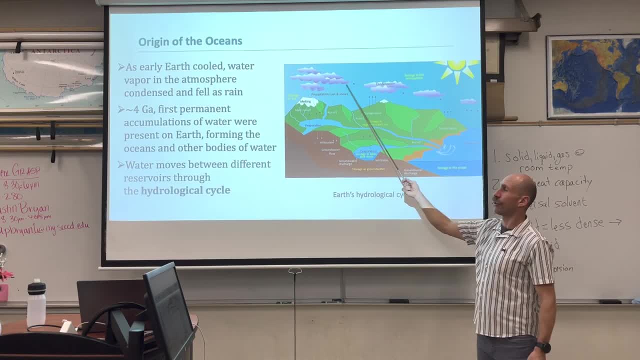 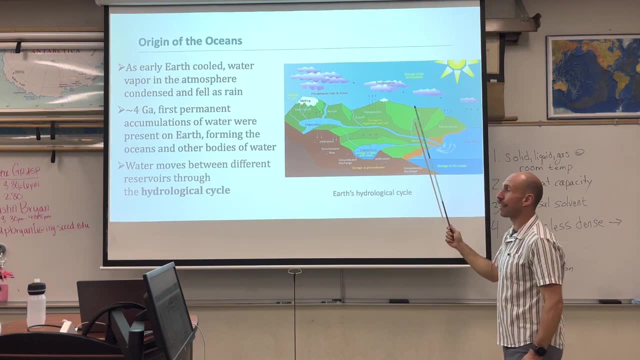 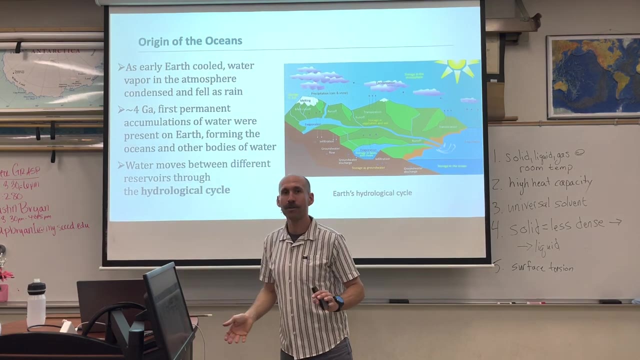 and so we call the movement of water, and so we call the movement of water through the earth system the hydrologic, through the earth system, the hydrologic cycle cycle. really amazing that this, really amazing that this exists, exists, thank you. thank you earth's early oceans, and thank you to our dynamic earth for having this complex system. 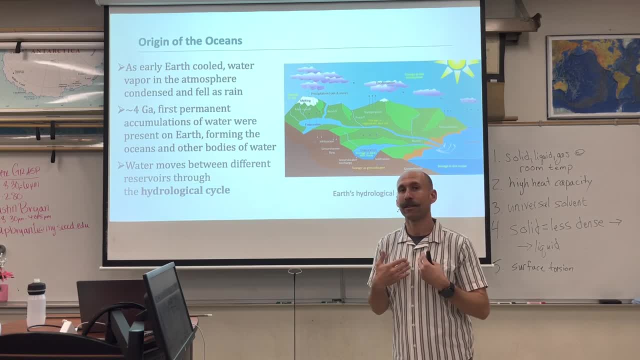 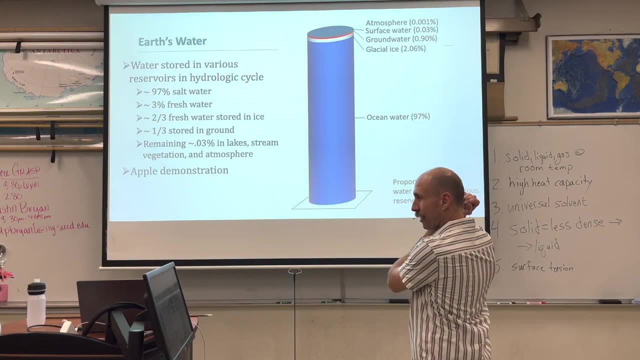 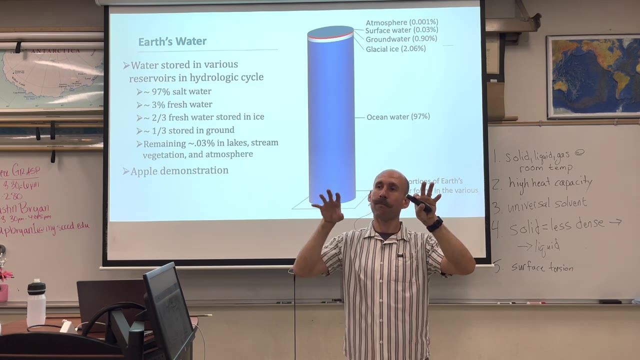 that helps support and sustain all life on earth, and you and i. so there's a lot of water on earth. where exactly is it okay if we talk about the distribution of water and land? we've got 70 percent water, 30 percent lands. let's take that land out. 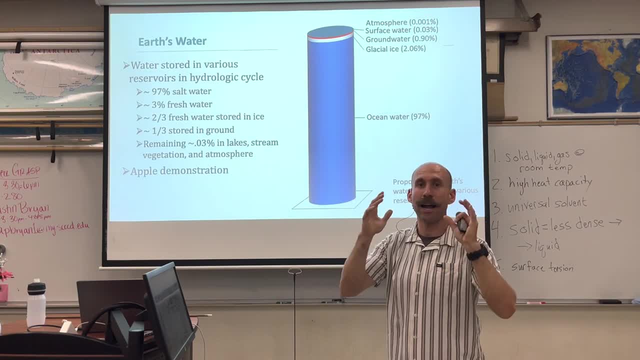 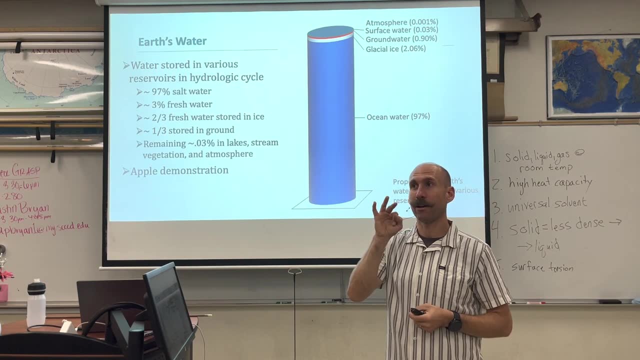 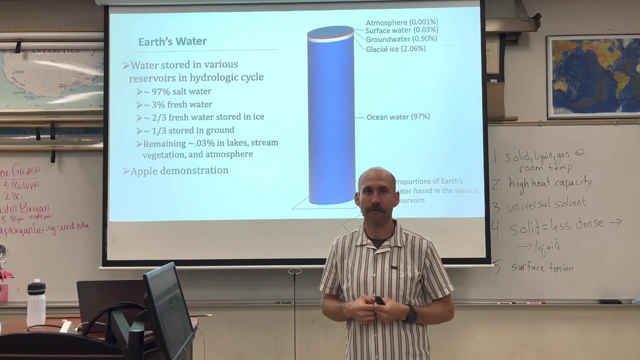 let's look at just the water on earth. of all of earth's water, 97 of it is in the oceans. that's a lot that remain that the three percent remaining is fresh water. so 97 salt, three percent fresh. of that three percent fresh water, about two percent is locked in glaciers, continental and alpine uh. 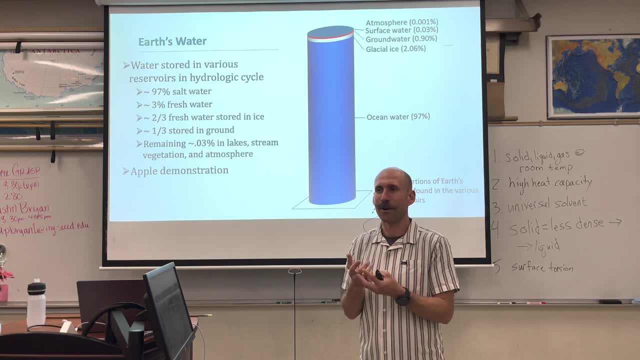 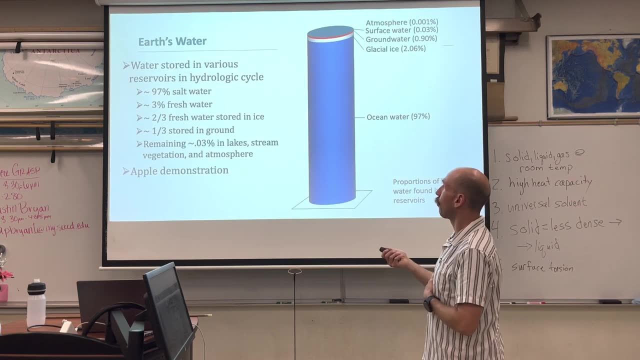 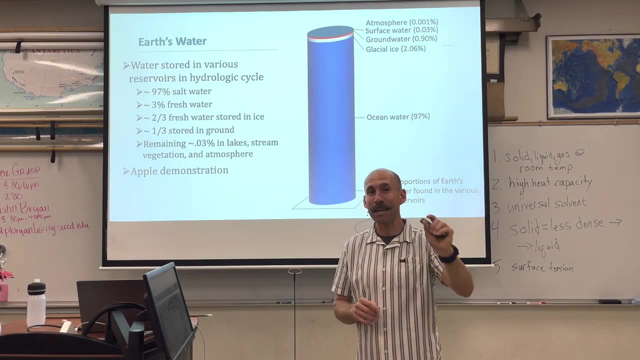 trapped in sea ice. it's all frozen in so inaccessible to humans for uh, potable and municipal consumptional uses. about one third of that- three percent, is stored in the ground, leaving very trace amounts left for people to use. now i have a great demonstration of this in the earth apple demonstration, please. 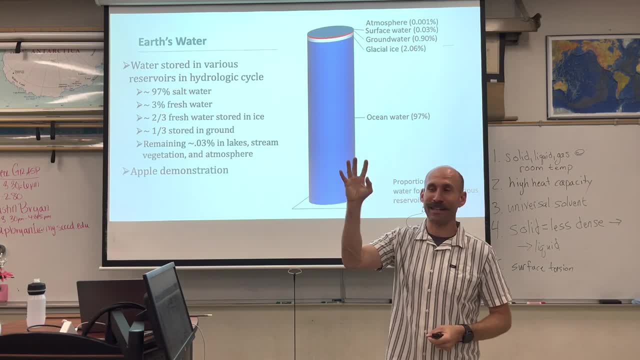 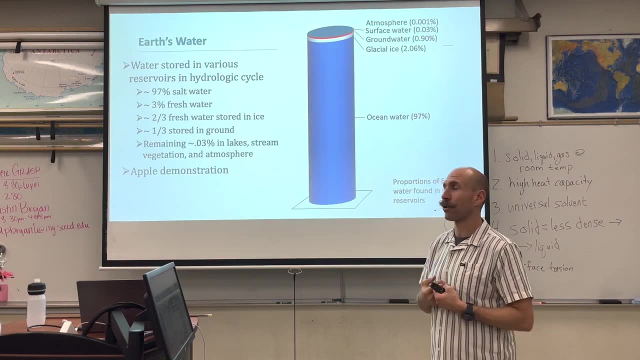 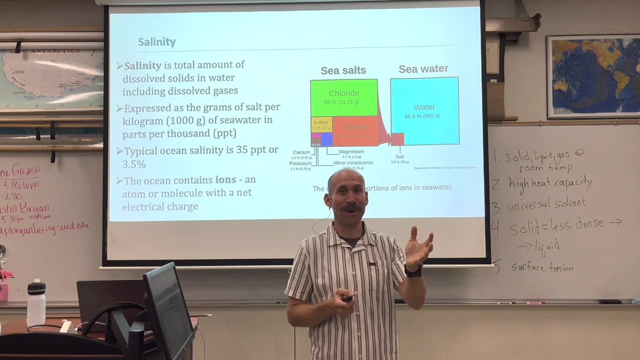 watch that video, check it out. it's going to blow your mind to think about how little water is actually available to humans to use as fresh water resources. okay, so we talked about how cool water is, its unique properties, where water came from and how it moves around the earth. 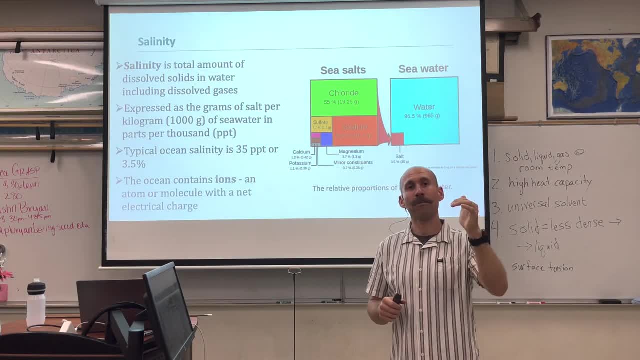 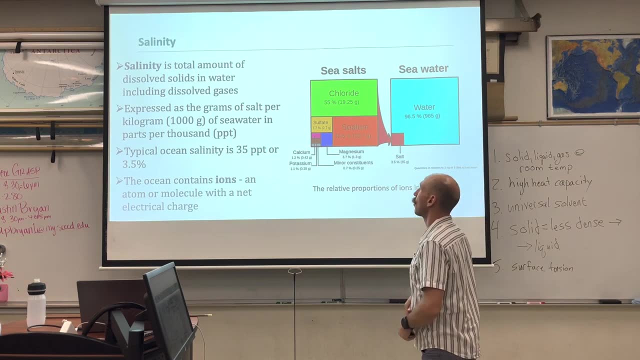 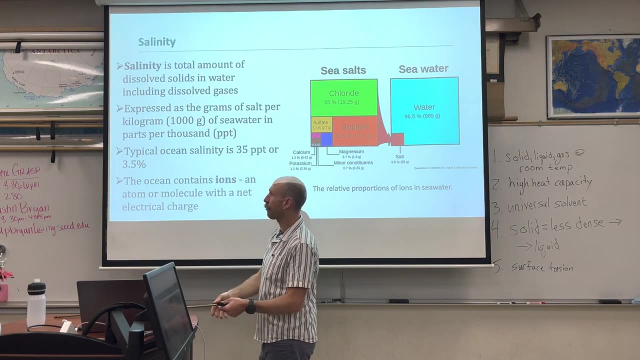 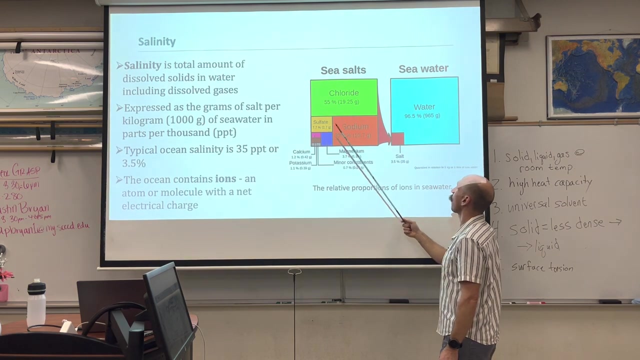 now let's talk about the salinity, the total amount of dissolved solids and dissolved gases that are located in water. so when we're thinking about salinity we can give it a percent. the average ocean salinity is about three and a half percent. we can also express it as a part per thousand, so ocean salinity is about 35 parts per thousand. 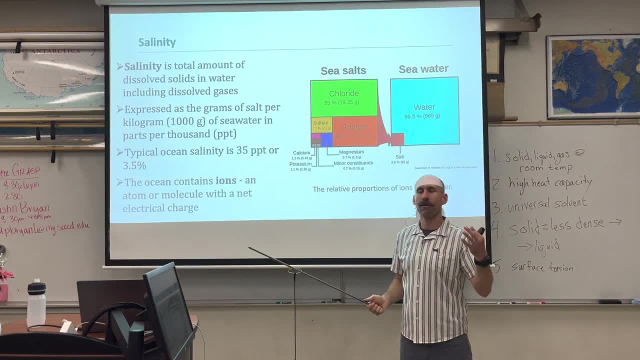 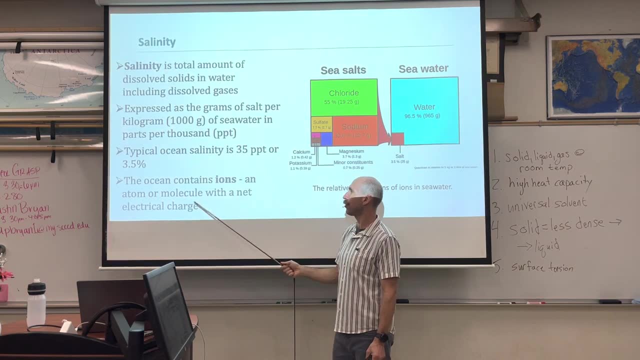 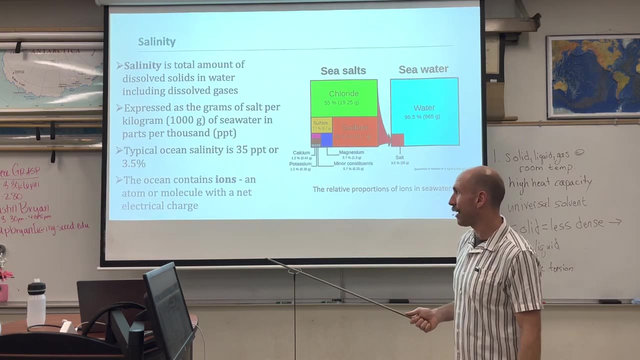 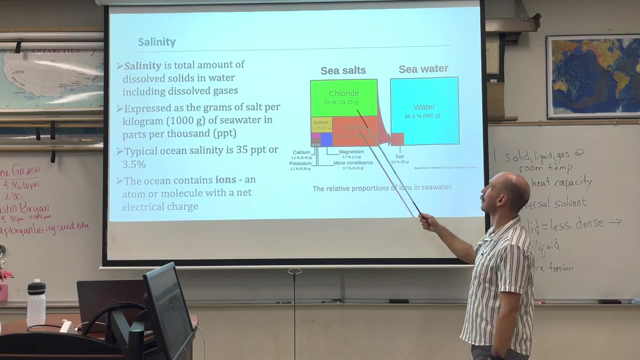 now we've been throwing these terms around: ions, compounds, molecules. what exactly are these things? well, the ocean has ions. an ion is an atom or molecule with the net electric charge. the water molecule is an ion because it is polar, it has electric charge. there's other ions in the ocean that are really important. the big six: chloride, sodium, sulfate, calcium, potassium and magnesium. three and a half percent of the ocean is dissolved solids and gases. of that three and a half percent we have big six dissolved ions: chloride, sodium, sulfate, calcium, potassium and magnesium- and we can see the relative proportions in the ocean of the big six. these are all conservative ions because 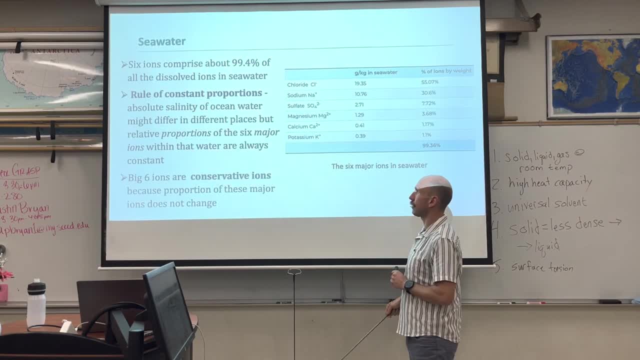 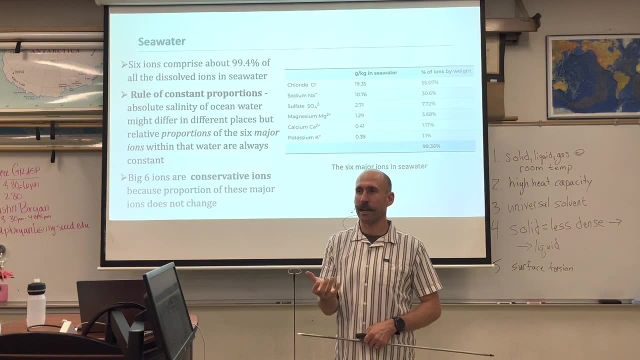 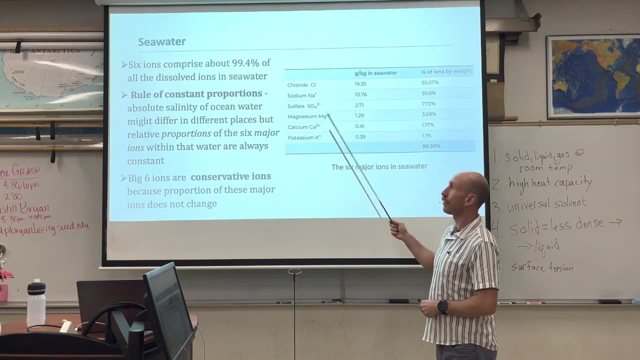 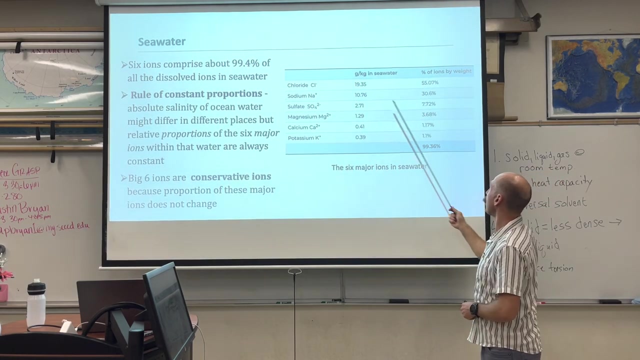 the proportion doesn't change. so it goes a little something like this: the rule of constant proportion states that if i have a sample of seawater that contains two percent salinity, in that two percent we will have 55 percent chloride, 30 percent sodium, seven percent sulfate, three percent magnesium, one percent calcium, one percent potassium. 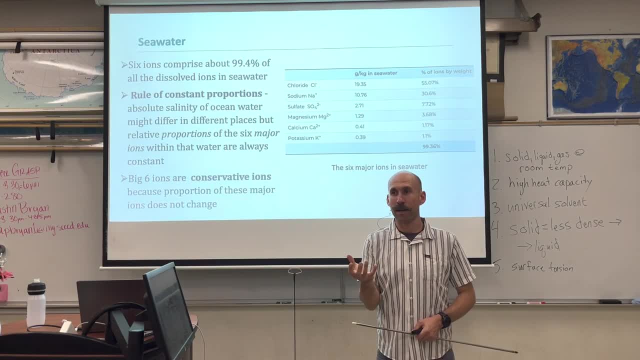 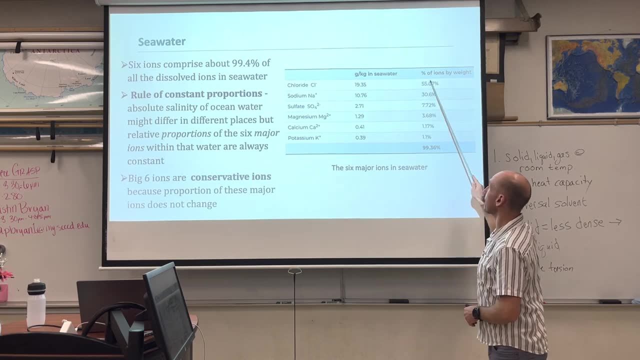 if i have a sample of ocean water that is five percent salinity. of that five percent salinity, fifty 55% will be chloride, 30% will be sodium, 7% will be sulfate 3, magnesium 1, calcium 1, potassium and so on. 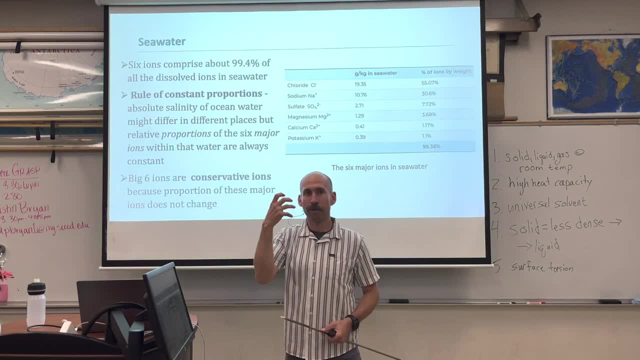 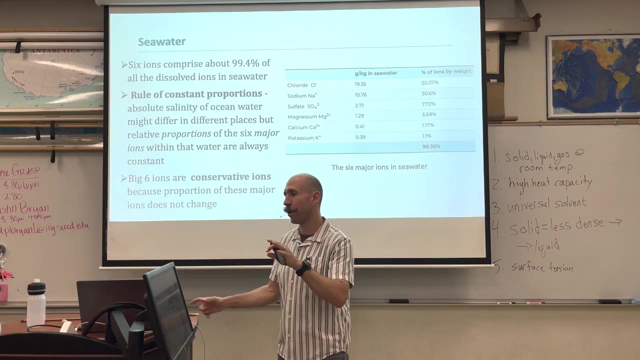 So what this says is that the proportion of the ions, of these six major ions in seawater, no matter what the salinity, are constant. They're always going to be the same: The proportion, the relative abundance of one relative to each other. 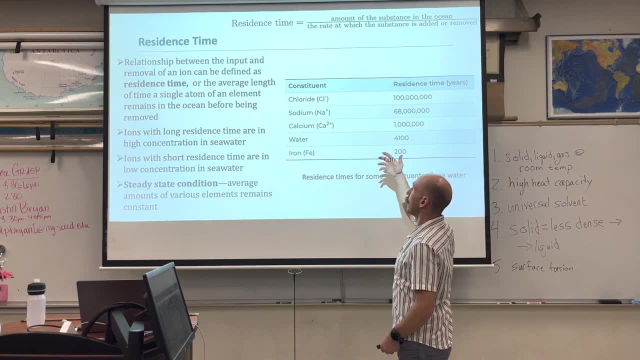 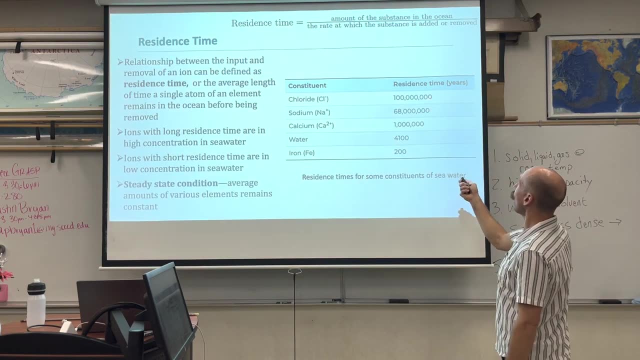 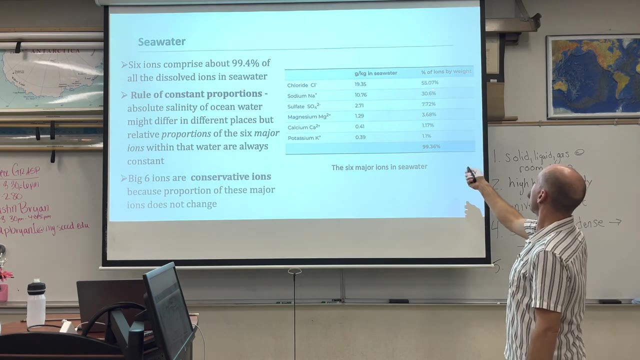 So let's think about the residence time, the length of time a single atom of an element remains in the ocean before it's removed, And so the residence time for chloride is 100 million years. That's a very long time. Chloride is, by far and large, the largest percent of ions by weight. 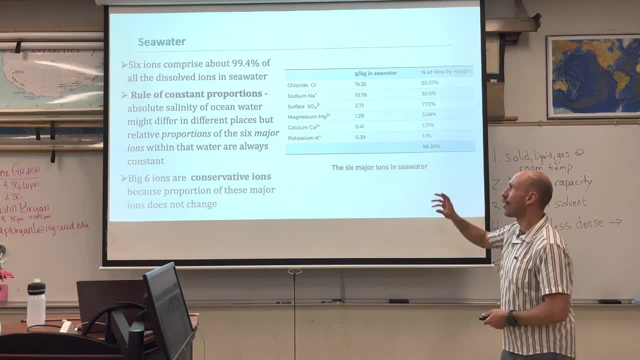 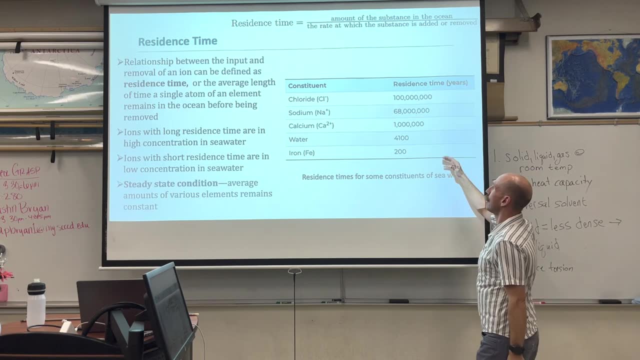 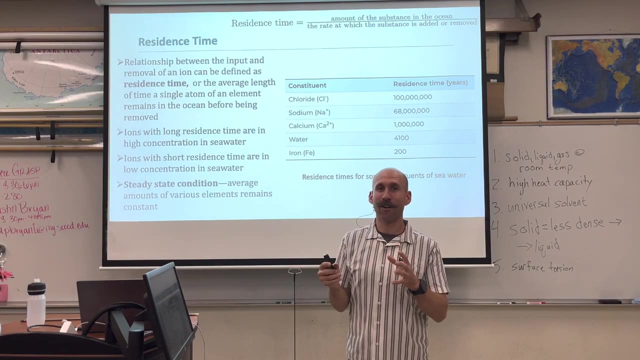 because it has the largest residence time. So residence time and relative abundance: sodium, 30% Sodium 68 million years, Calcium, so on and so forth. So what this does, having ions that have such long residence times, is it creates steady state conditions. 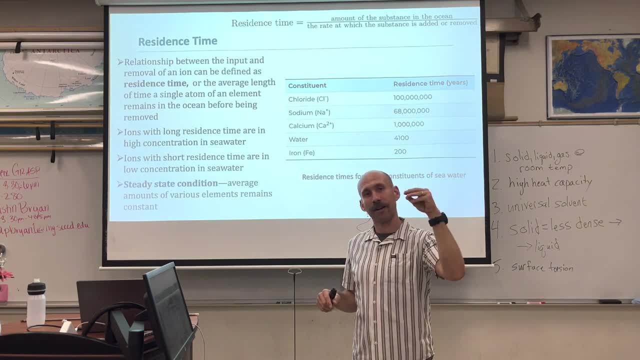 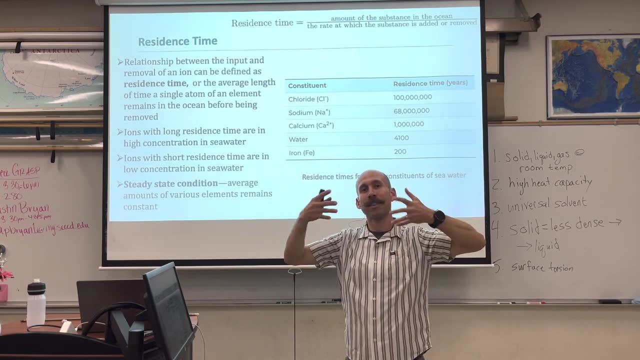 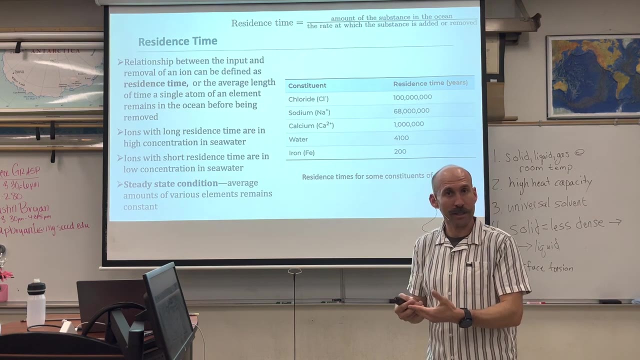 where the amount coming in of ions that are entering and the amount of ions that are exiting are equally balanced with the length of time that the ions can remain in the ocean. What's happening here is there's only aidad of ions that are coming in. 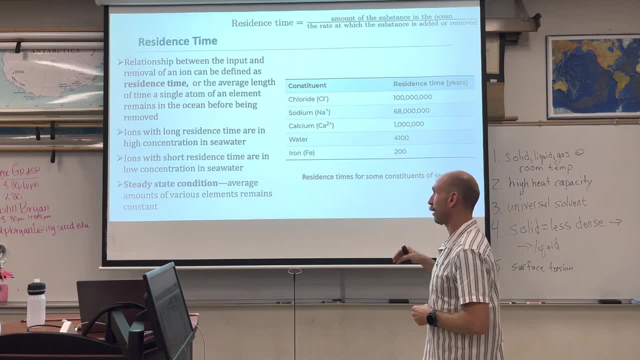 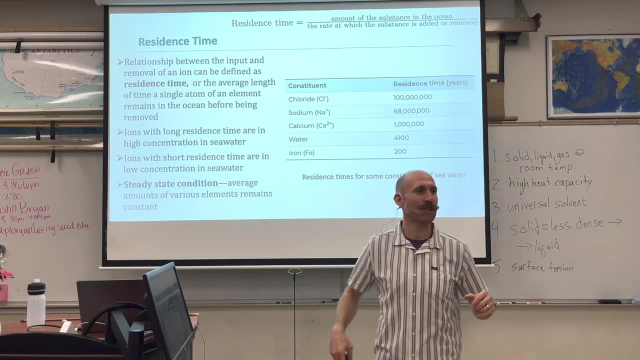 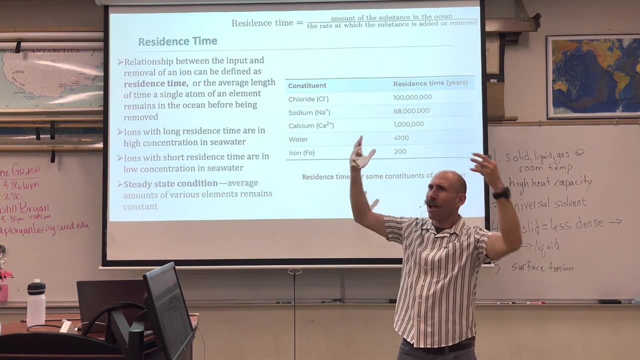 and they're everywhere. I had already talked to some people who have crazy momentum which allowed us to know that the speed of evolution has no reaction to occurred. So we've actually created some so-called medicines to give us these relatively proportional constants and also 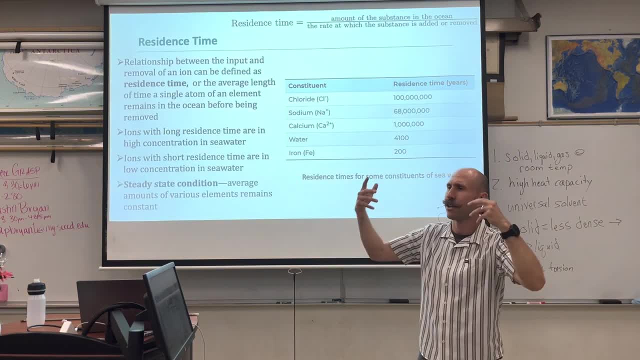 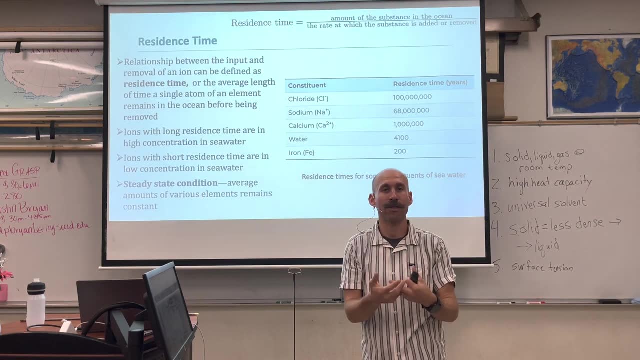 volcanoes and- thank you- arrival of comets and uh. through this we will precipitate oceans and they will have dissolved solids in them and the the relative proportions of dissolved solids has remained pretty stable over the past billions of years, as we can see identified in the rock. 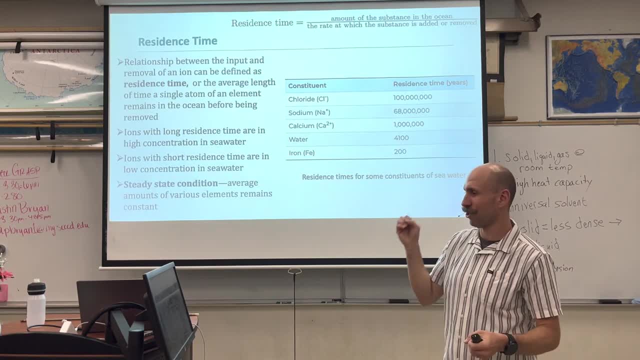 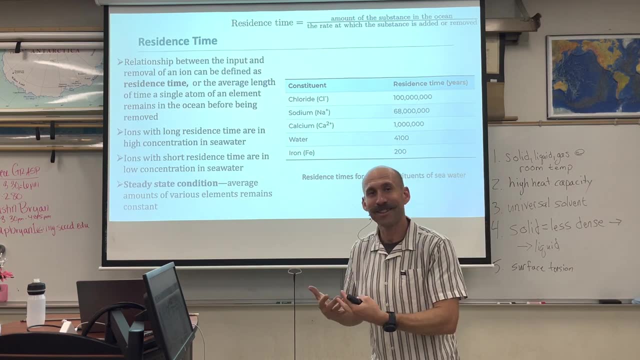 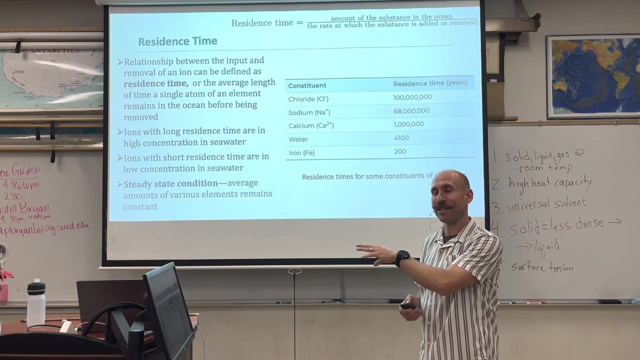 record. because rocks- yeah, what is this? just some stupid rock. oh, don't say that rocks are really, really important, because rocks are like the earth's history pages. they tell us what's happened in the past. they tell us about the salinity of the oceans in earth's history. but 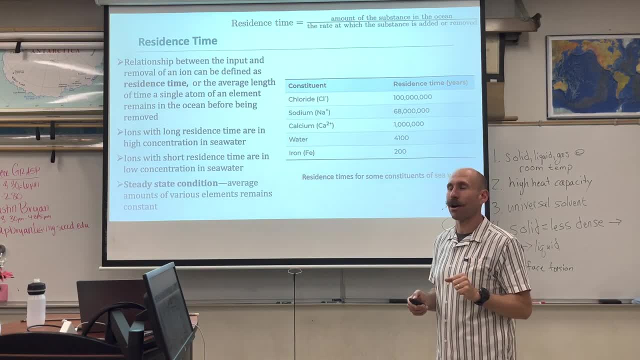 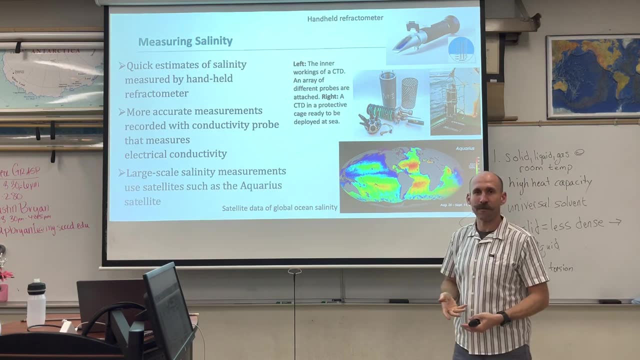 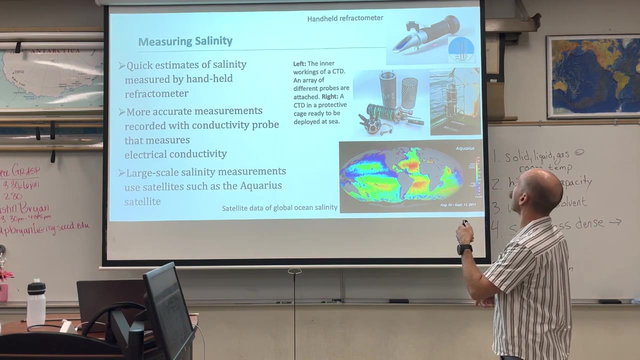 let's not get too excited about geology, because we're excited about oceanography, and let's keep this going. there's ways of recording and measuring and observing. our technology is great, and so measuring salinity can be done by hand from a handheld refractometer. 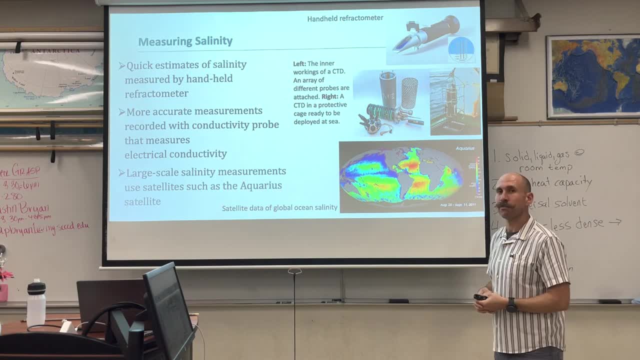 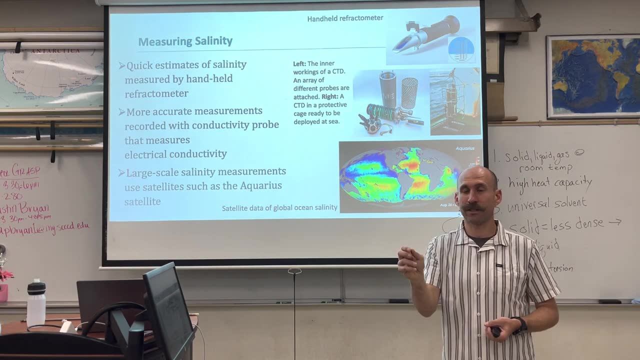 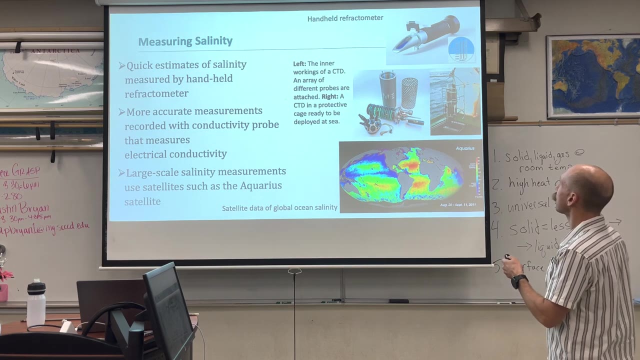 this is quick, it's not the most precise, but it can give us an idea of um point. observations, specific point in the ocean boom measure- that's what it is more accurate- are going to be with the conductivity probe that's going to measure the electric potential that will. 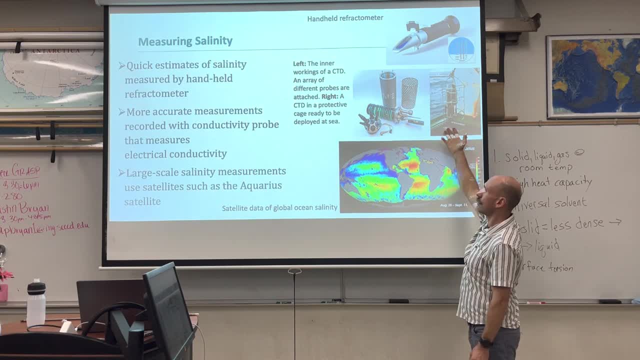 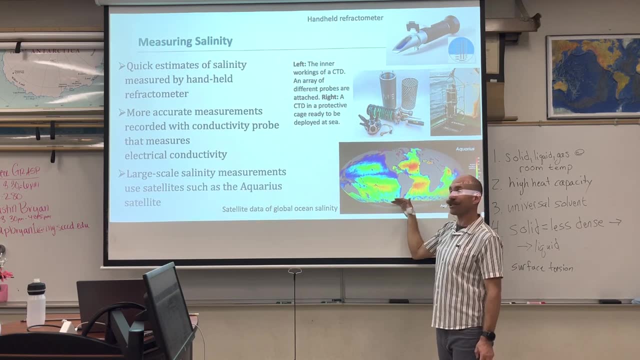 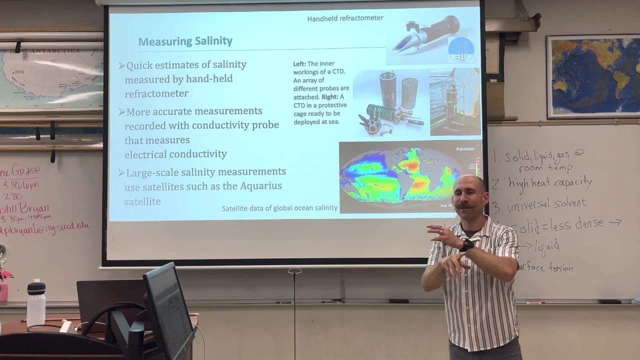 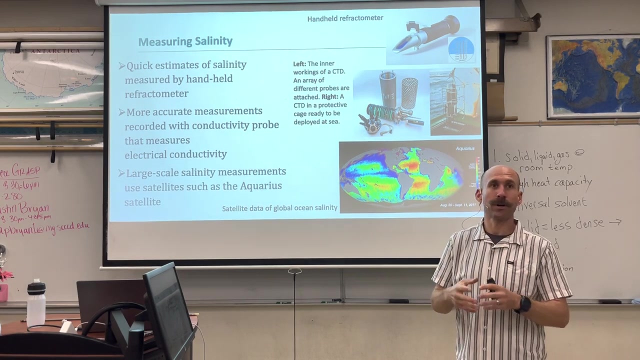 give us a surrogate for the dissolved solids. we've also got large scale salinity measurements using satellites. so cool. satellites are amazing. they're all over the earth, uh, swooping around recording all kinds of data and incredibly valuable for our understanding of how earth systems work on a very global scale. so where did this original salinity of the oceans come from? well, it happens from the water vapor. the oceans have always been about as salty as they are now, and the balance remains the same. through the entry of runoff, volcanic activity and hydrothermal vents, ions can be. 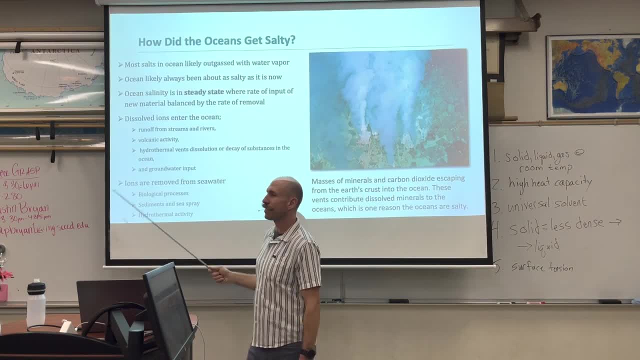 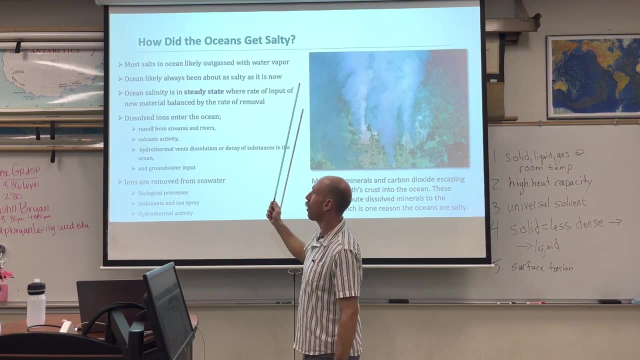 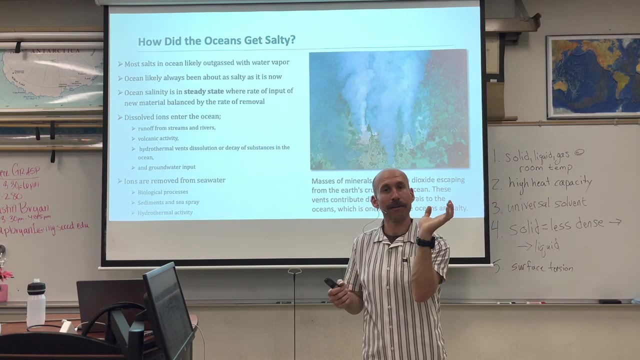 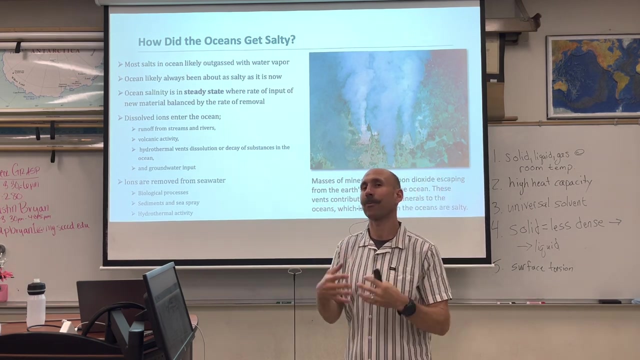 removed through biological processes, sediments and sea spray and then hydrothermal activity. so we've got a whole variety of processes, but again it's basically ions come in and ions enter and they are balanced. so one of the big ways they enter is the silicate weathering system, which basically is when it rains on land, it erodes rocks. 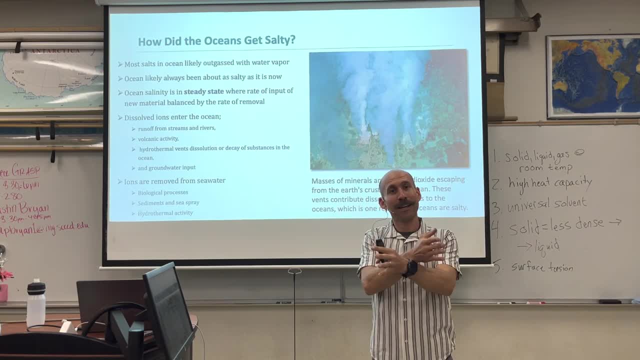 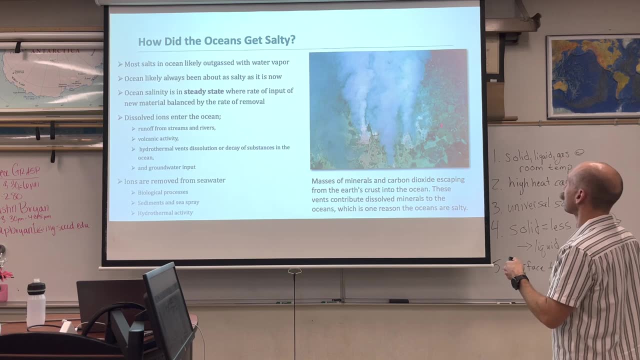 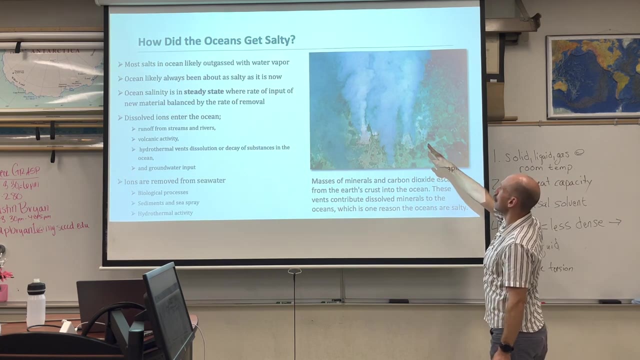 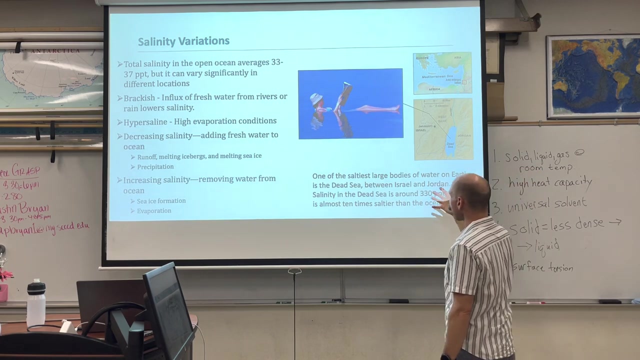 the rocks break down and are transported through rivers, delivered to the oceans. underneath at the surface, at mid-ocean ridges, we have black smokers and they are very highly Ulsterly, but we have these minerals in the air, from where minerals in earth's crust are released into the ocean by dissolving through these superheated. 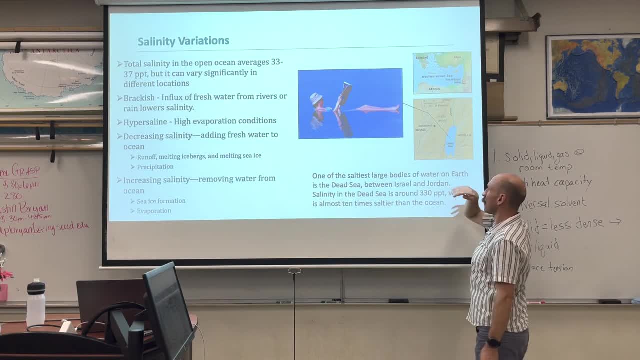 cracks in earth's crust- really amazing process. i've talked about it before. we'll go in depth even more so. salinity can vary all the way to hypersaline the dead sea. please see video of the dead sea where you have an order of magnitude of this Duluthi and Hurts водλ. 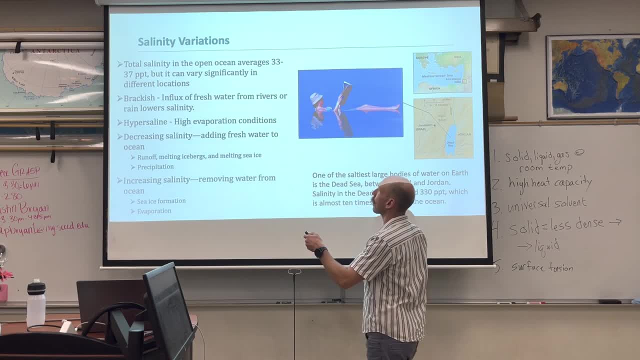 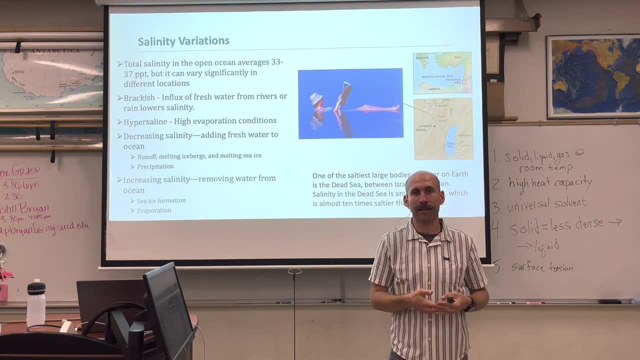 the higher concentration of salinity into brackish waters And what are the processes that could create more saline, hyper saline or less saline? Input of fresh water basically will dilute, Temperature can change and that can really lead to the amount of evaporation. 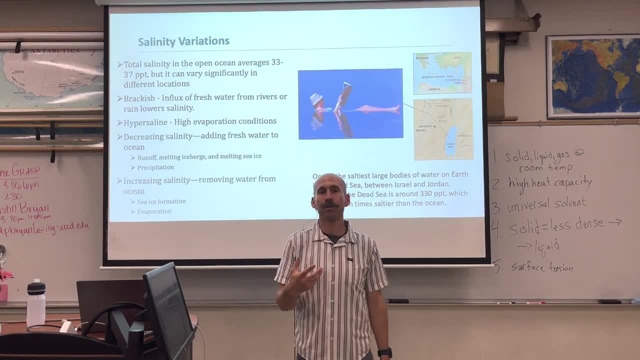 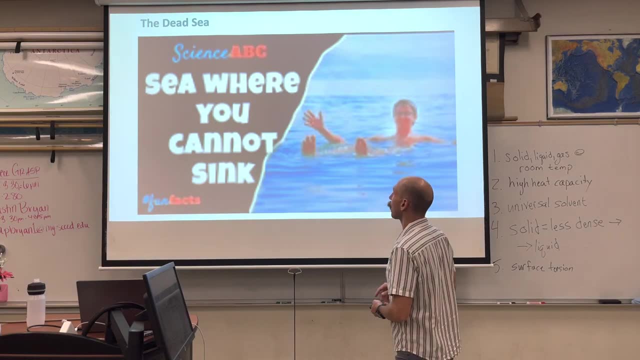 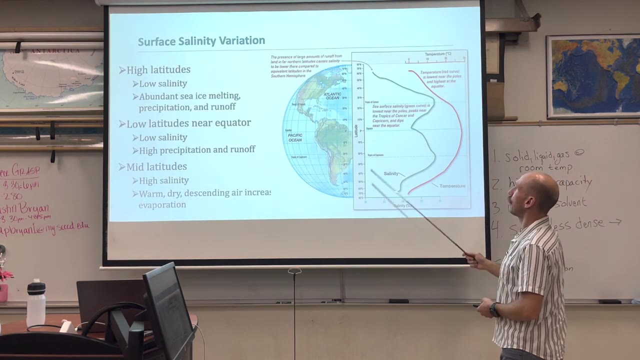 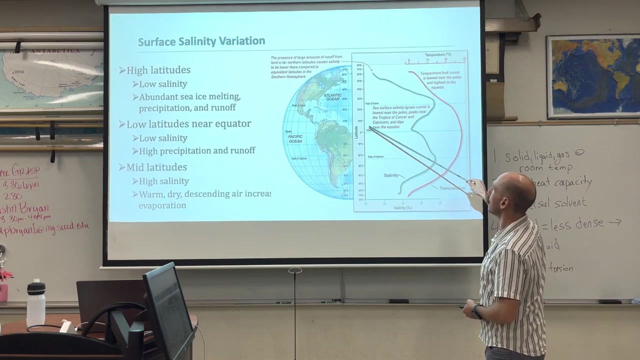 or precipitation And temperature can also contribute to the development of sea ice or the melting of sea ice. So here's our video. Please be sure you check this in the video section. This is the earth: Latitude, zero degrees, the equator. 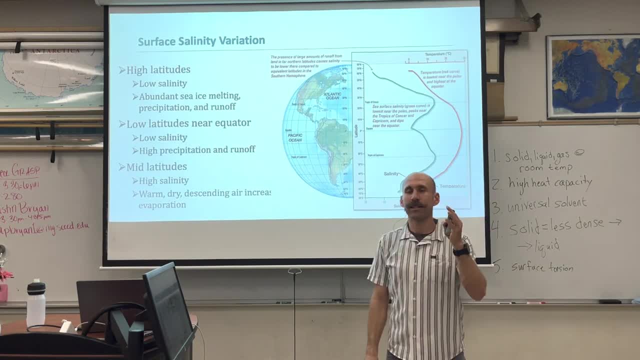 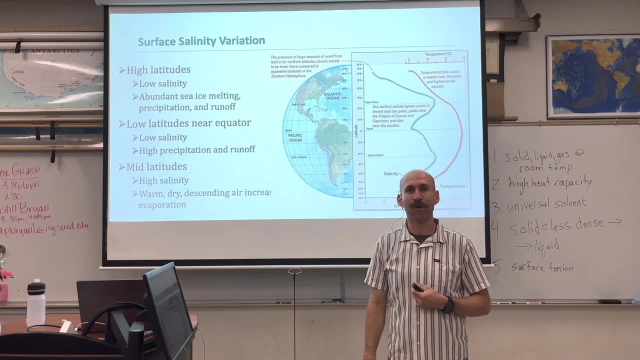 90 degrees south and north. So let's think about this: Is it hot or cold at the equator? It's hot, yes. Is it hot or cold at the poles? It's cold. okay, Intuitively, we know this. 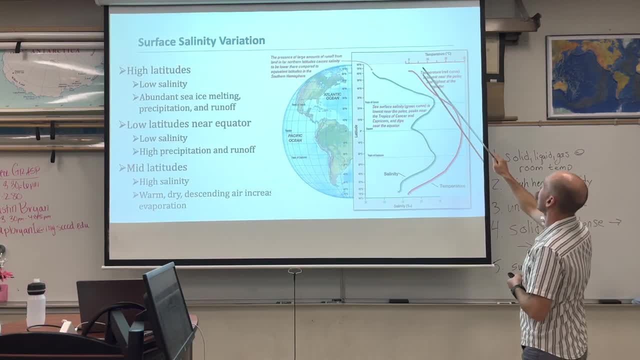 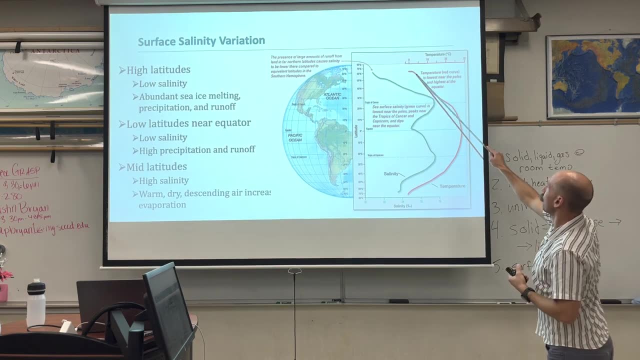 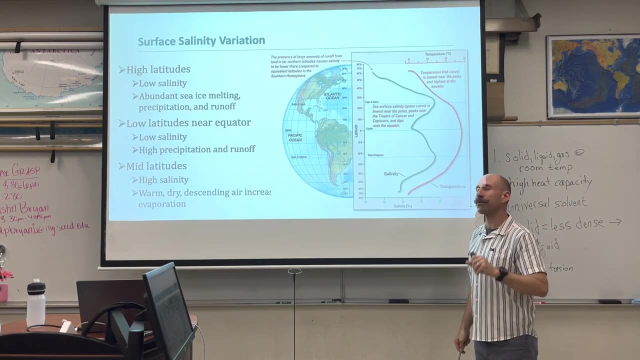 So red line temperature: cold at the poles, hottest at the equator, cold at the south pole. So north pole, equator, south pole. Now salinity varies, with latitude also, but a little bit differently. The equator is hotter. 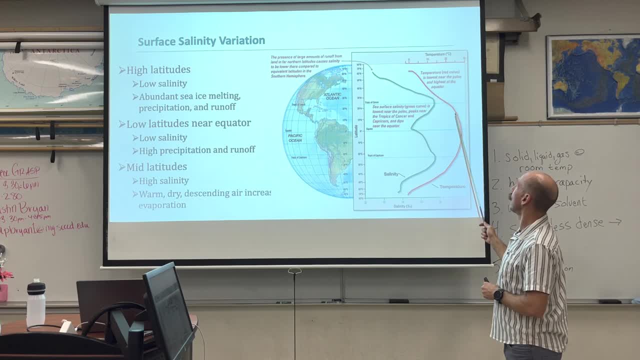 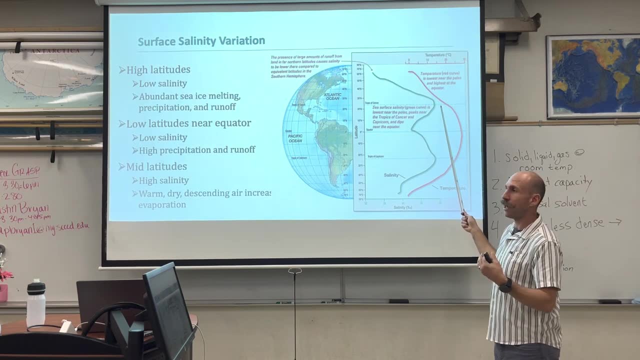 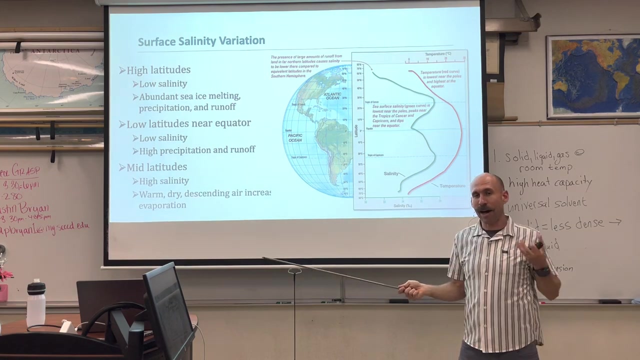 but when that's hot there's a lot of precipitation. The tropics are dry. This has to do with atmospheric circulation hadley cells. We'll talk about that in our ocean circulation chapter. Really great stuff. I love this topic. but the tropics are dry. There's a lot of evaporation We talked about on the last slide. if we pull water out, it increases salinity and if we put water in it decreases. So it's like putting water in and decreasing. 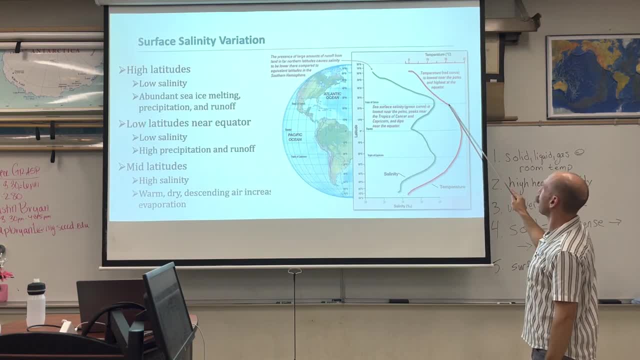 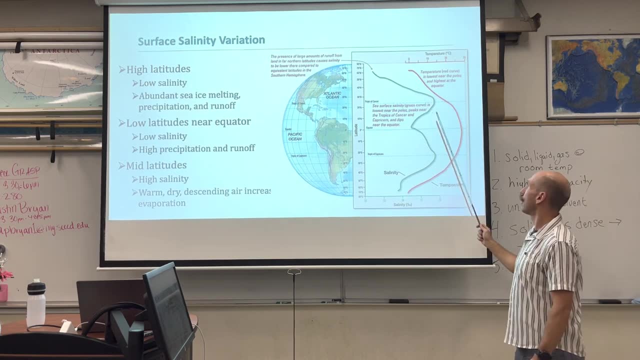 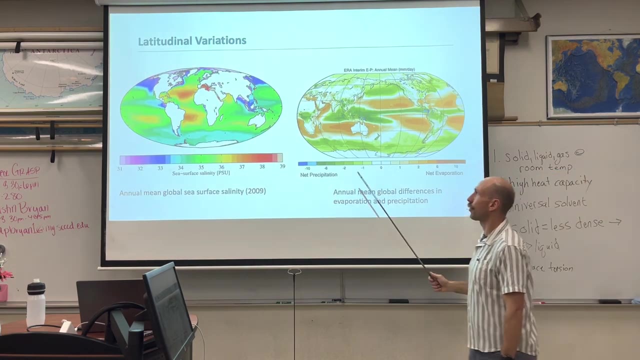 So rainy decrease, Evaporation increase. We get this double hump of salinity where the maximum salinity, the highest salinity, is going to be at the mid-latitudes, specifically around the tropics. So here we get latitudinal variability. 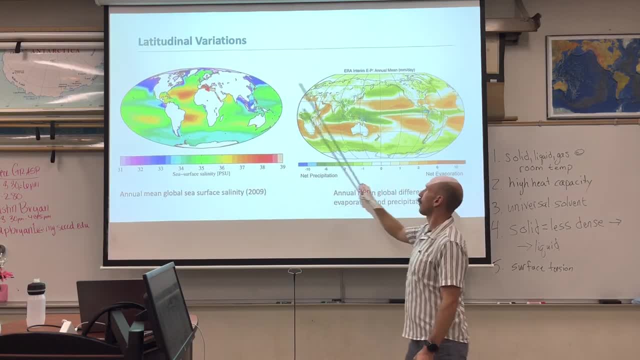 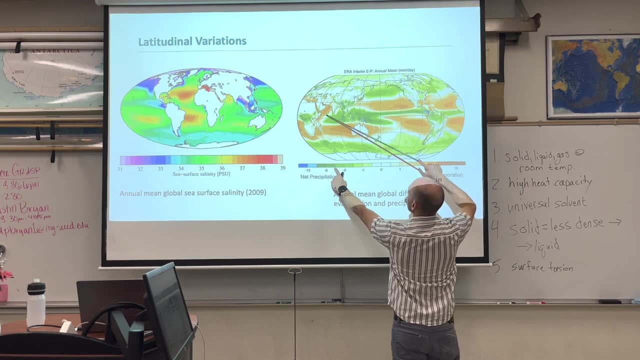 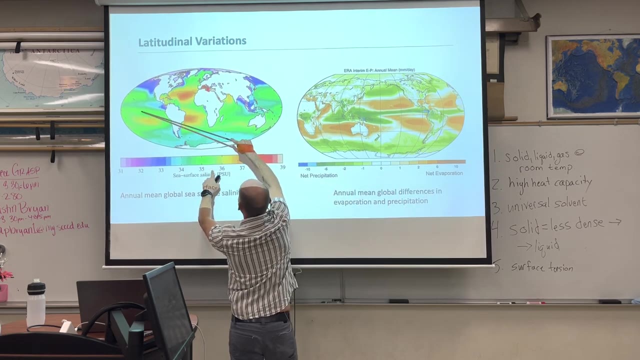 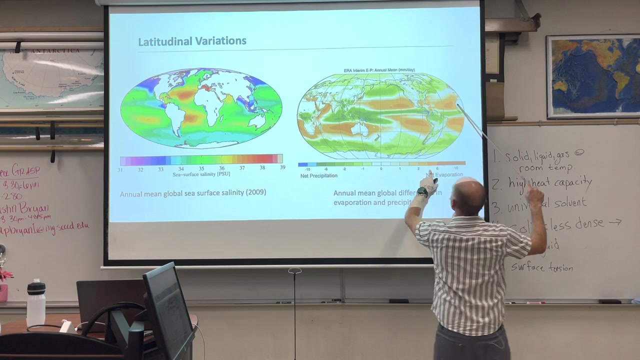 We have global sea surface salinity and we have net precipitation. Now green is high net precipitation around the equator. Take this over to a little bit lower salinity: mid-range here. Now net evaporation right here, tropic. 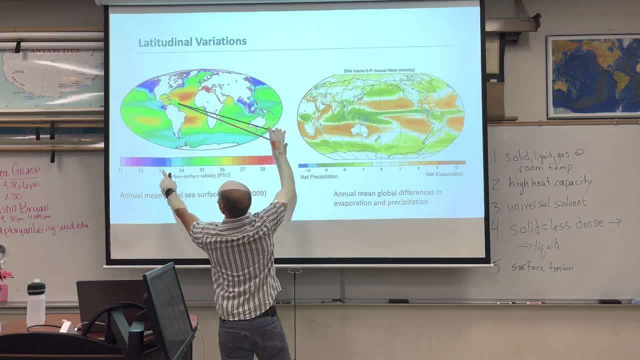 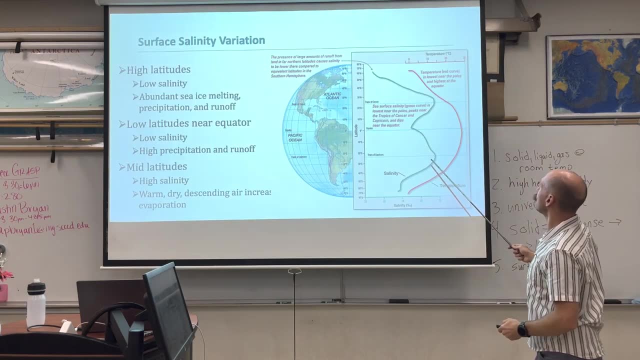 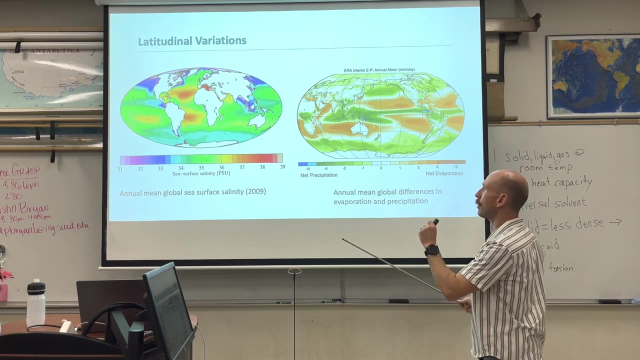 Take this over. We're going to have lower salinities here And here. So again, what do we see? We see the salinity at the tropics a little bit higher. I think I misspoke. Let me do this one more time. 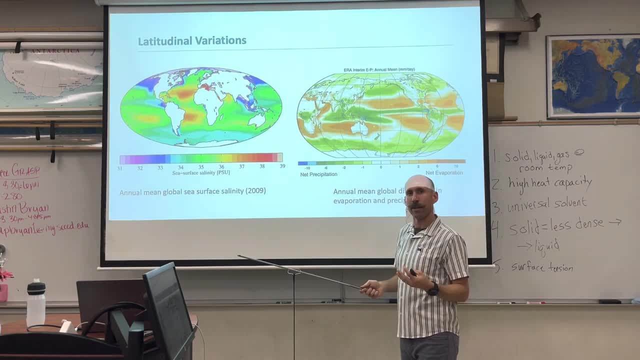 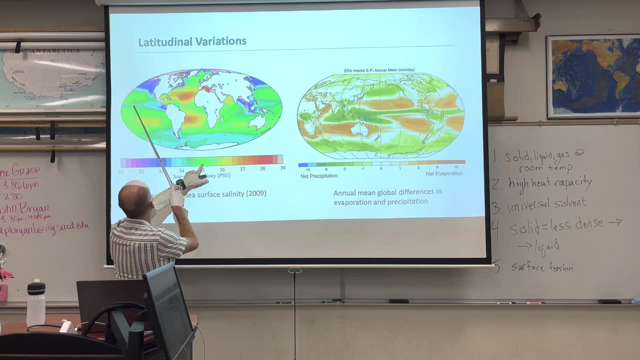 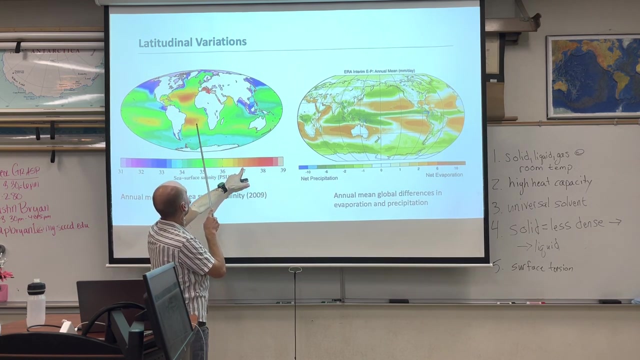 Higher precipitation at the equator. right, So the equator is hot, There's higher precipitation. Now here we go. So salinity right around 35 through here. So our salinity: 35 at the equator. Now let's go down here to the tropic: 37,, 38. 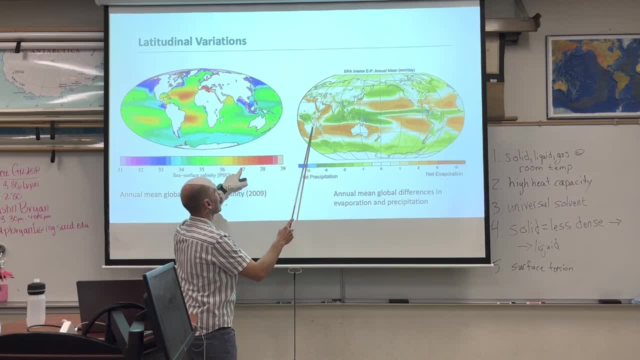 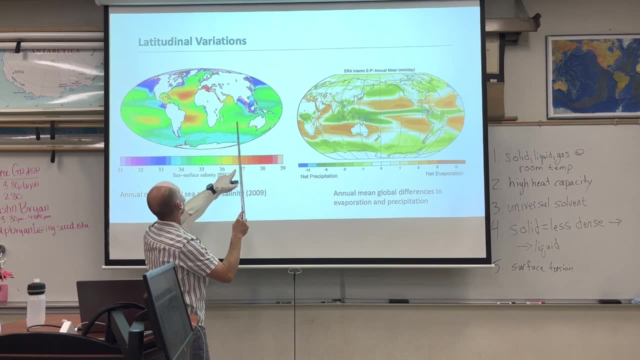 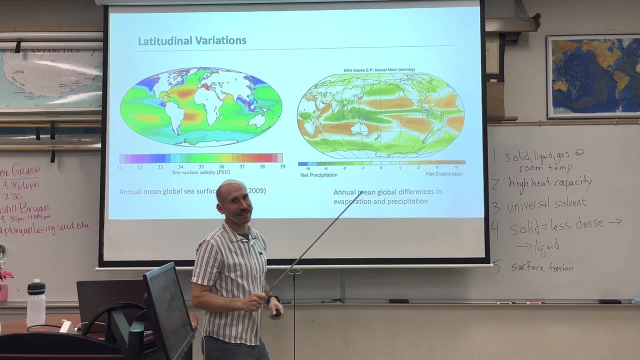 This is where there's net evaporation. So what these two graphs show us is that where there's net evaporation, we have higher salinities. Where there's net precipitation, we have lower salinities. So there you have it. 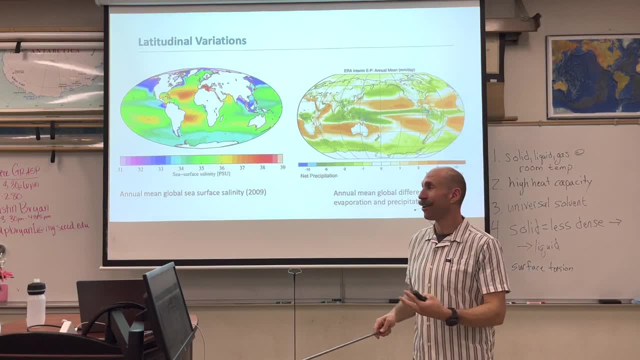 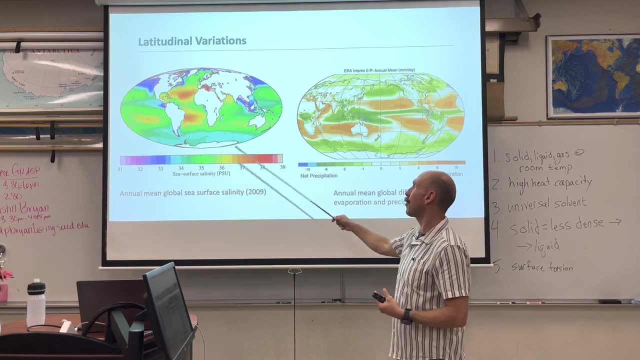 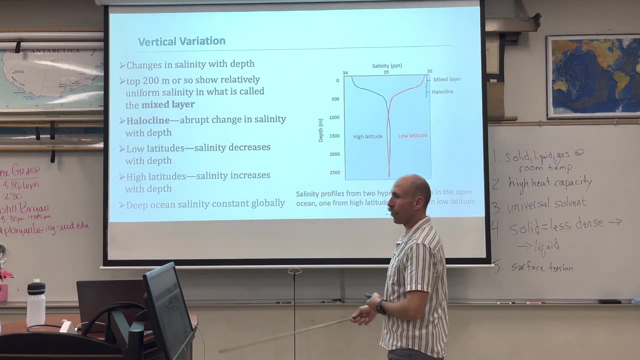 Not only do we understand this process, but we can observe this phenomenon by recording measurements of both sea surface salinity and global precipitation and evaporation differences. So this isn't the only way that salinity varies, It also varies by depth. So we just said in that last discussion. high latitudes have lower salinity than low latitudes. High latitudes have lower salinity than low latitudes. These are the low. These are the high. Now there's a mixing layer in the upper 200 meters of the ocean. And then below that we have what's called a halo line. This is an abrupt change with salinity at depth, where high latitudes increase, Low latitudes decrease And then they line up for a deep ocean salinity that is globally constant. 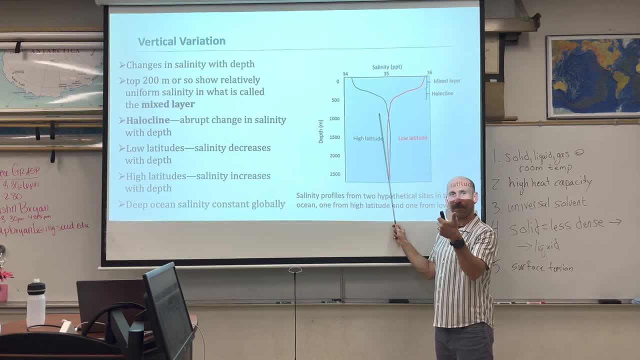 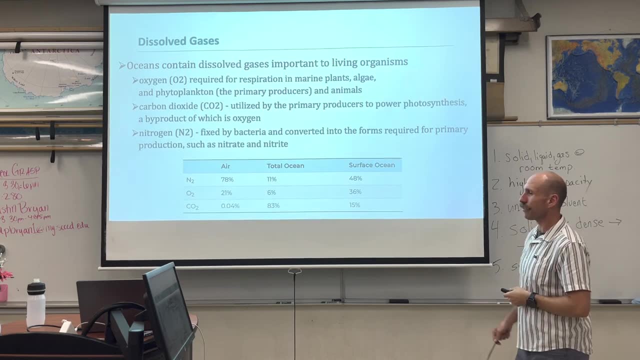 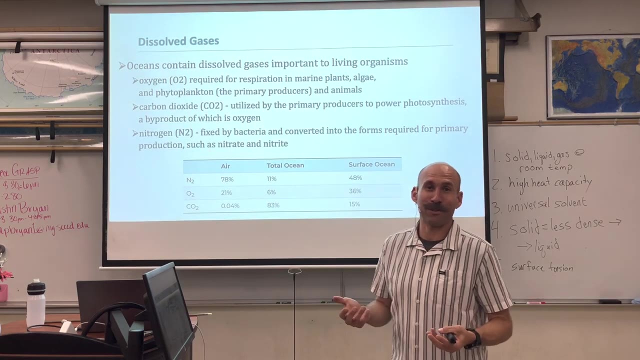 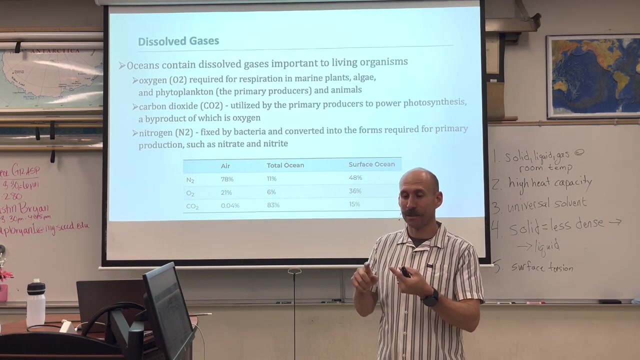 Cool stuff here. So we've got latitudinal variation and variation with depth. This takes us into our next discussion of how cool oceanography, the chemistry of the ocean and the chemistry of the ocean are oceans are. so not only do is there dissolved solids, but there's also dissolved gases, specifically, 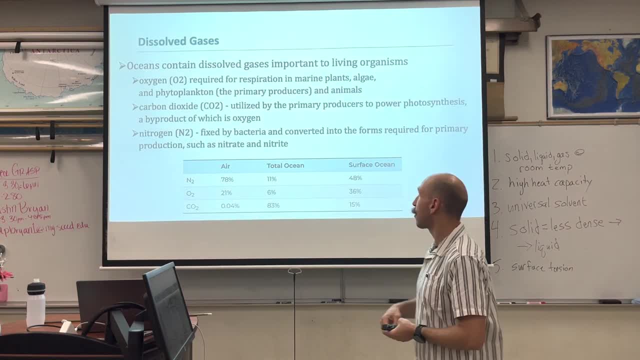 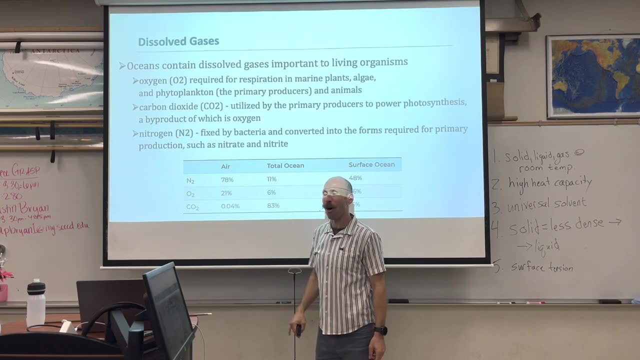 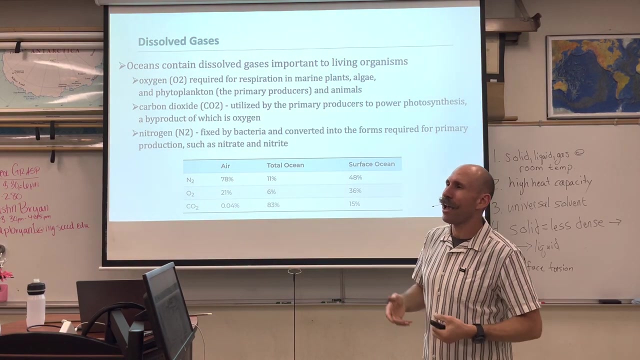 oxygen, nitrogen and carbon. and when we think about this, what's the atmosphere? 78 nitrogen, 21 oxygen, 0.04 carbon. where are the dissolved gases in the ocean that are important for life- nitrogen, oxygen and carbon? it's like somehow the earth thought: hey, if i'm going to evolve and i'm 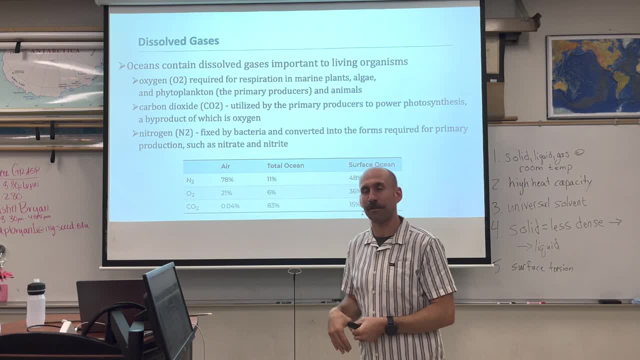 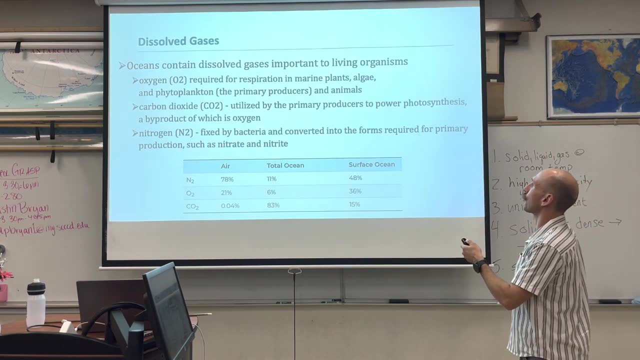 going to evolve life. let's just use the materials that are available and that's exactly what we see. so oxygen is really important for the respiration of marine plants, algae and phytoplankton, and animals. carbon dioxide is used by primary producers to power photosynthesis. nitrogen is a primary 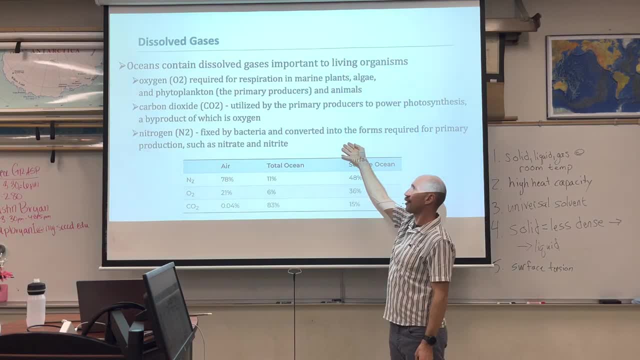 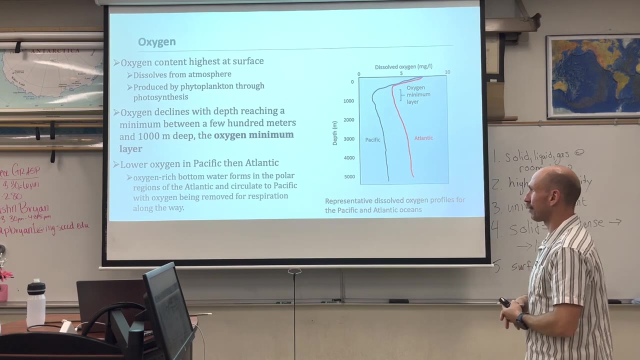 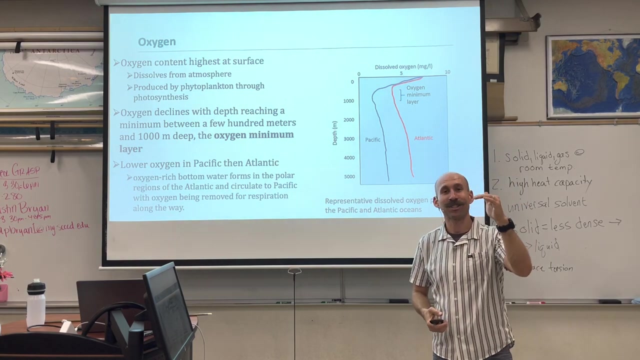 production is a nutrient that is required for primary production also. so not only is there oxygen, nitrogen carbon in the atmosphere, it's in the oceans and it's in the biology, it's in the life of marine and terrestrial organisms. so let's talk about oxygen. oxygen content is highest at the 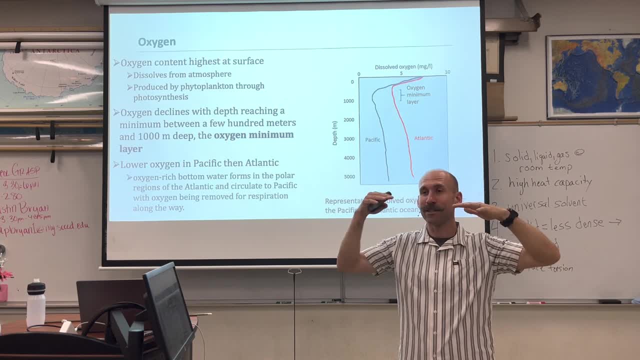 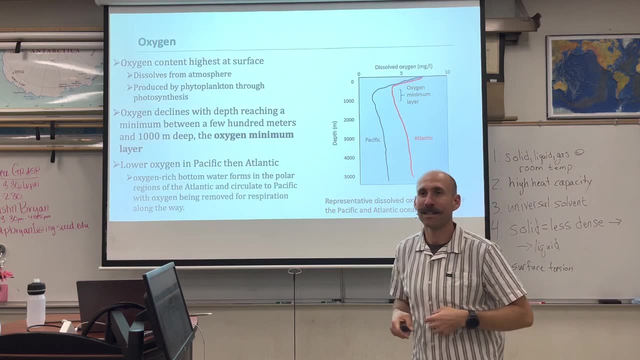 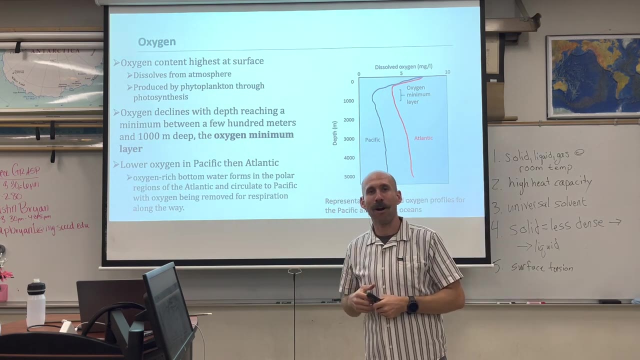 surface. this has to do with the organisms, with photosynthetic organisms that need light to survive. right the process of photosynthesis: a little bit of light, a little bit of carbon, a little bit of water. next thing you know you have oxygen. so, okay, we've got oxygen that comes from dissolved, that dissolves from the atmosphere. we've got oxygen produced by phytoplankton through photosynthesis. there's an minimum layer where there's the minimum amount of oxygen and then it stays pretty constant at depth and it's pretty low. if we go to this graph of dissolved. 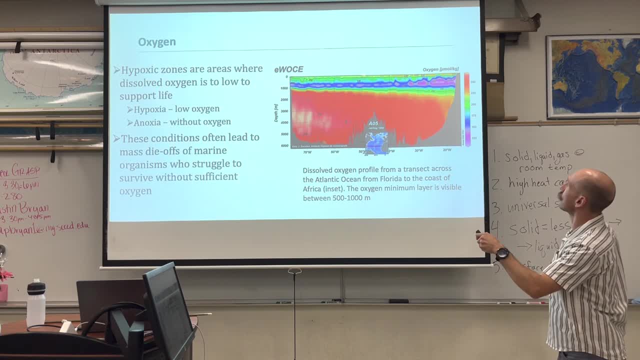 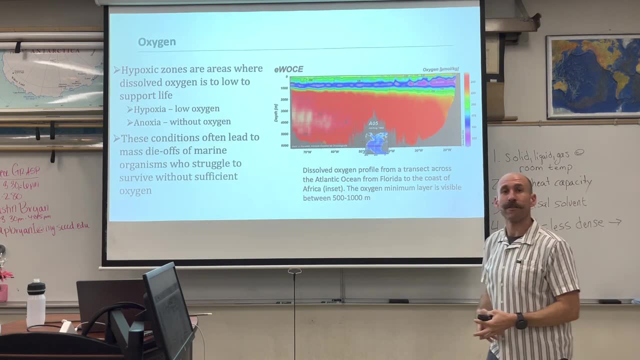 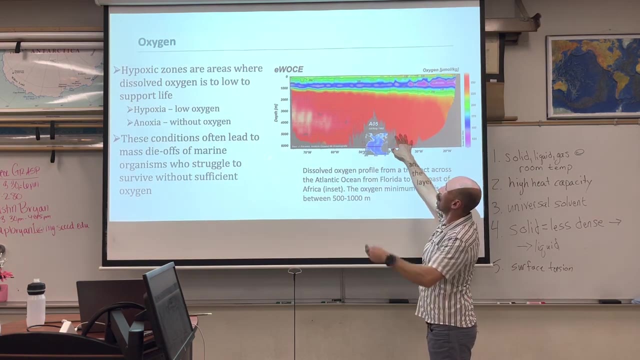 oxygen right varying. we can see that oxygen is highest in that upper reach, the upper kilometer. this is also known as the photic zone, the area where light can penetrate down into the oceans and it decreases. there's much more life, especially life that needs oxygen, in the shallow surface of the ocean than at 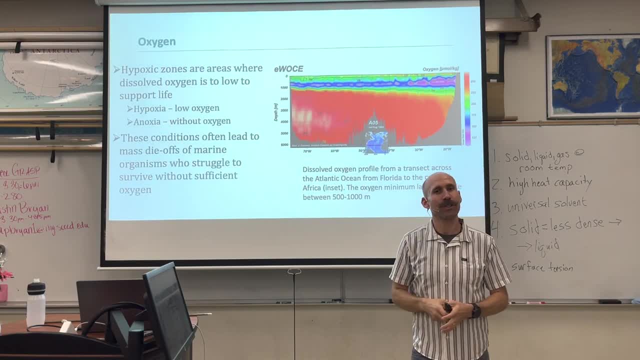 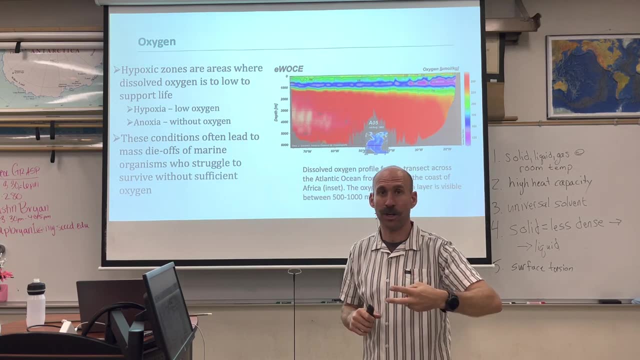 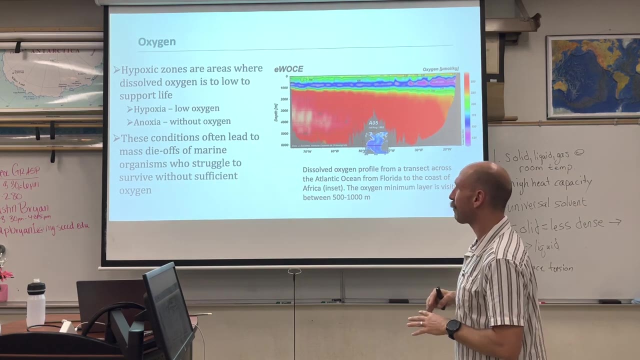 depth. if there isn't enough oxygen, then it creates conditions- hypoxia, low oxygen, anoxia, no oxygen- and if we have these hypoxic conditions, it can lead to mass dialysis, which is no good for anybody. it creates dehydration and it can lead to mass dialysis, which is no good for anybody. 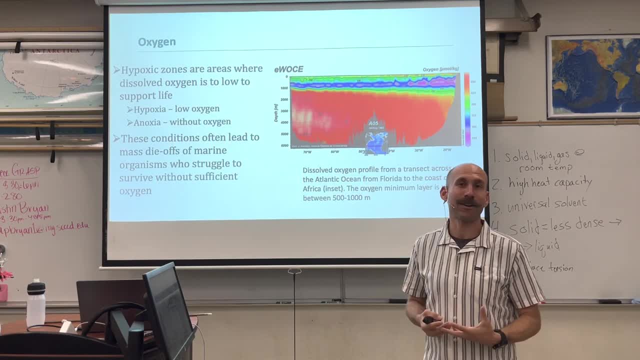 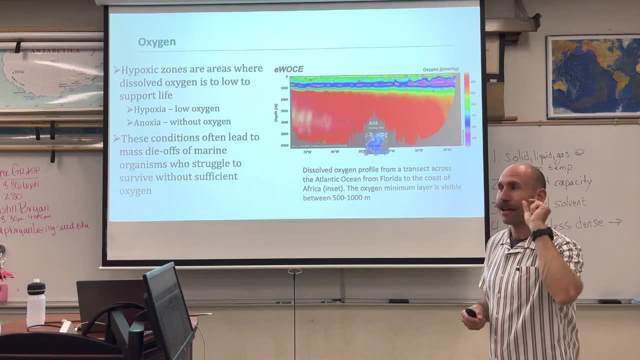 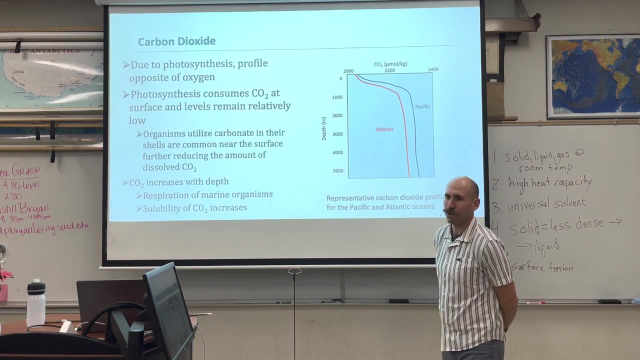 dead zones in the oceans. we'll talk about them. not good, we want to avoid them. they're environmental catastrophes that we can actively mitigate through our own actions. okay, so oxygen is important. different organisms need it. carbon dioxide is important in so many ways, so there is low amounts of carbon lower. 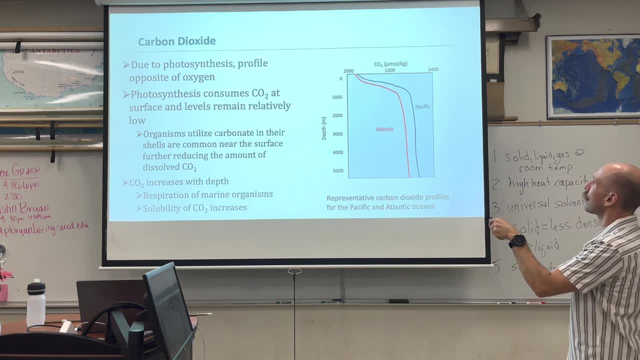 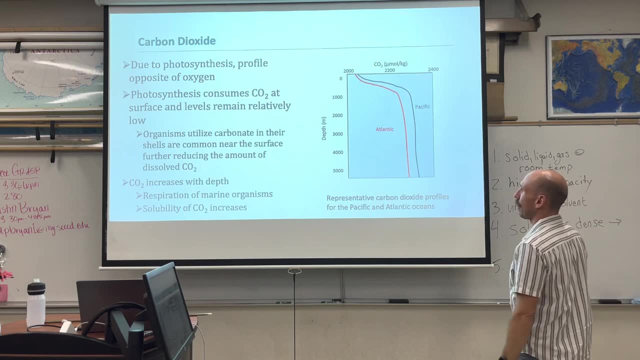 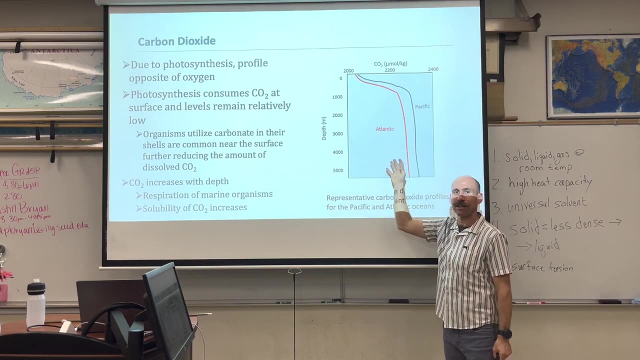 uh, in the surface. but then photosynthesis consumes that co2. right, that's why it's lower at the surface and it increases with depth. okay, there's respiration of marine organisms, there is an increased solubility of co2, the relative distribution and proportions of carbon in the 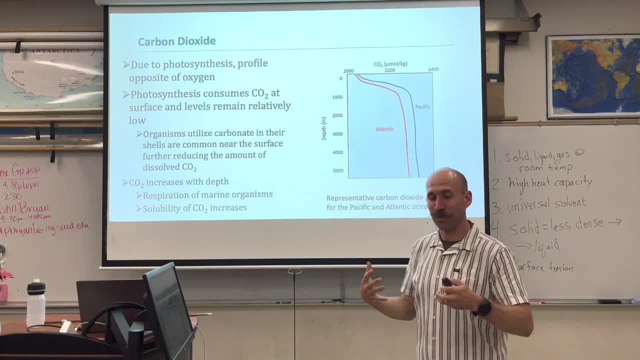 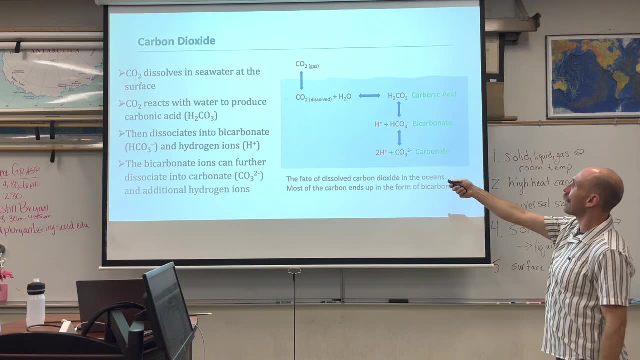 oceans, but carbon has a much bigger story. it's way more exciting than this. so it's just like this. if we're thinking about this model of lava, we often think about waters, and so here's an example of a lot of oceanетровan ocean disconnections. 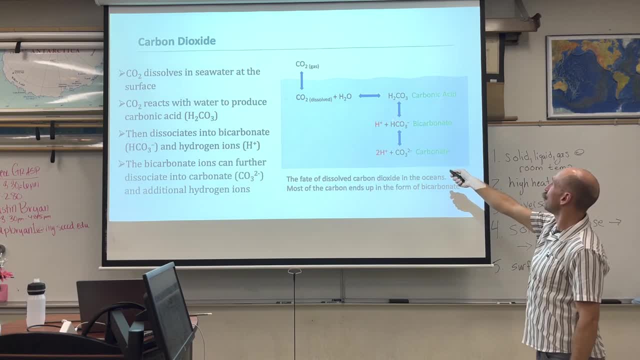 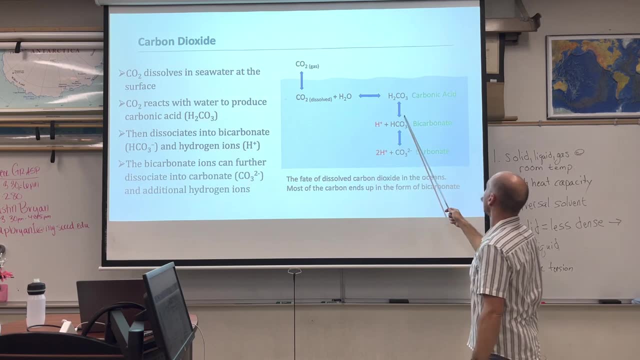 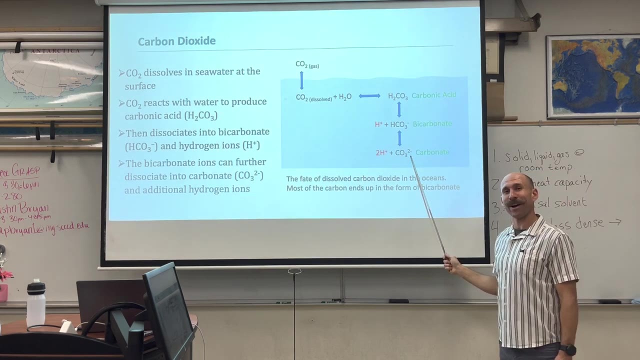 loudly. there's even this realRe них hier persecuted. and this is the one that we're able to get fromurai river or ocean tankers. these are the two SAM 알았어. but then there are all these rescued environments. here we getulse water which may be a pretty 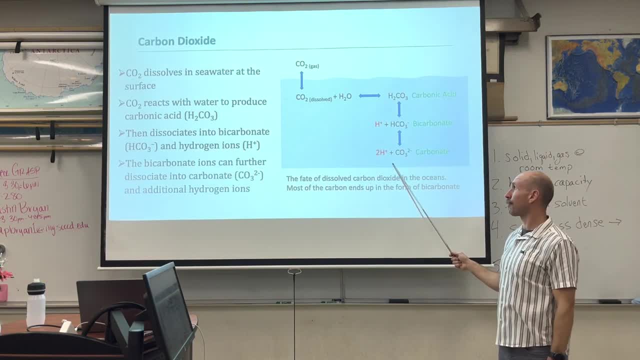 useful. so it's in the middle classes, because if you're looking at socaldeok, and very vibrant or a reservoir for the biogeochemical cycle of carbon, it can also produce two hydrogen ions, So most carbon in the oceans ends up as bicarbonate. 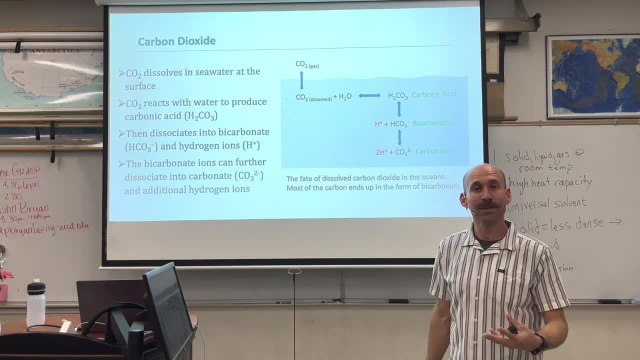 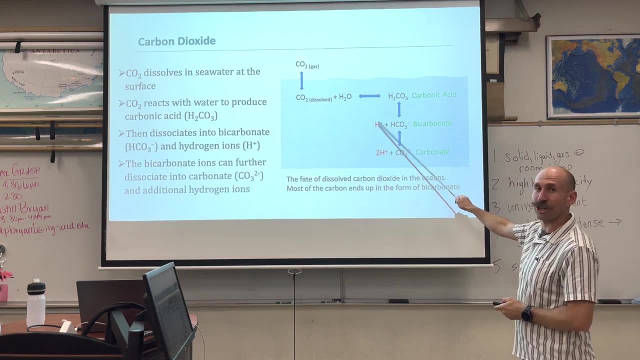 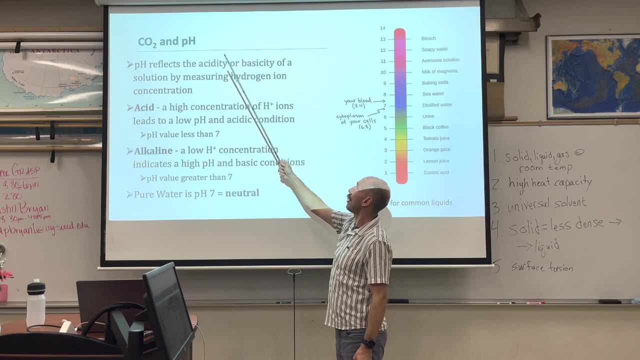 This bicarbonate is taken up in the shells of marine organisms, both macroscopic and microscopic. Now the proportion of hydrogen ions that's left over. this is going to affect the pH, which is measuring the hydrogen ion concentration. If it's below seven, it's acidic. 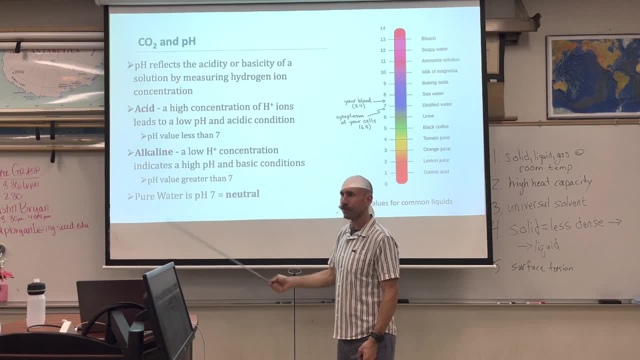 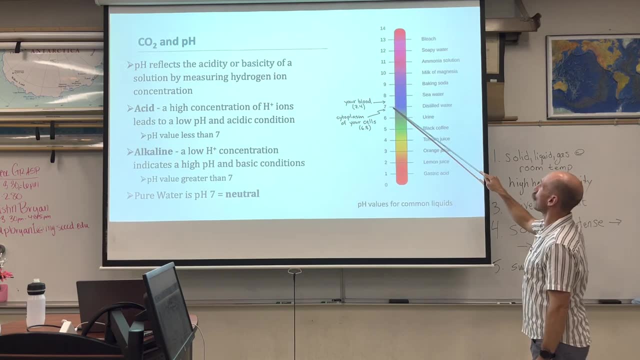 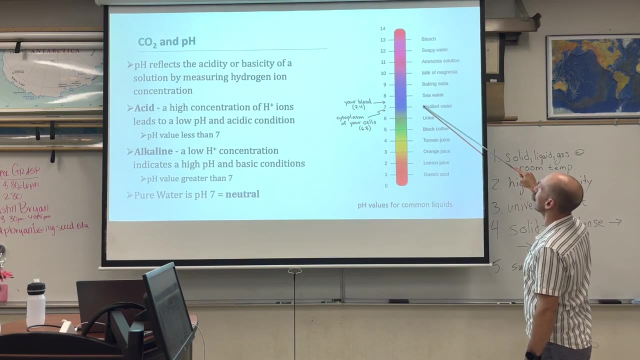 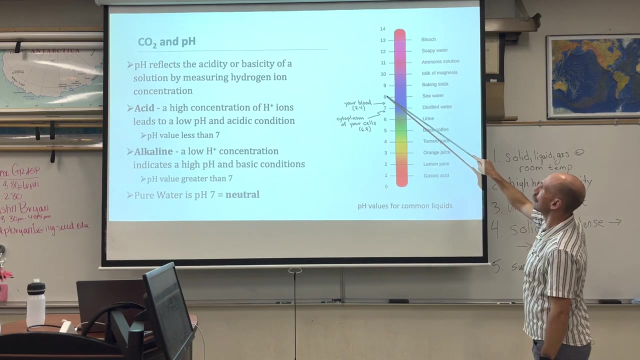 If it is above seven it is alkaline. There are hydrogen ions in all liquids. Distilled water has a neutral hydrogen ion concentration. Our blood is slightly alkaline at 7.4.. Seawater is roughly 8.1.. 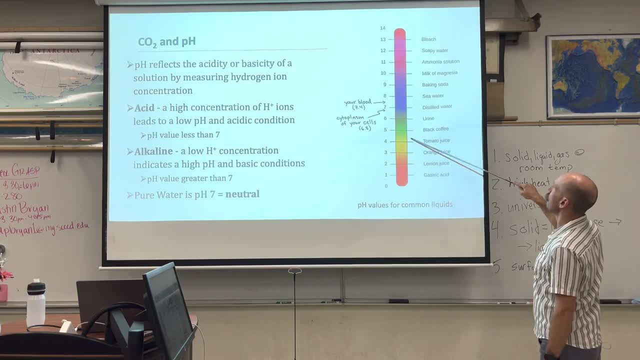 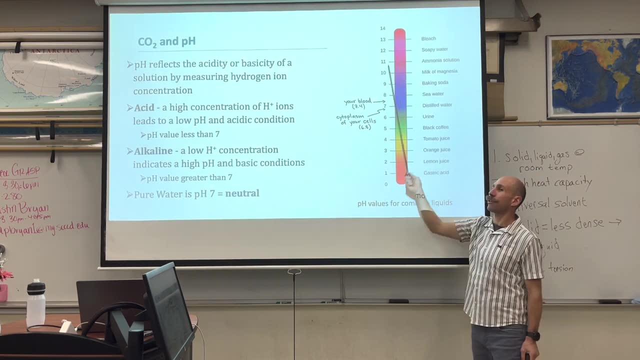 Acidic things. we know about lemons, oranges, tomatoes, coffee, alkaline cleaning solutions, bleach, soap, ammonia, And so the variation right is hydroxide versus hydrogen ions in solution. measuring those, Okay, so who? how did we get on pH? 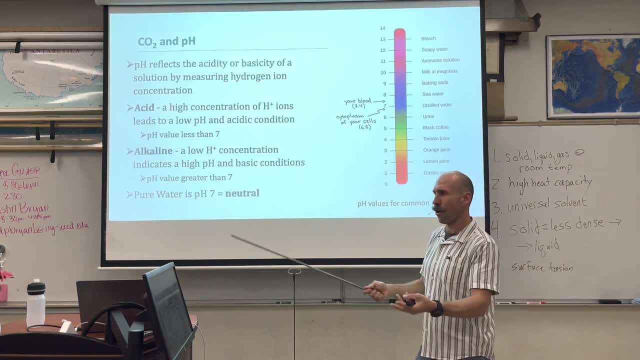 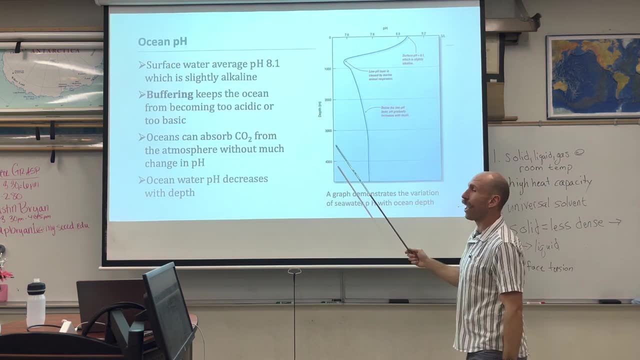 What did we get on pH? What did we get on pH? What the heck is going on here? Why is this even important? Well, the oceans have a pH, and the pH has to do with the amount of carbon that's being deposited in the oceans. 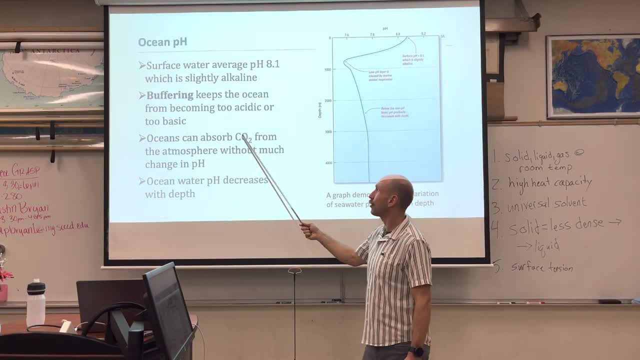 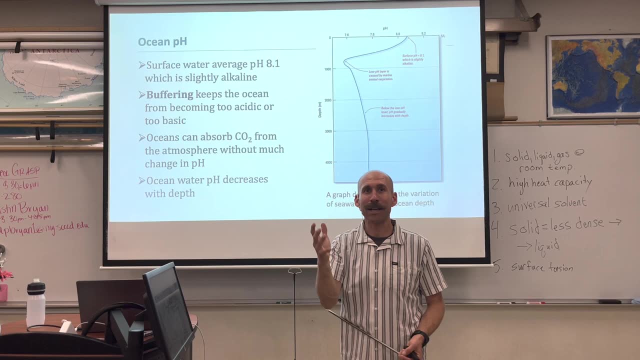 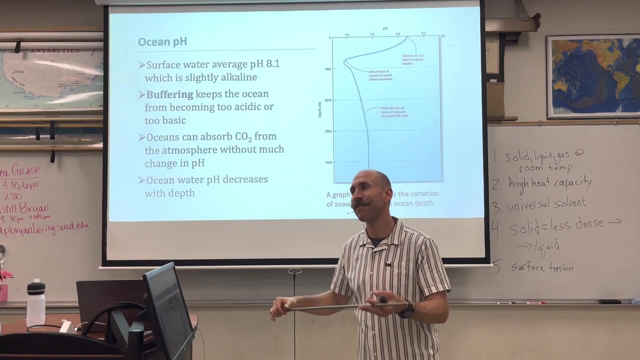 Now, whatever is happening with the carbon in the oceans is buffered, keeping the oceans from becoming too acidic or too basic. This regulates, it creates a stable environment in the Earth's oceans, And that stability is necessary for life to exist. It is the stability of temperature and salinity and pH. 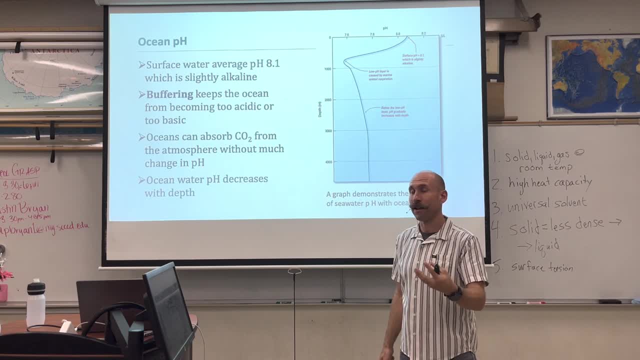 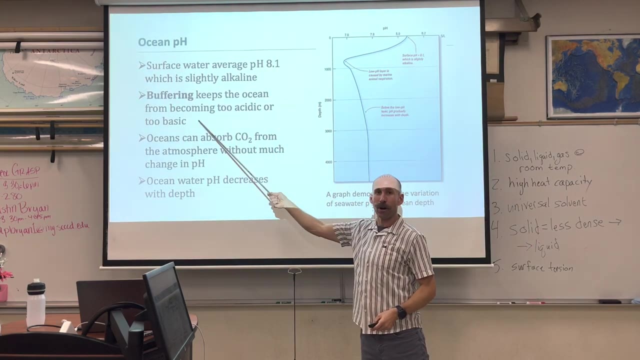 that created a hospitable environment for life to begin and also for life to evolve into the beautiful diversity, the biodiversity, which we have today. So oceans buffer carbon from becoming too acidic or basic. So oceans buffer carbon from becoming too acidic or basic. 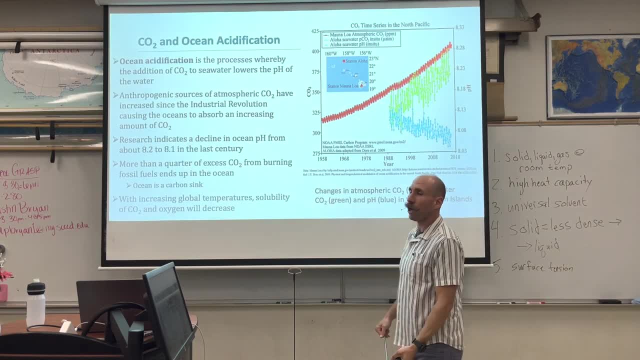 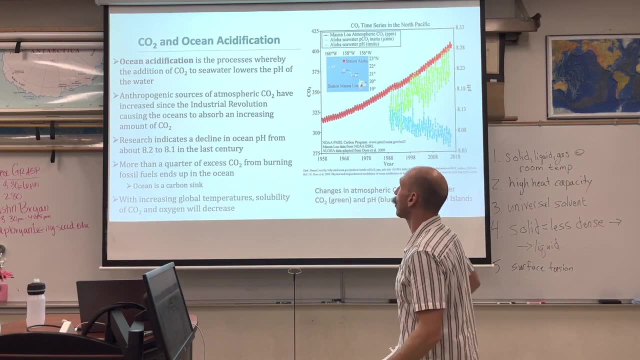 So oceans buffer carbon from becoming too acidic or basic. But fast forward to today and we'll talk a lot about this. but we cannot talk about chemical oceanography without the discussion of ocean acidification, which is the addition of CO2, lowering the pH of water. 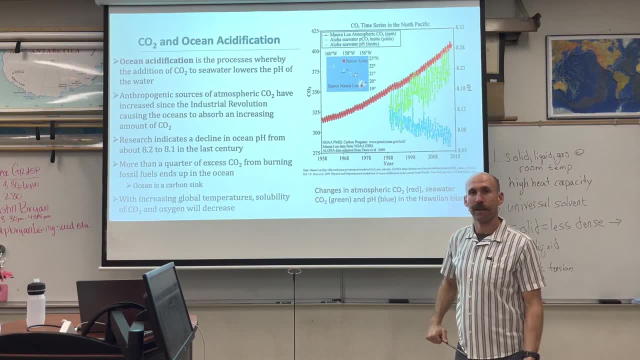 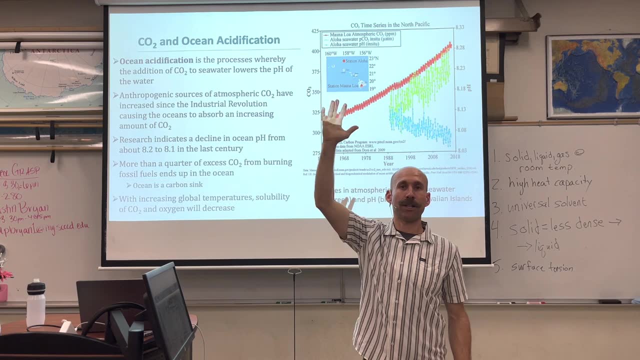 This red line is the Keeling curve. There is a site on top of Mauna Loa in Hawaii that measures atmospheric concentration. It's been doing this since 1955. It's been doing this since 1955. It's been doing this since 1955.. 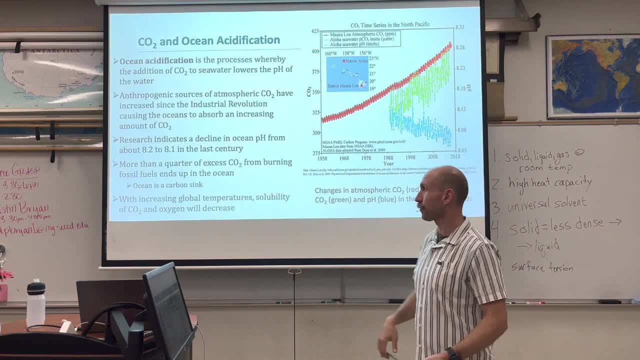 And it's been doing this since the 1950s, And it's been doing this since the 1950s And it's been doing this since the 1950s. Those measurements- direct measurements- show an increase and it varies by winter and summer. 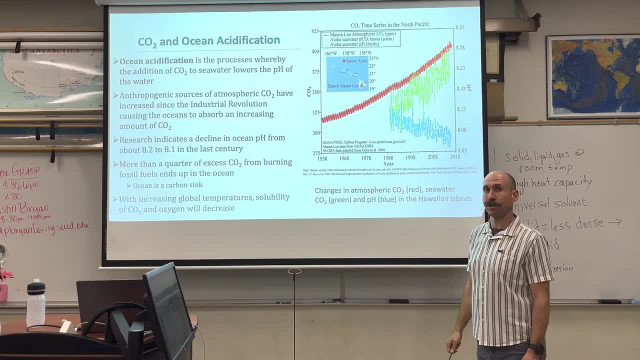 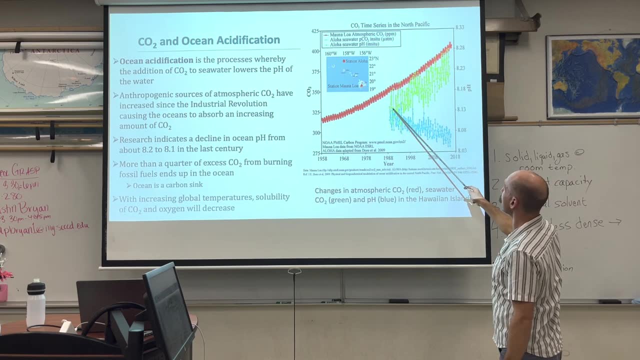 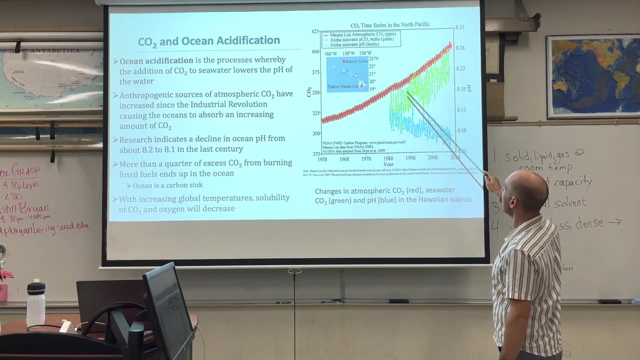 an increase of atmospheric CO2.. Also, with an increase of atmospheric CO2, there's an increase of oceanic carbon. With that increase of oceanic carbon dioxide, there's an observable decrease in ocean pH levels. There's an observable decrease in ocean pH levels. 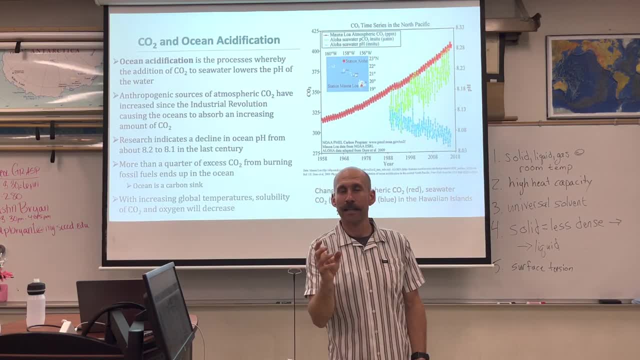 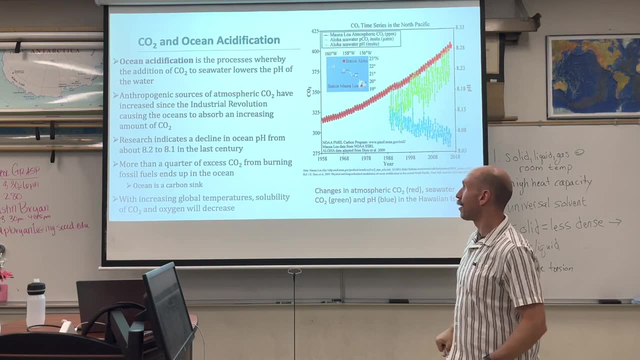 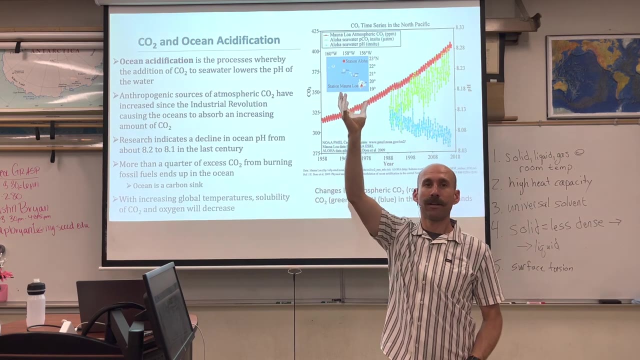 So it's not that the oceans are acidic, It's that the pH is lowering. They're becoming more acidic, They're developing towards that end because- and we'll save this conversation- but essentially the burning of fossil fuels puts more carbon dioxide into the atmosphere. 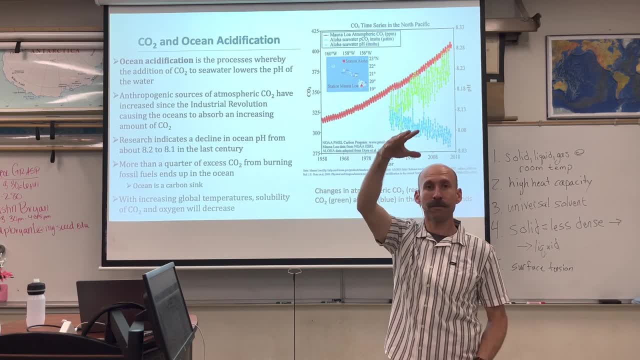 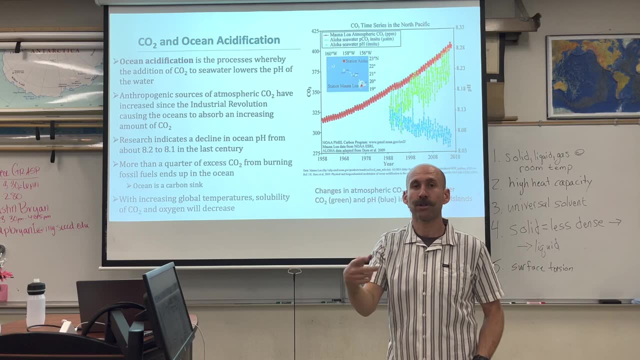 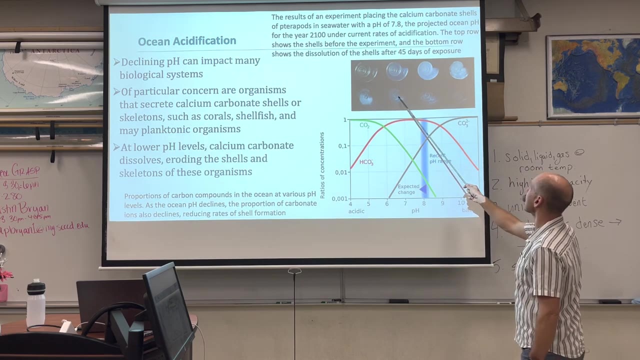 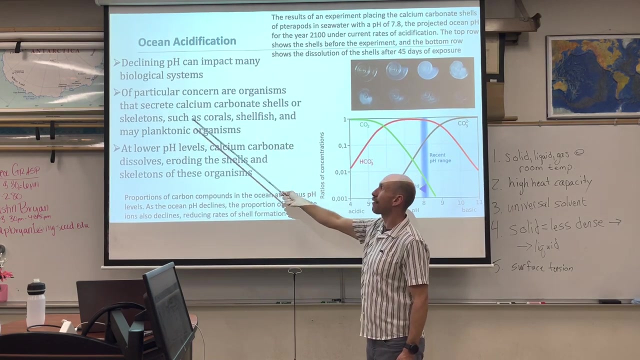 than would normally occur. More carbon in the atmosphere means more carbon in the oceans. More carbon in the oceans means more carbon dioxide, more chemical reactions creating more bicarbonate with more hydrogen ions, which in turns affects marine organisms such as corals, shellfish and marine phytoplankton. 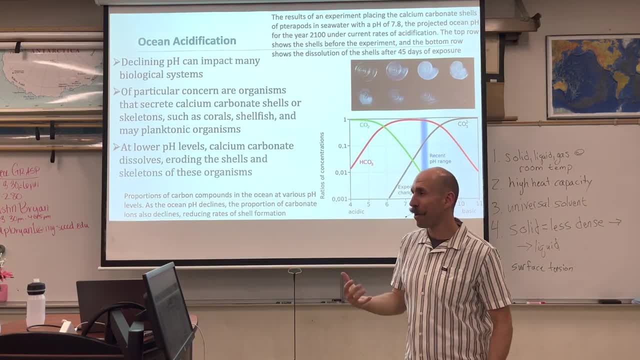 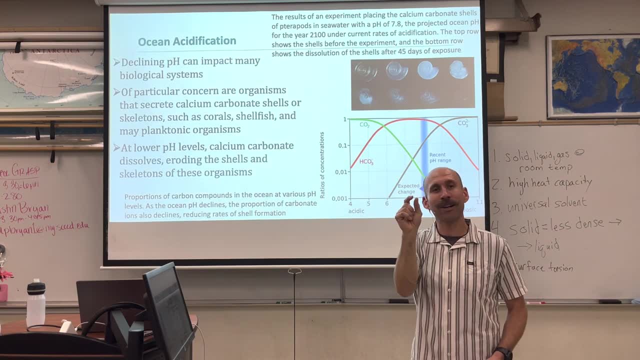 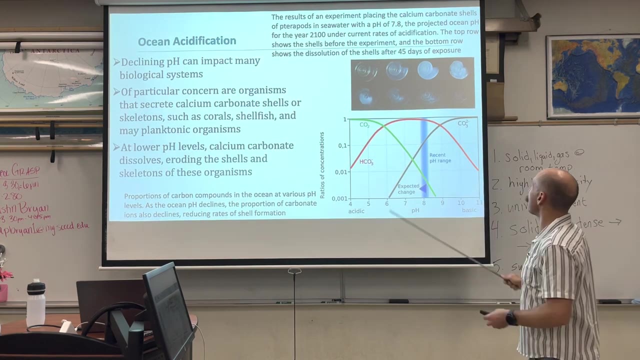 This is the base of primary productivity. The base of the food chain is the small photosynthesizing cyanobacteria and algae that are in there. They're amazing, They're microscopic. They produce calcium carbonate shells that they get from the ocean. 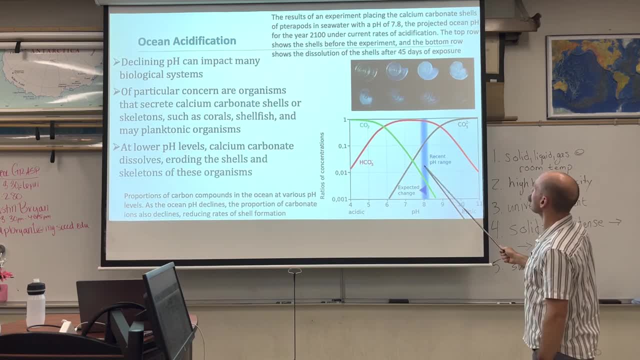 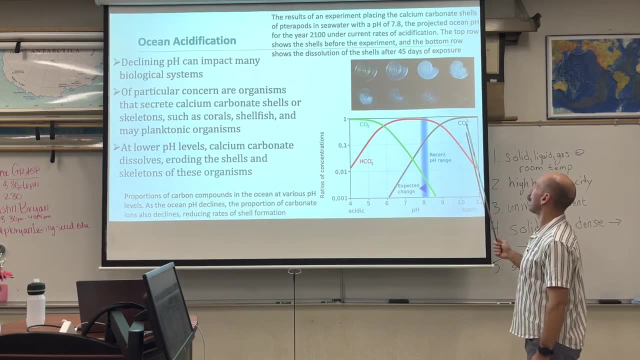 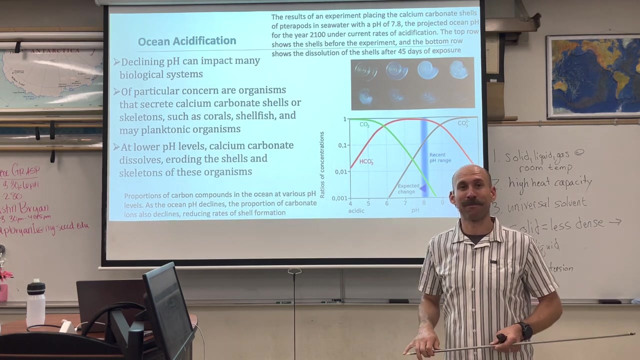 So if we have a decrease in ocean pH, right then essentially what happens is our bicarbonate and our calcium and our carbonate switch and they flip and this throws the entire system out of whack. So the short of this is: this is a big environmental problem. 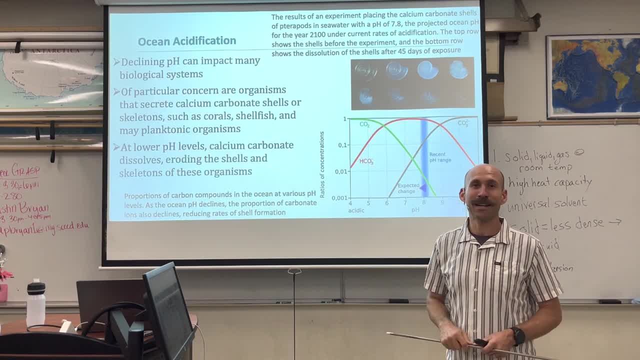 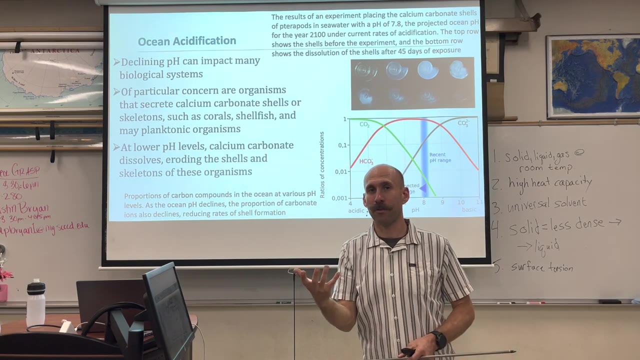 Too much carbon dioxide in the atmosphere, too much carbon dioxide in the oceans, the carbonate buffering system of the oceans starts to get thrown out of whack, affecting marine organisms, which the problem here is what happens when we cross a tipping point, which is a concept of earth system science. 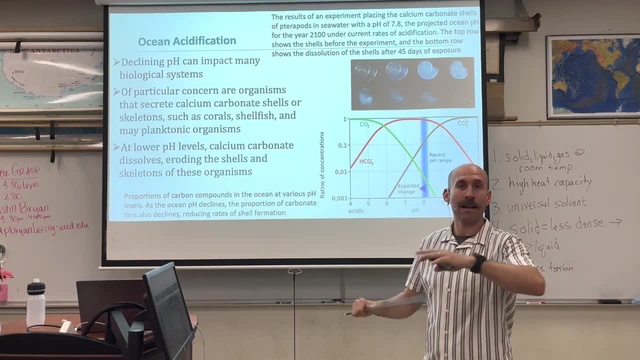 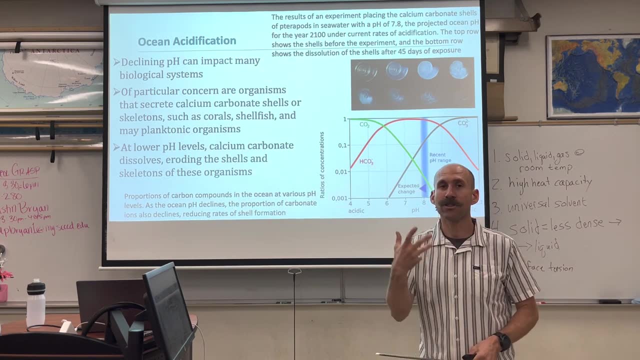 where you don't really notice the effects until it's too late, and then, oh no, what are we going to do? So if we already use the precautionary principle, then we can understand how systems work. We can make decisions now to regulate policy. 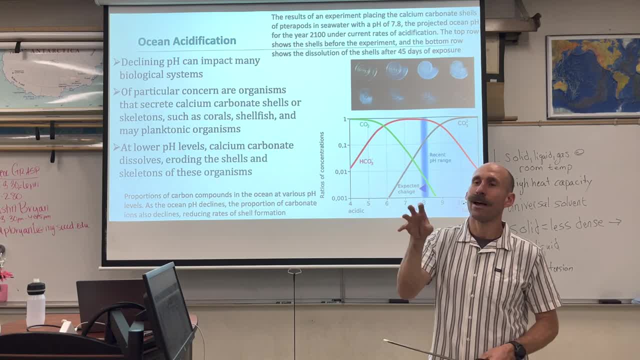 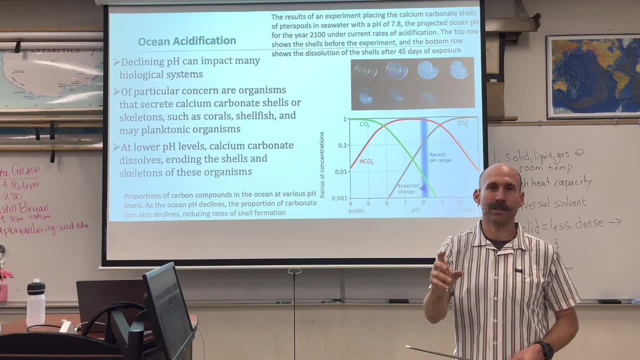 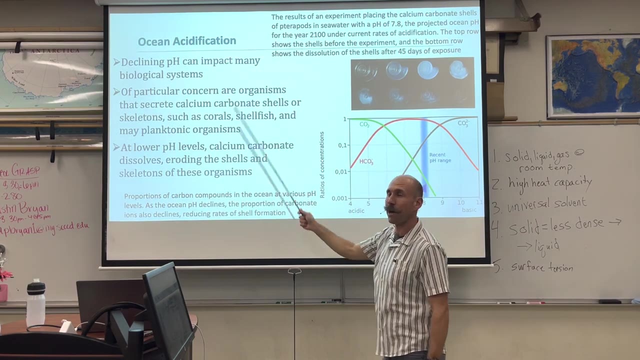 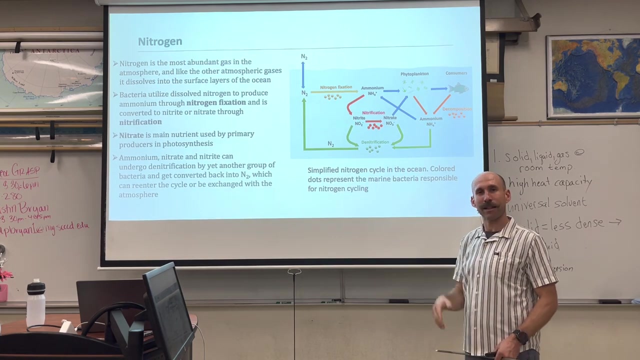 in regards to the environment, to protect marine and terrestrial ecosystems so that ocean acidification can halt the decline of biological systems. We'll talk a lot more about that, but that's kind of my little bit of a rant right there. The oceans are important. 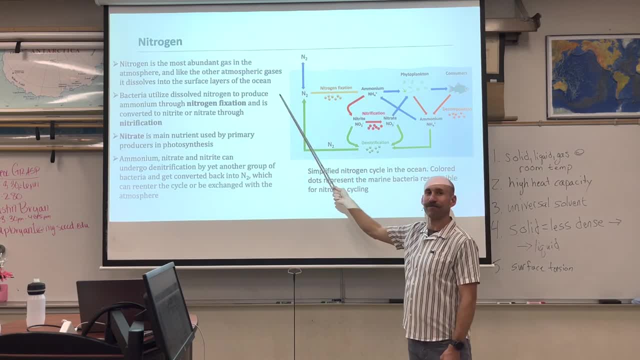 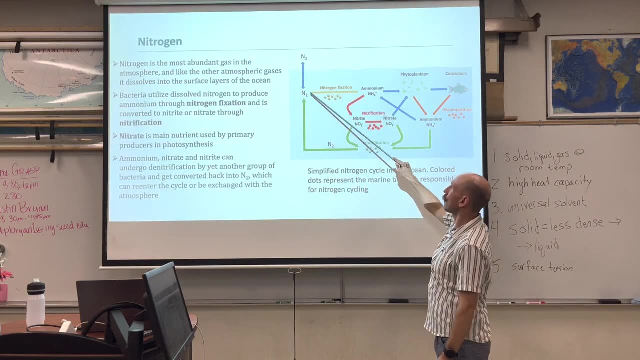 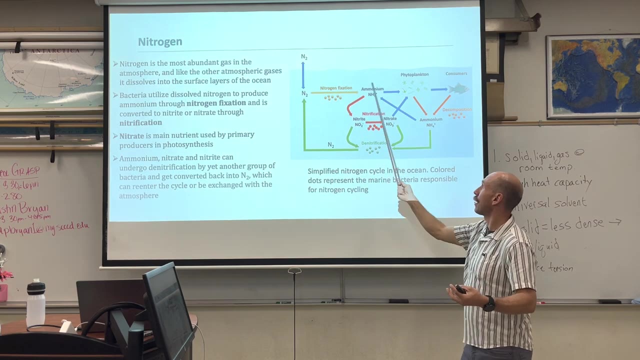 Okay, so last thing to talk about nitrogen: 78% in the atmosphere, much less in the oceans, but nitrogen from the atmosphere dissolves into the oceans and then bacteria take that into and they fix it through the process of nitrogen fixation. 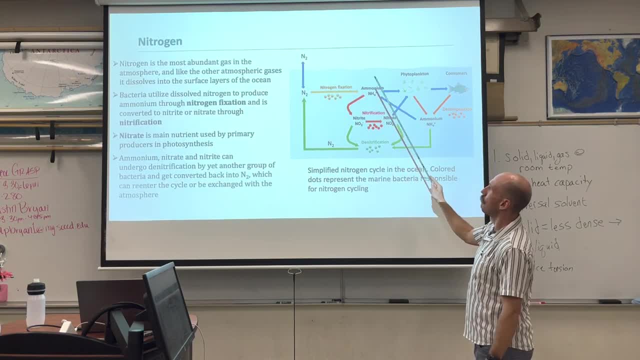 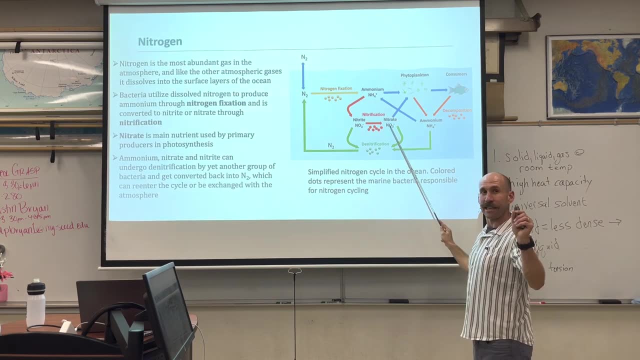 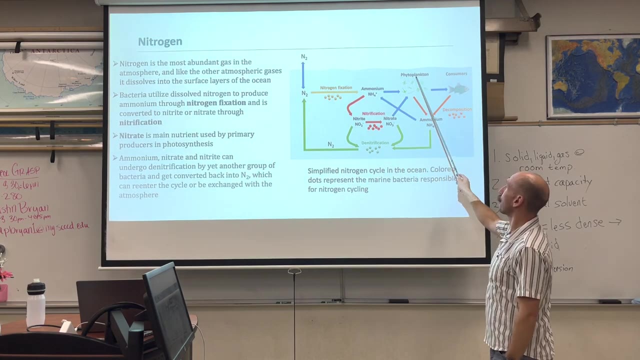 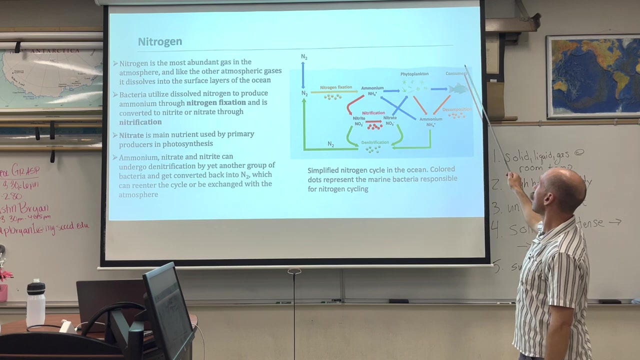 into ammonium, Now that oh, oh, oh That ammonium can be converted into nitrite and nitrate. The nitrate is the key nutrient for marine organisms, specifically for producers that need nutrients to reproduce, Producers feed consumers and, when they decompose, 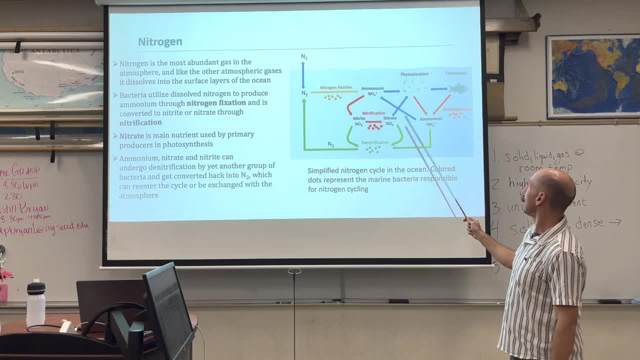 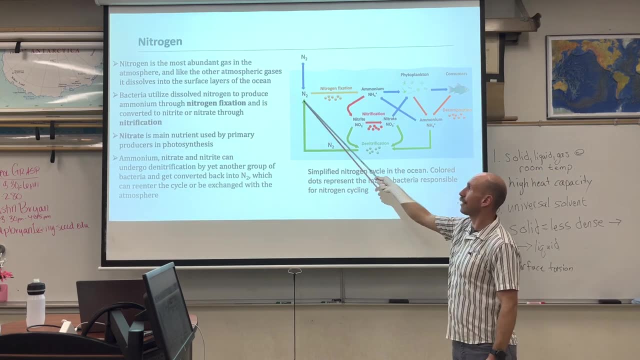 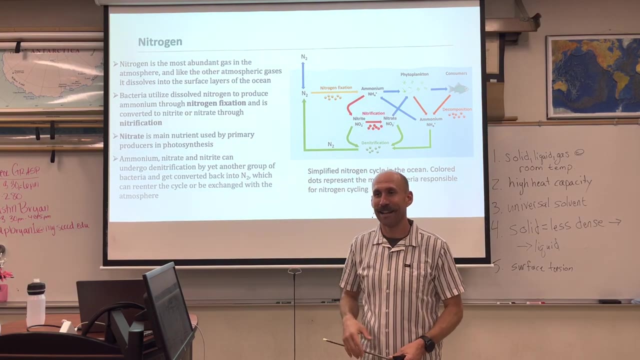 there's a process of denitrification which takes the ammonium, takes the nitrate, and then oh, oh, oh, And the nitrate that's in consumers converts it back into nitrogen again. So, wow, The oceans are so amazing that they have the ingredients. 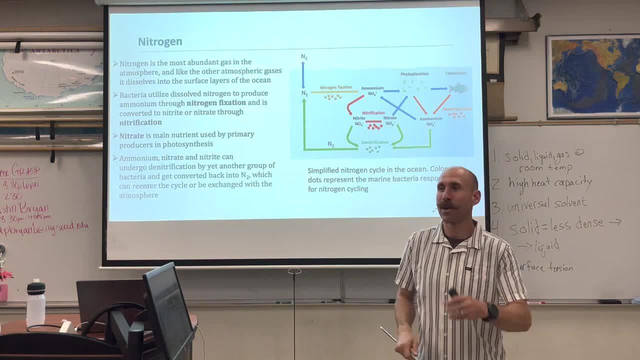 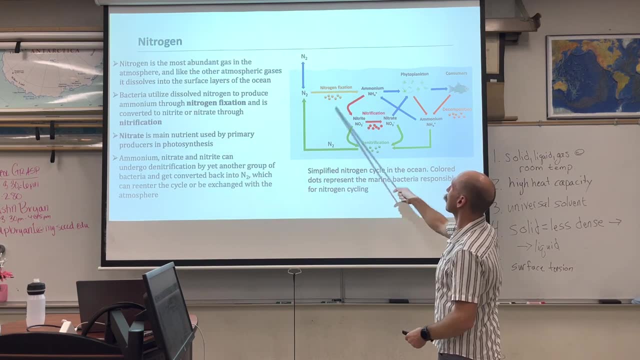 and they can switch from one form to another, from carbon dioxide to bicarbonate, from dissolved nitrogen gas into nitrate, and then cycle these nutrients back again. These are called biogeochemical cycles. These are called biogeochemical cycles. 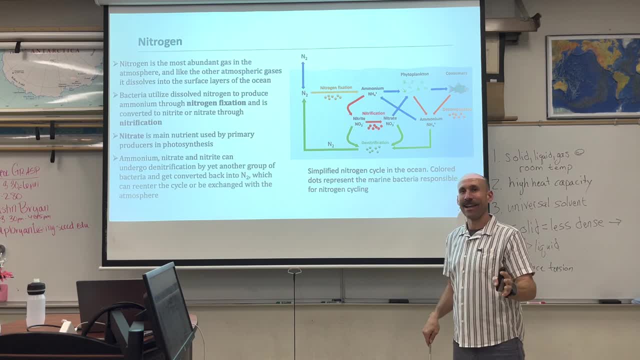 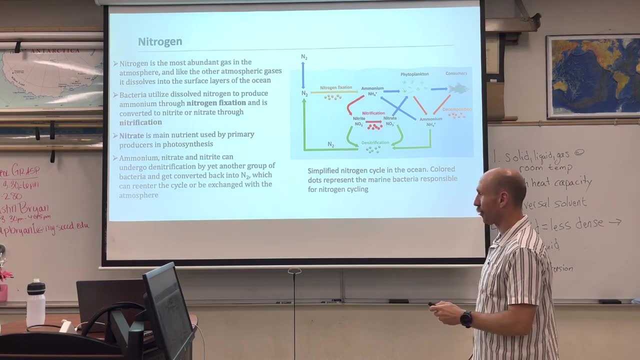 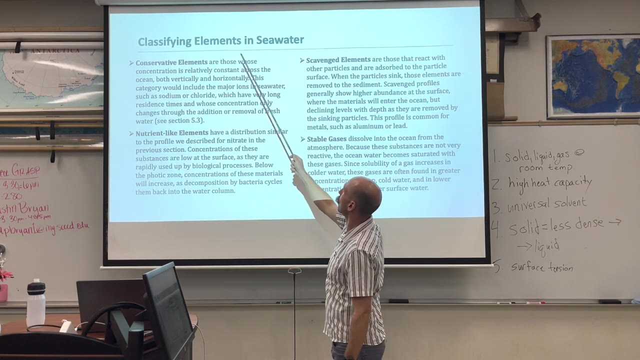 These are called biogeochemical cycles. They're fascinating in how they move elements and compounds and nutrients around the earth. So this gives us different types of elements. in seawater We've got conservative elements, the ones whose concentration is relatively constant. 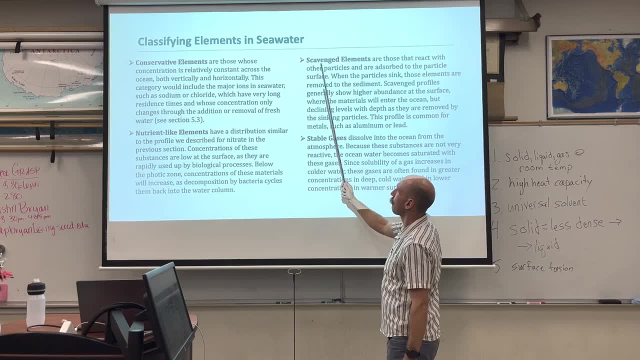 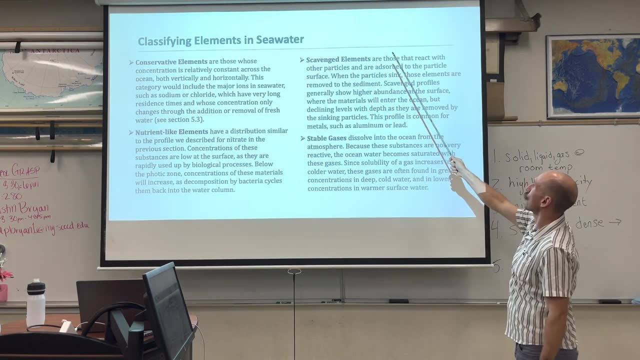 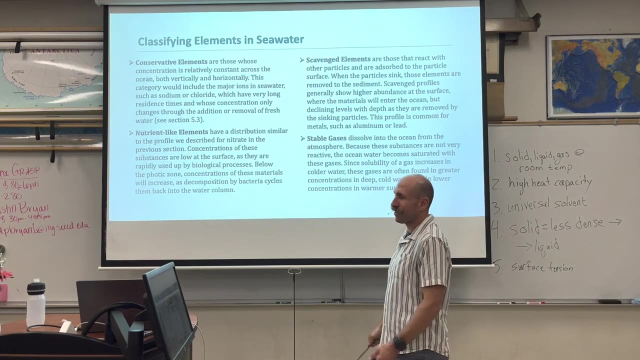 nutrient-like elements where the distribution is very similar to nitrates. They're nutrients Scavenged, are those that react with other particles, that are absorbed to the particle's surface and then dissolve stable gases from the atmosphere. And this is kind of the variability of elements. 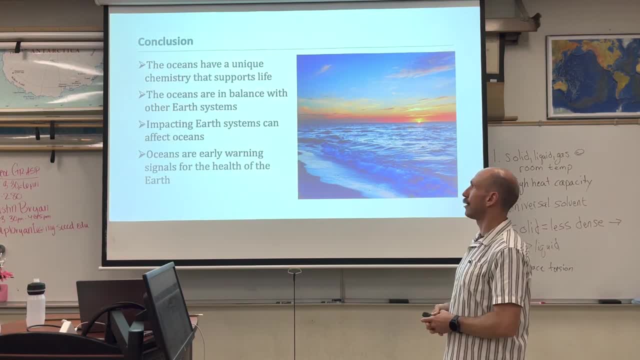 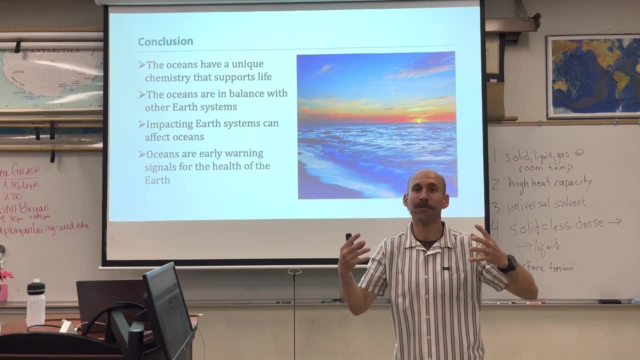 that we have in seawater. So do-da, da-da-da. that was a lot of information and I really appreciate your attention and I hope that you could absorb this. If it was too much content, watch the video again. That's why it's here for you. 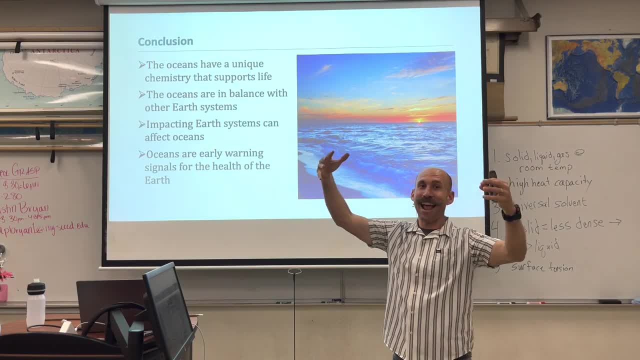 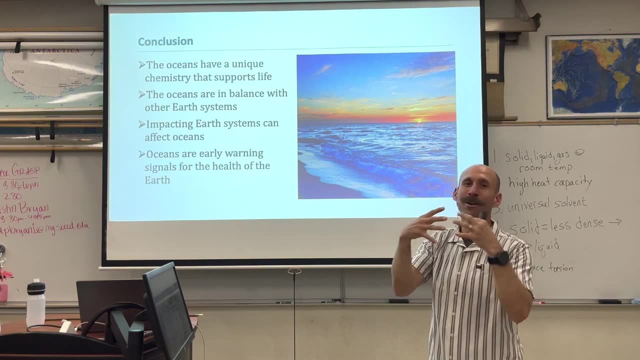 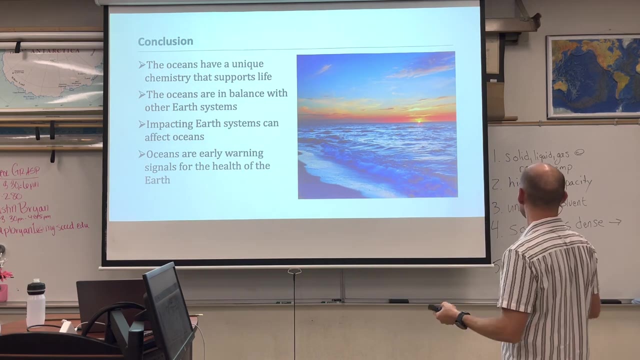 But, in summary, these are the things that we have room for. The oceans are amazing and they have a very unique chemistry that supports life, and a lot of it has to do with the water molecule and its very distinct shape and its unique properties that allow for solid liquid gas at room temperature. 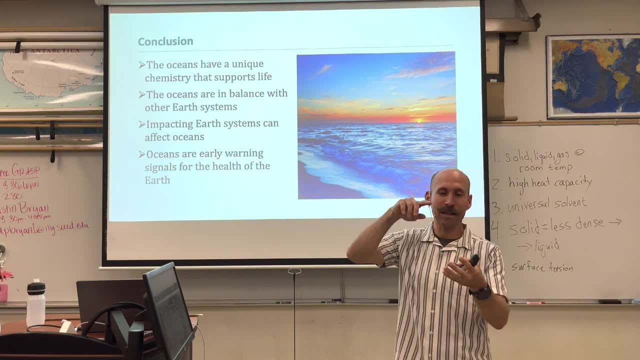 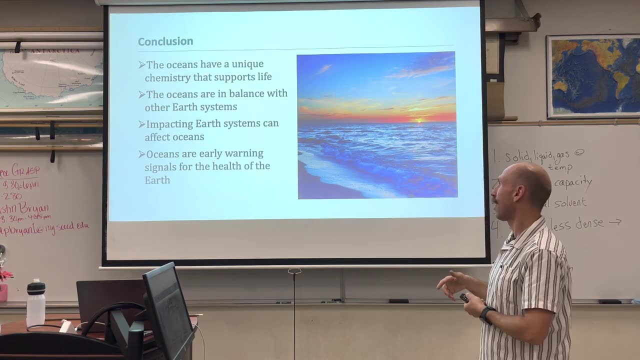 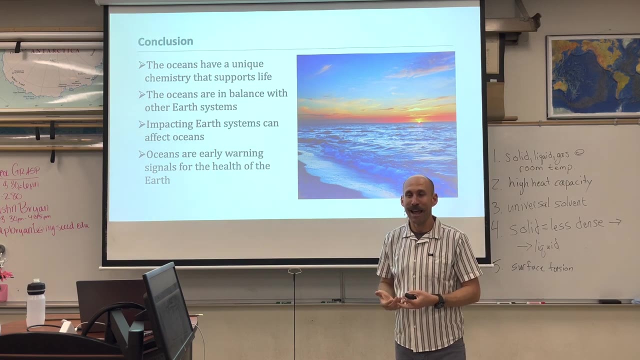 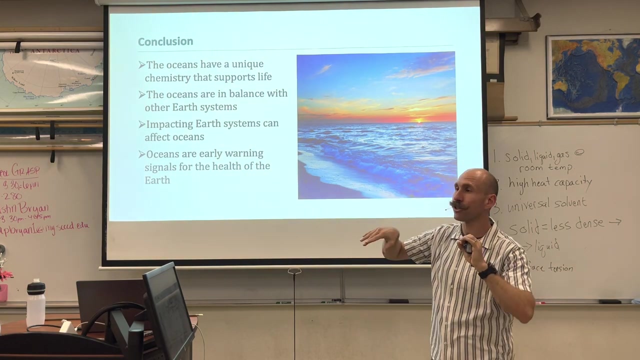 high heat capacity. being a universal solvent, less dense solid than it is liquid, and being such an extreme surface tension substance, The oceans are in balance with other Earth systems. and if the oceans are thrown out of balance because of other impacts, anthropomorphic especially,